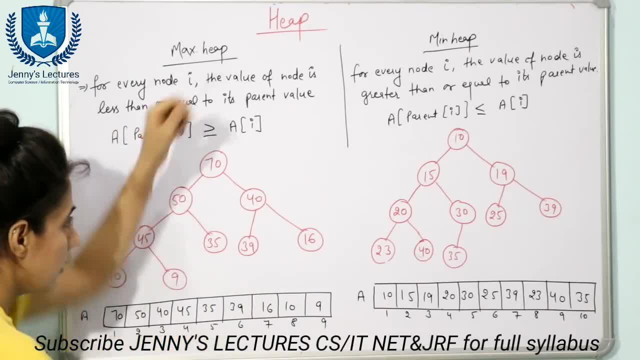 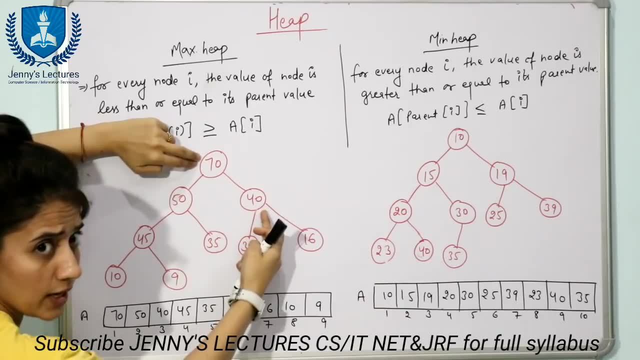 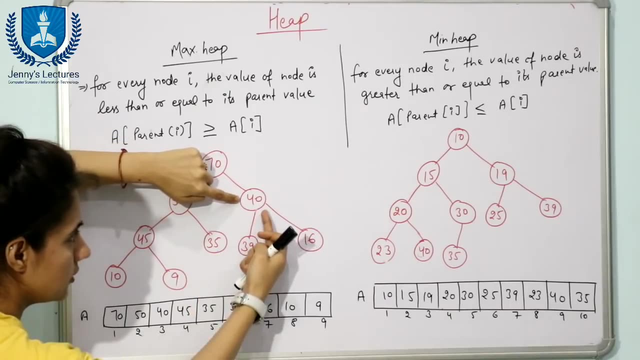 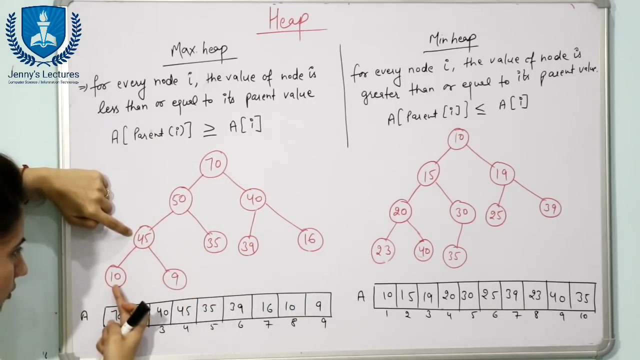 here see, let us analyze this tree. Here you can see this: the 70.. 70 is greater than 50 and 40. Yes, means parent is greater than its child node. This 50 is also greater than then its child node 45 and 35. This 40 is greater than 39 and 16, both greater than its child nodes. 45 is also greater than its child node, that is, 10 and 9.. So here what you can say is here the parent. 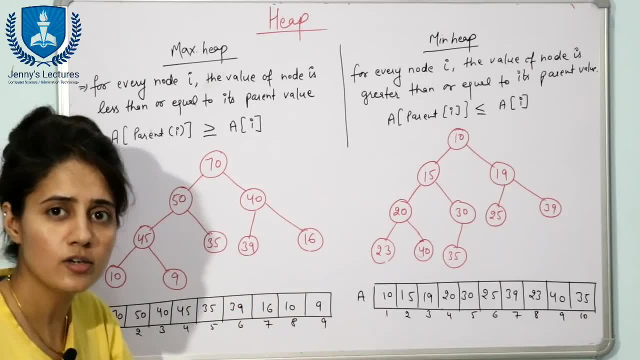 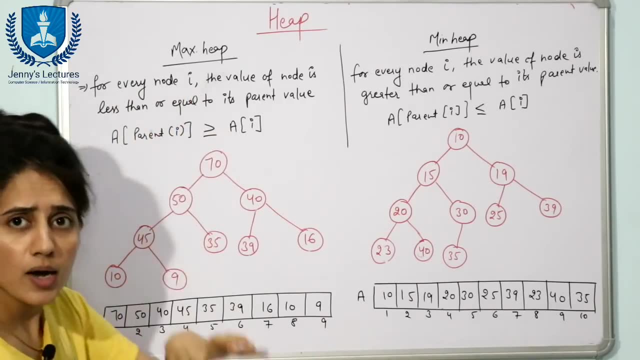 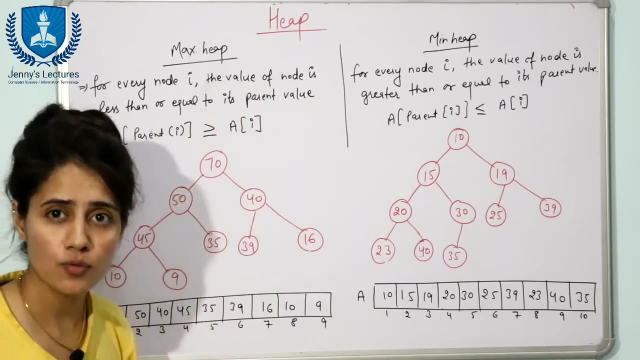 each parent node is greater than its child node, fine. so max heap is what in max heap you can say for every node i the value of the node is. value of the node is either less than or equal to its parent value, fine. or you can write like this: except root node. here you are writing: 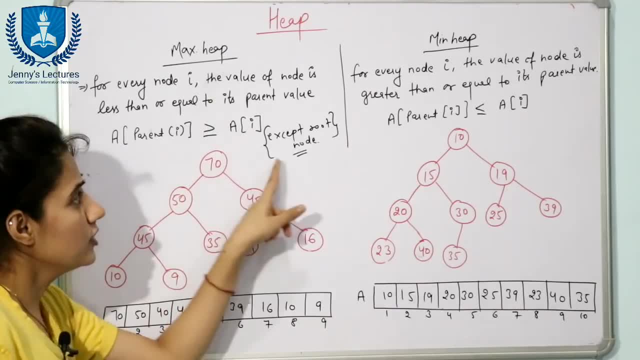 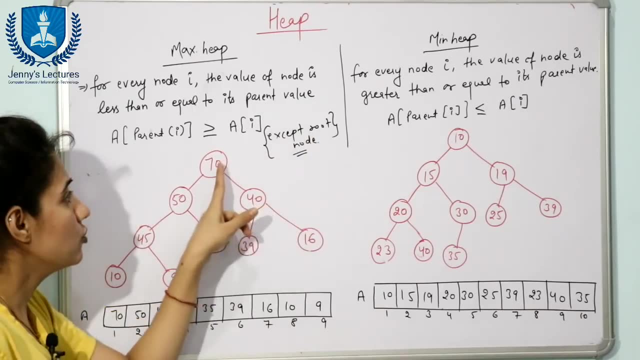 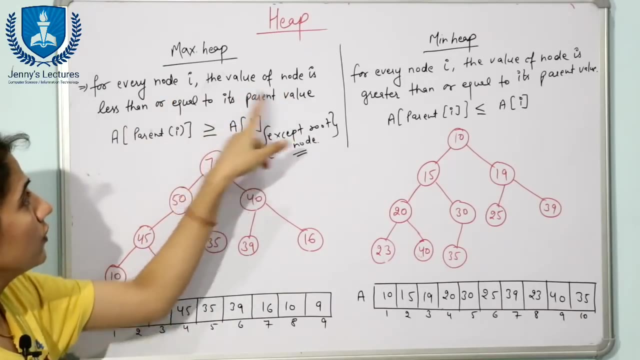 say this condition is not true for root node. this condition is true for every node except root node. why so? because root node is not having any parent. fine, and here i am saying that the value of the node is less than or equal to its parent value, but it is not having any parent. 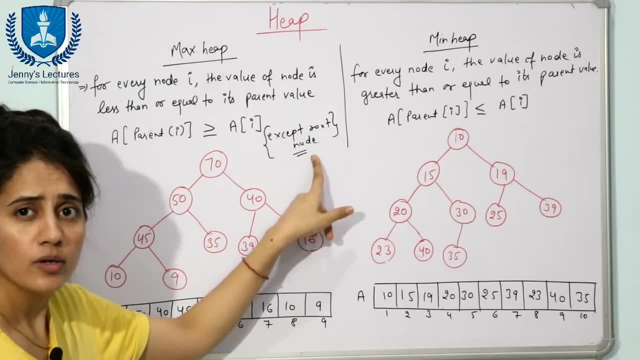 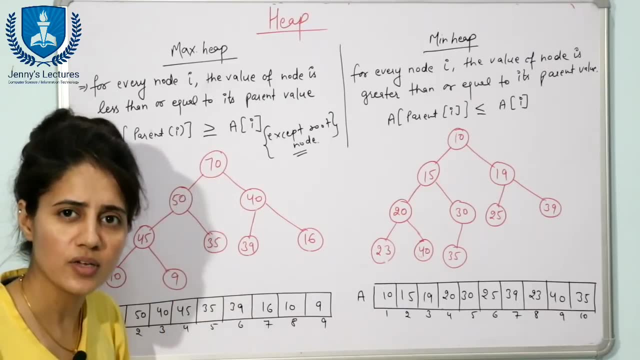 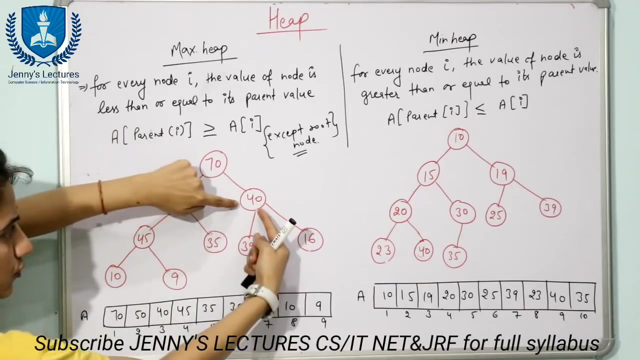 value. so that is why this condition is not true for root node. fine, or in simple word, you can say every parent, or you can say every node is having value greater than or equal to all its descendant values. fine, see this: 70 is greater than to all its descendant values. you can check this. 40 is 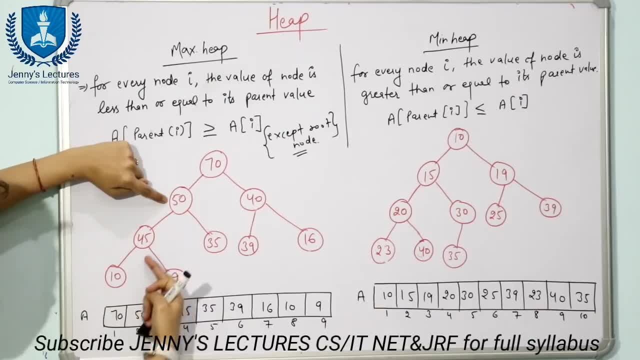 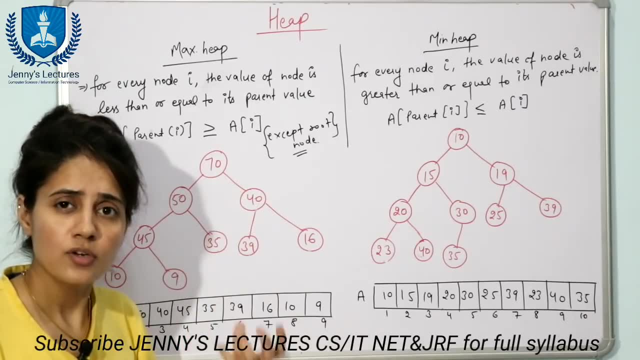 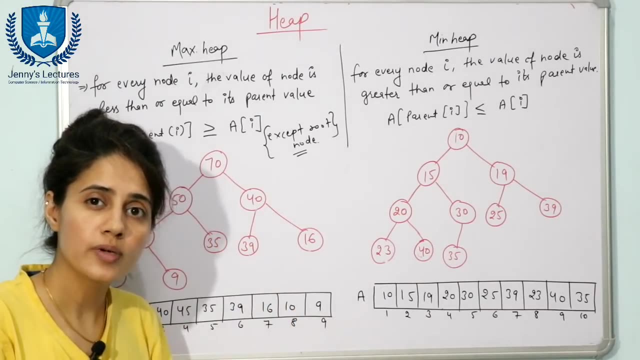 also greater than its descendant value. this 50 is also greater than to all its descendant values. fine, or you can say: for every node i, for every node i, the value of that node would be either greater than or equal to its child node. okay, and that condition is true for all the nodes. 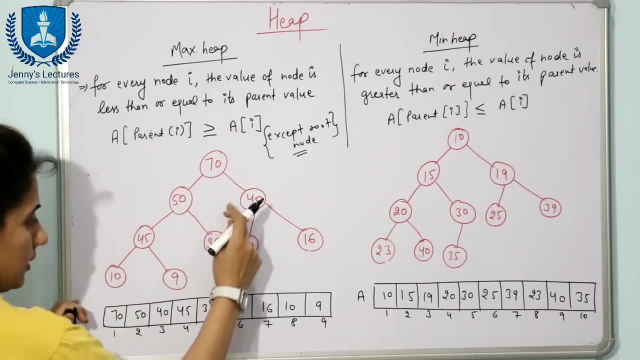 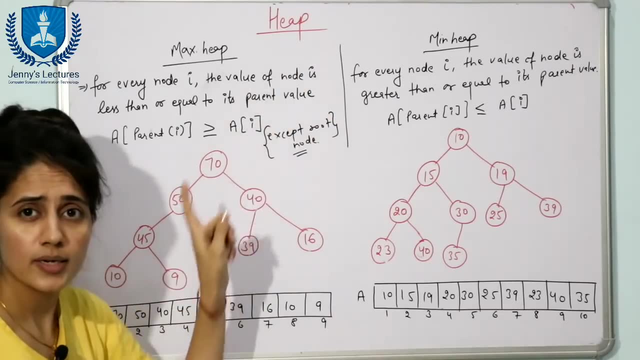 so here, if you are taking, i value see, this is the binary, this is the array, representation of this binary tree. this is first condition, for heap is what it is: a complete binary tree, or you can see, it is a almost complete binary tree. this is a complete, almost complete binary tree. 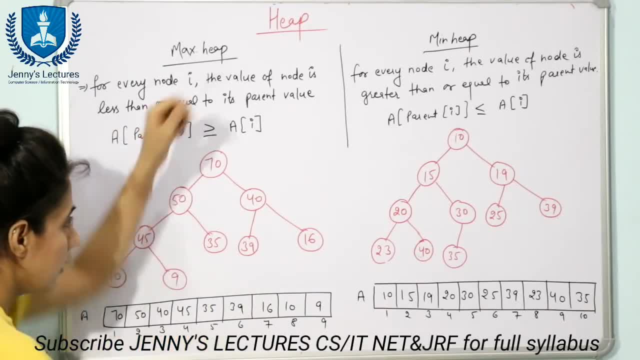 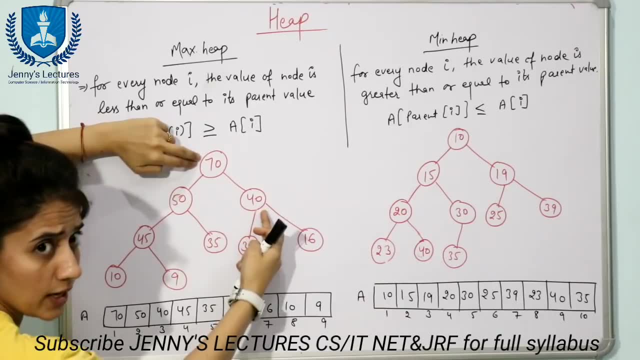 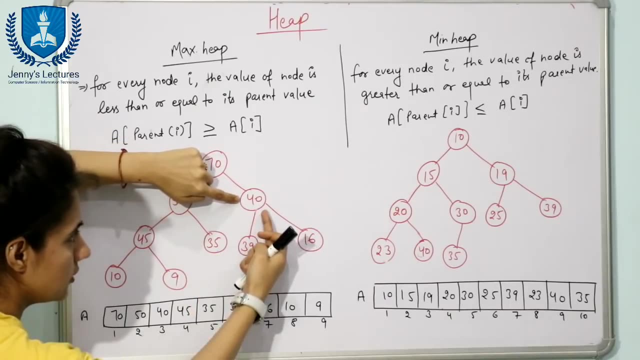 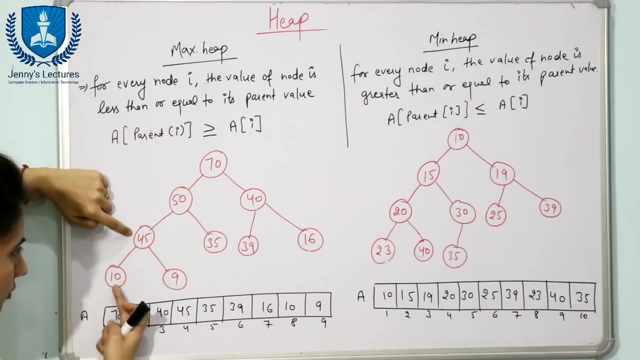 here see, let us analyze this tree. Here you can see this: the 70.. 70 is greater than 50 and 40. Yes, means parent is greater than its child node. This 50 is also greater than then its child node 45 and 35. This 40 is greater than 39 and 16, both greater than its child nodes. 45 is also greater than its child node, that is, 10 and 9.. So here what you can say is here the parent node. 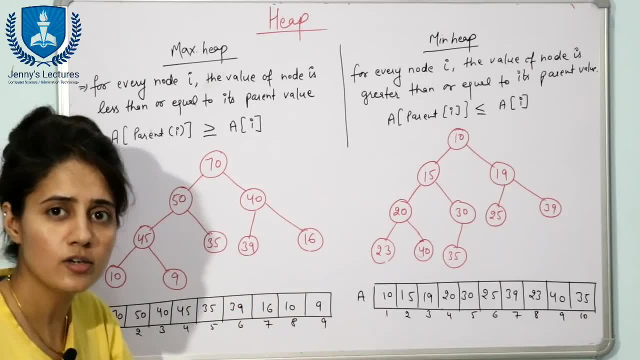 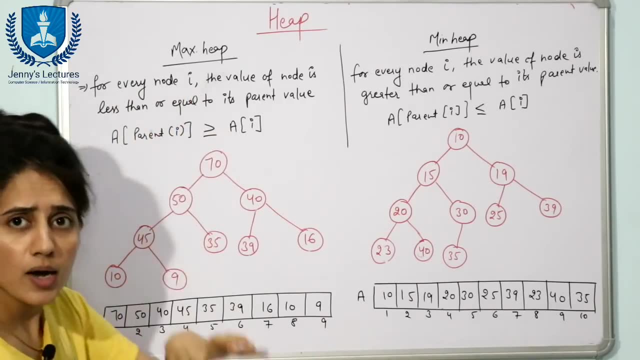 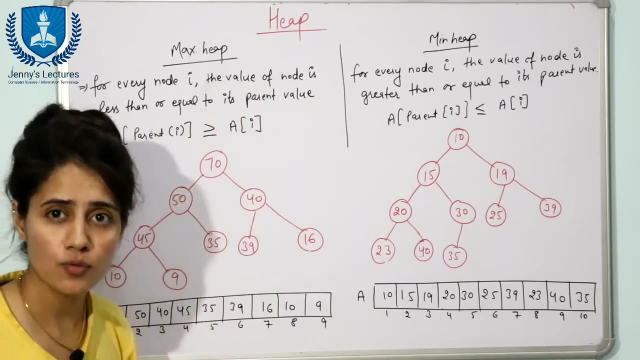 each parent node is greater than its child node, fine. so max heap is what in max heap you can say for every node i the value of the node is. value of the node is either less than or equal to its parent value, fine. or you can write like this: except root node. here you are writing: 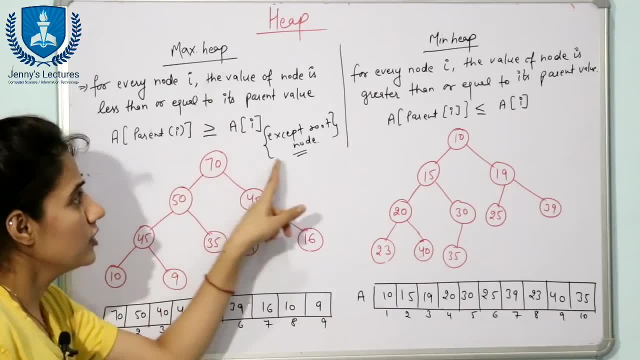 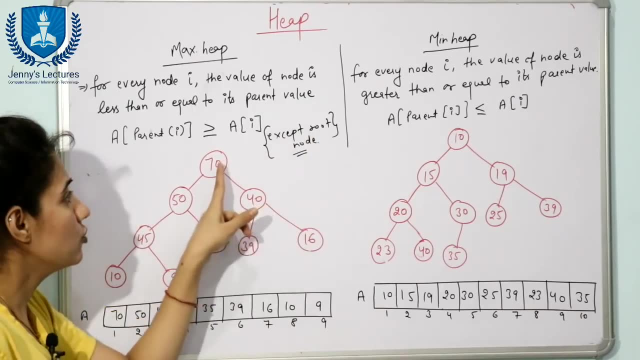 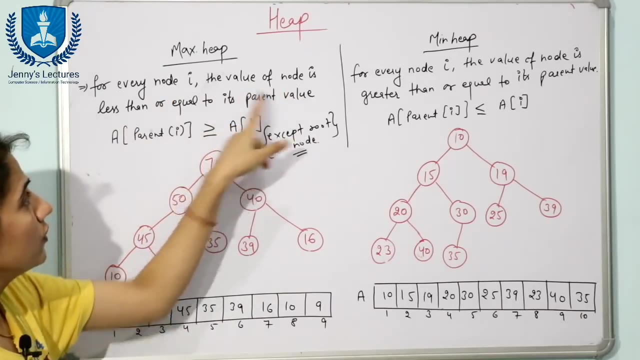 say this condition is not true for root node. this condition is true for every node except root node. why so? because root node is not having any parent. fine, and here i am saying that the value of the node is less than or equal to its parent value, but it is not having any parent. 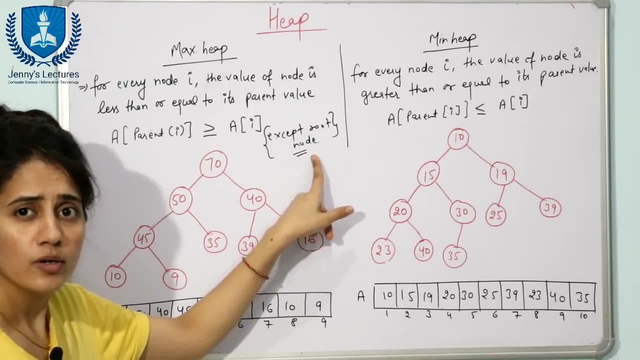 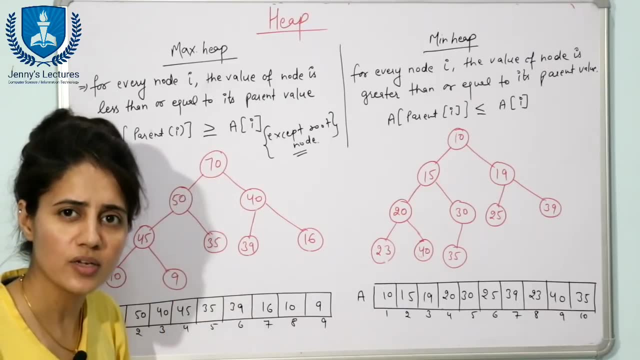 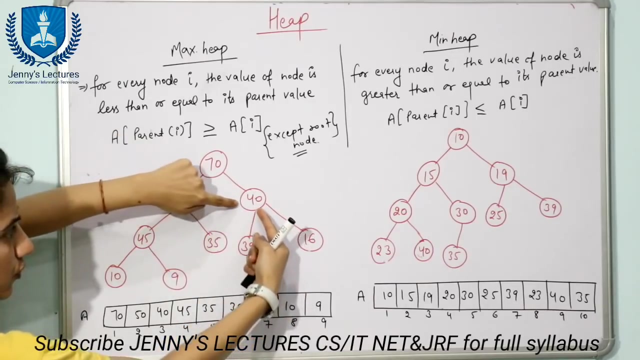 value. so that is why this condition is not true for root node. fine, or in simple word, you can say to every parent, or you can say: every node is having value greater than or equal to all its descendant values. fine, see this: 70 is greater than to all its descendant values. you can check this. 40 is 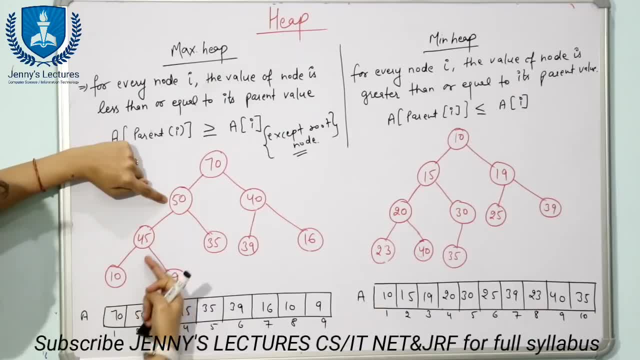 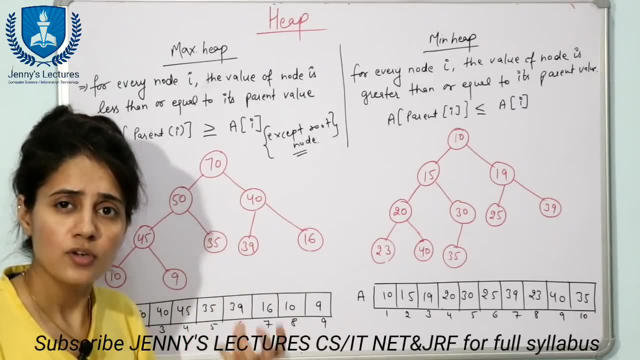 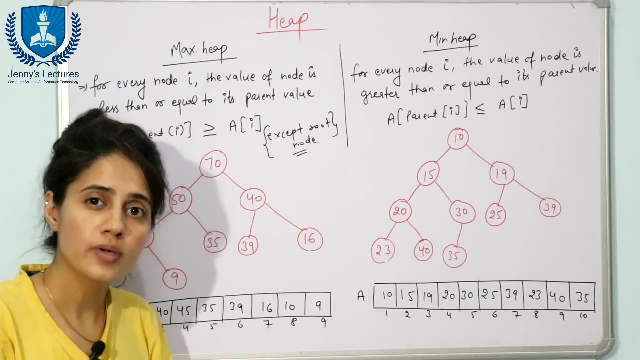 also greater than its descendant value. this 50 is also greater than to all its descendant values. fine, or you can say: for every node i, for every node i, the value of that node would be either greater than or equal to its child node. okay, and that condition is true for all the nodes. 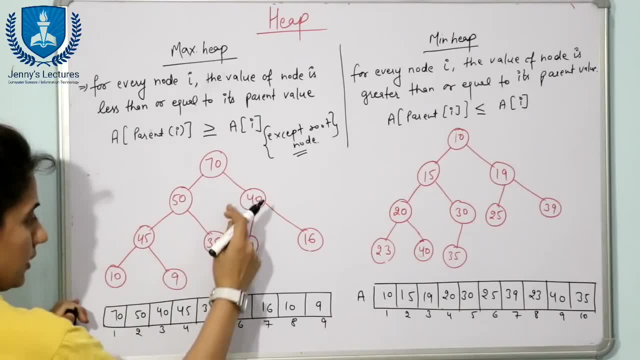 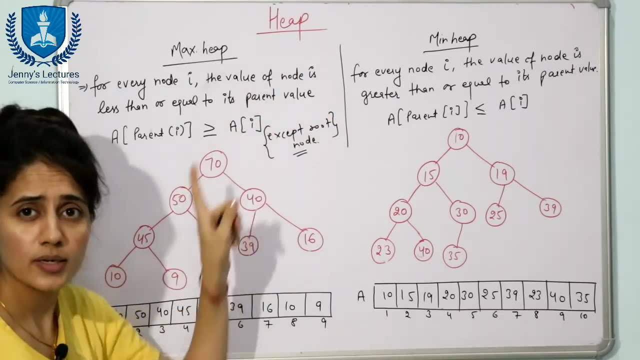 so here, if you are taking, i value see, this is the binary, this is the array, representation of this binary tree. this is first condition, for heap is what it is: a complete binary tree, or you can see, it is a almost complete binary tree. this is a complete, almost complete binary tree. 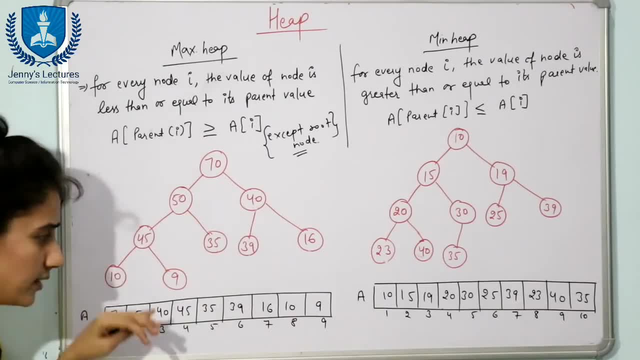 yes, all the levels except the last level are completely filled and the elements in the last level are as left as possible. fine, so here this is the array representation of this thing. i have already discussed this thing in previous video. fine, array name is a index. i am going to start. 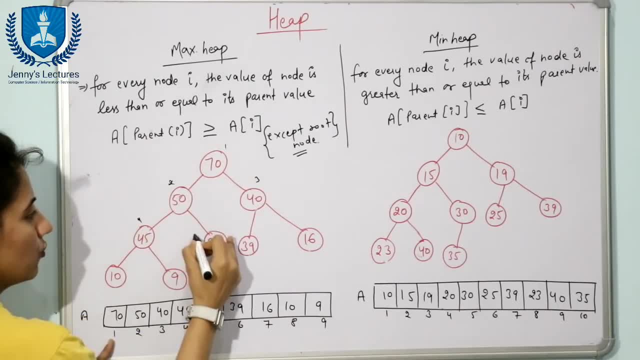 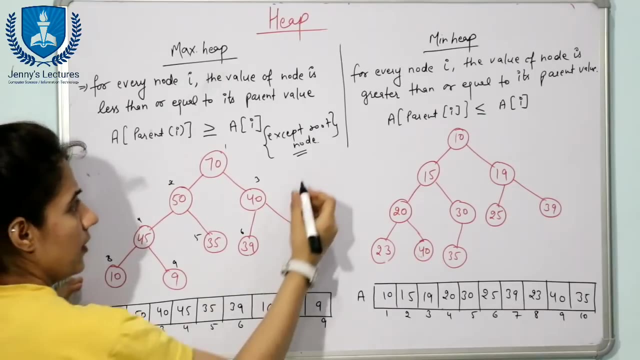 from one, so one here, two here, three here. we have four, five, six, seven, eight and nine. like this, we are going to write down this tree in a array, level by level and from left to right. fine, and see now, if you are taking, i value is equal to three for every node. i suppose i is equal to. 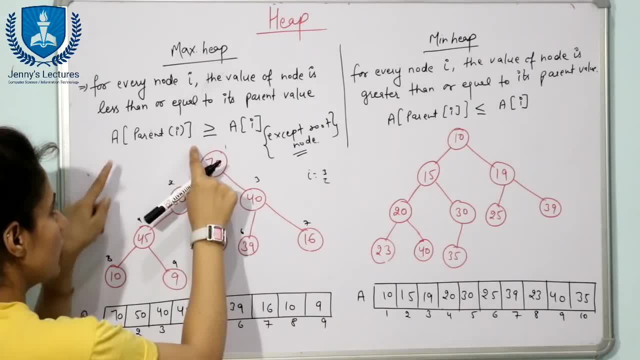 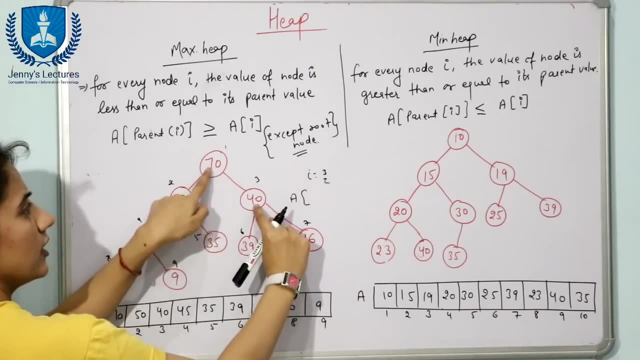 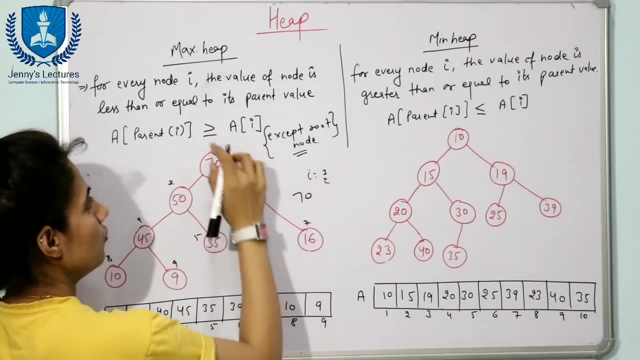 three. this condition should be held. now check a of parent of i. i mean i means three. fine now, parent of this thing is one right. so the value of a of parent of i is 70. it means you can say 70 would be greater than or equal to a of i. i value is three, a of three. 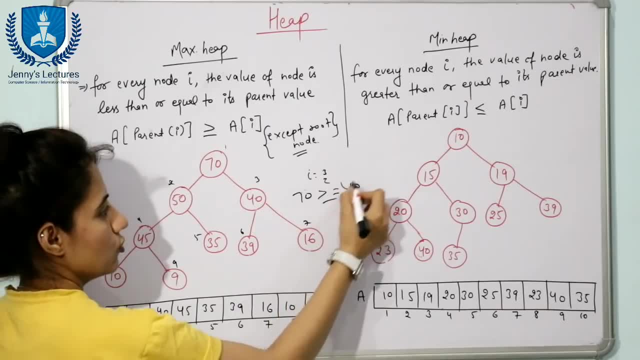 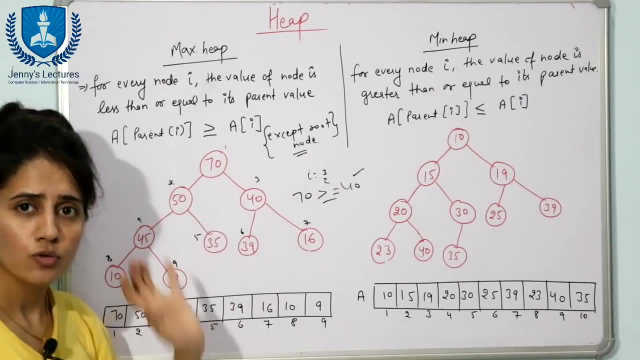 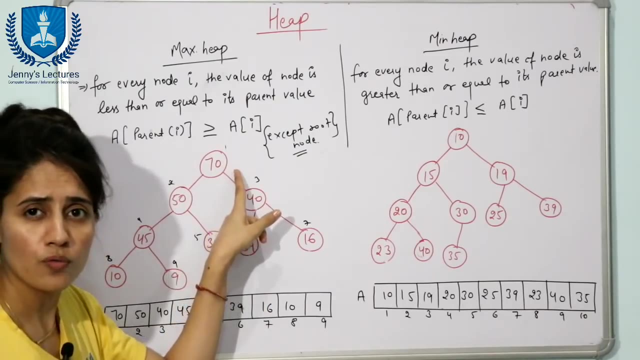 what is a of three value: 40, 40. so this condition is true. 70 is greater than 40. yes, so this condition is true for all the nodes except root node, because root node is having no parent node. so this is max heap, and in max heap the root node would always be the largest element. here you can check. 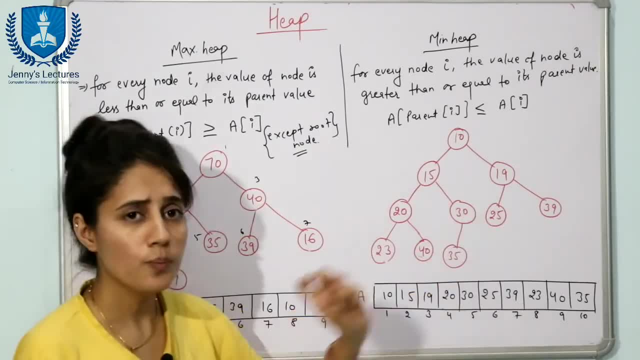 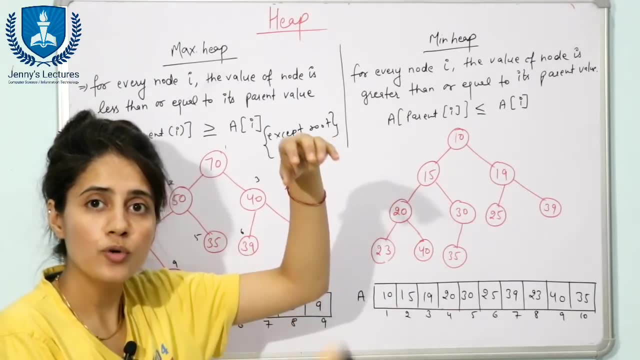 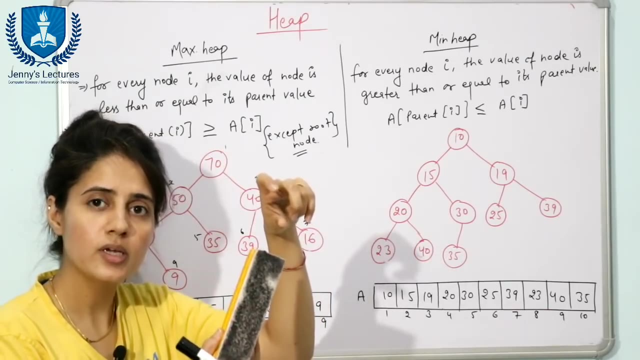 the largest element among all these. fine, now what about min heap? just opposite to this thing, parent node would be less than or equal to its child node. or you can say, for every node i, the value of that node would be less than or equal to all its descendant nodes. 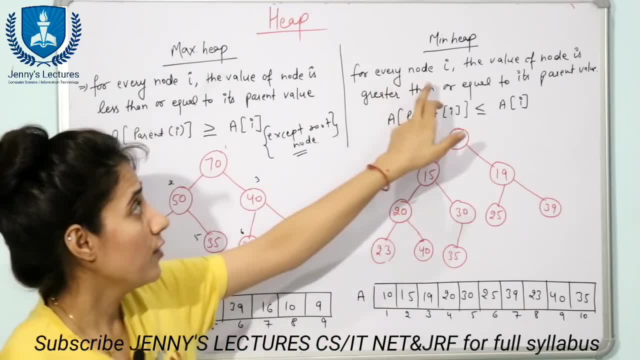 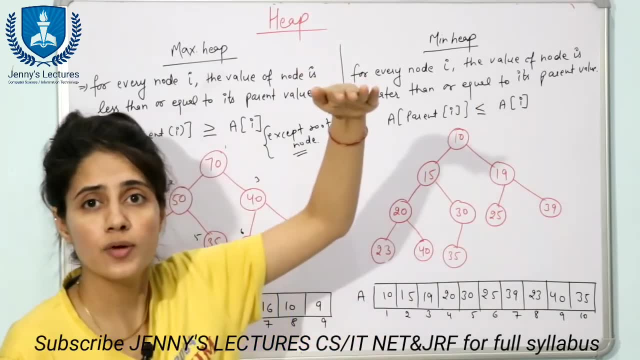 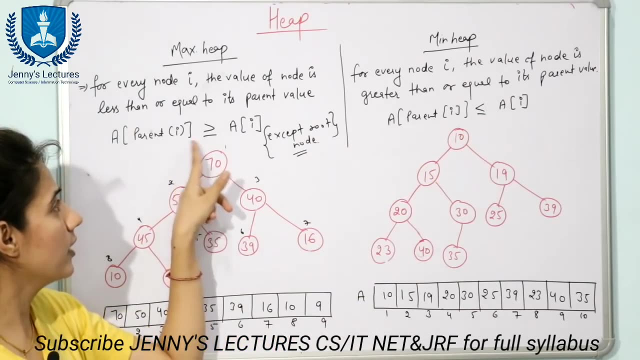 fine. or in another word, you can say: for every node i, the value of that node is greater than or equal to its parent value. fine, so this condition should be held: a of parent should be less than or equal to a of i. here a of parent i would be greater than or equal to a of i, and same this condition. 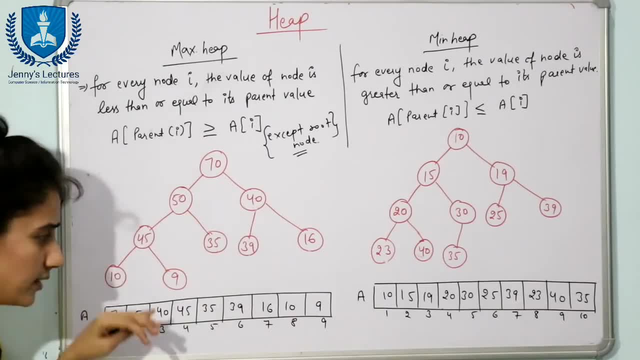 yes, all the levels except the last level are completely filled and the elements in the last level are as left as possible. fine, so here this is the array representation of this thing. i have already discussed this thing in previous video. fine, array name is a index. i am going to start. 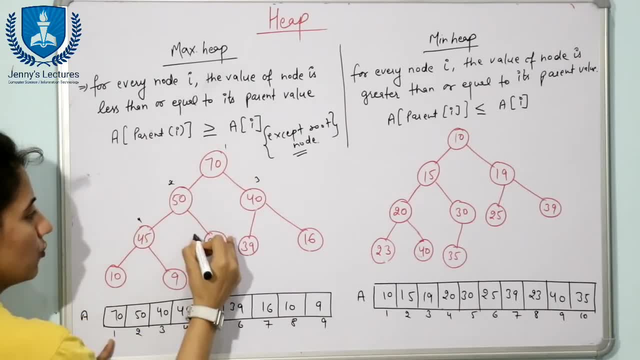 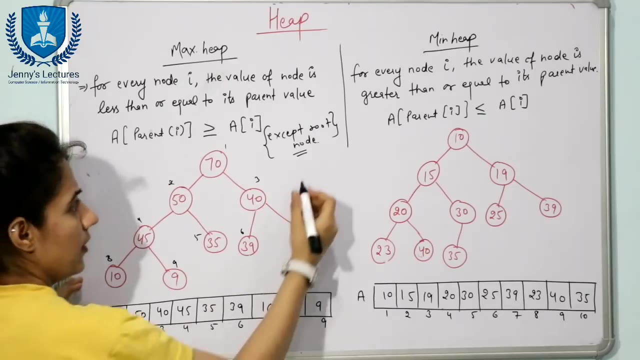 from one, so one here, two here, three here. we have four, five, six, seven, eight and nine. like this, we are going to, you are going to, you are going to write down this tree in an array, level by level and from left to right. fine, and see now, if you are taking, i value is equal to three for every node. i suppose i is. 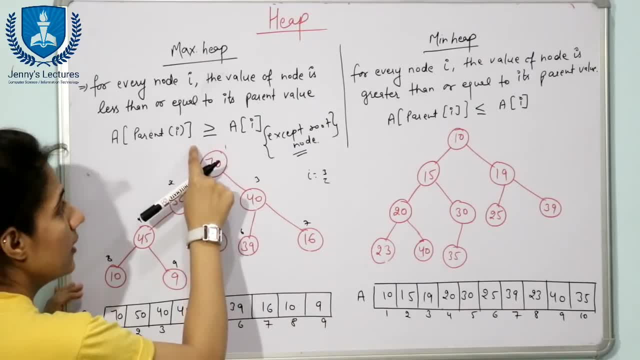 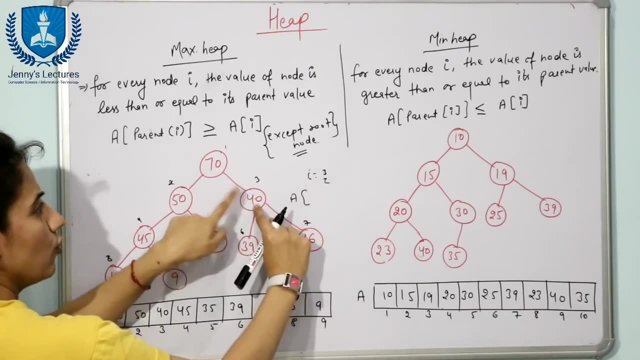 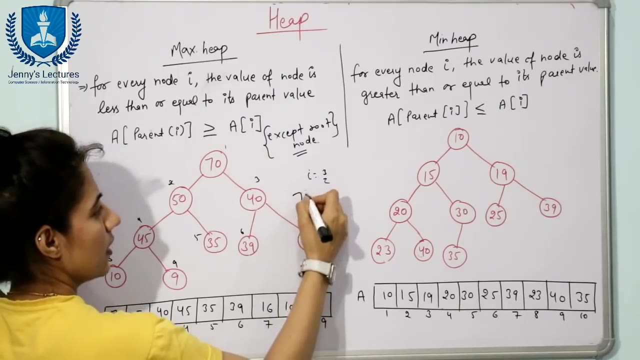 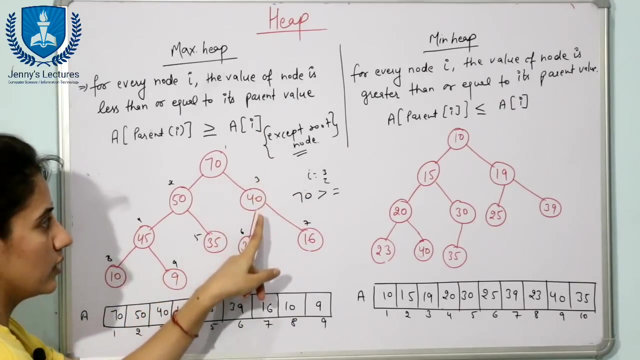 equal to three. this condition should be held. now check a of parent of i i i means three. fine. now, parent of this thing is one right. so the value of a of parent of i is 70. it means you can say 70.. would be greater than or equal to a of i. i value is 3, a of 3. what is a of 3 value, 40, 40, so this: 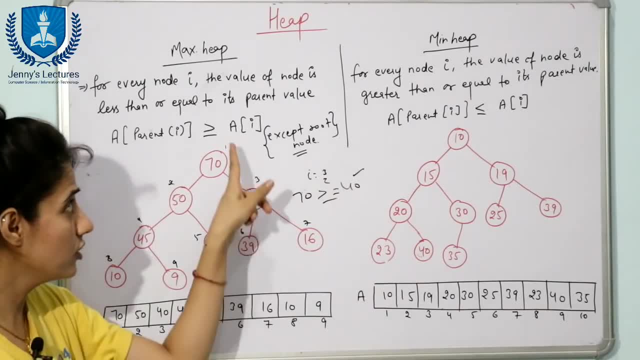 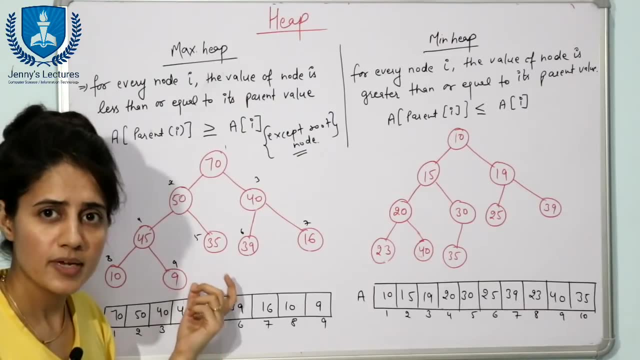 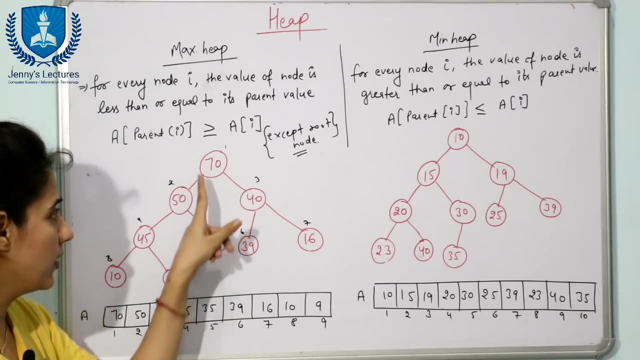 condition is true. 70 is greater than 40. yes, so this condition is true for all the nodes except root node, because root node is having no parent node. so this is max heap and in max heap the root node would always be the largest element here. there you can check, 70 is the largest element. 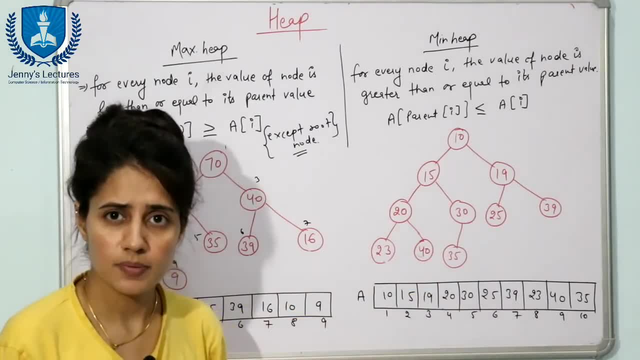 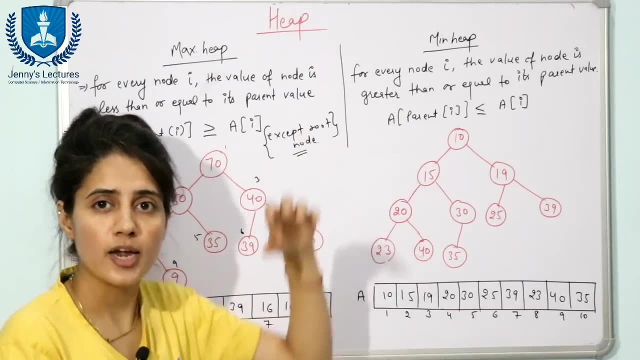 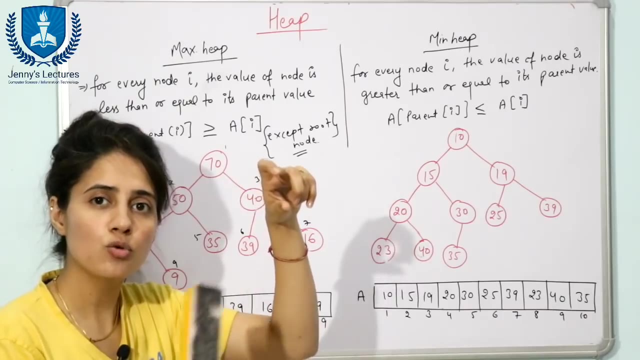 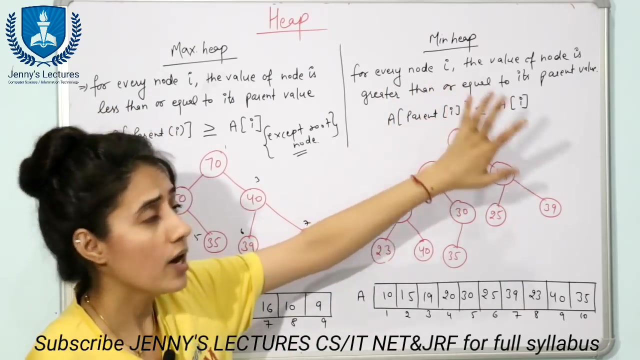 among all these: fine. now what about min heap? just opposite to this thing, parent node would be less than or equal to its child node. or you can say: for every node i, the value of that node would be less than or equal to all its descendant nodes. fine. or in another word, you can say: for every node i, the value of that node is greater than or equal. 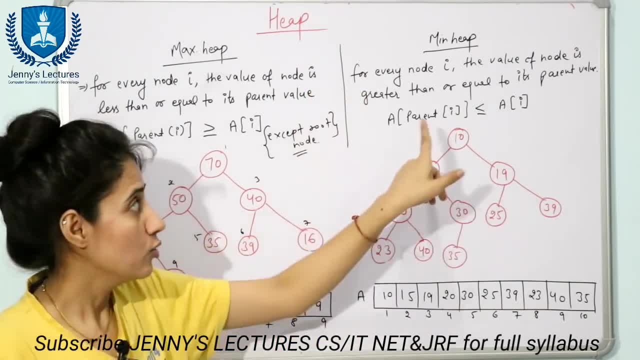 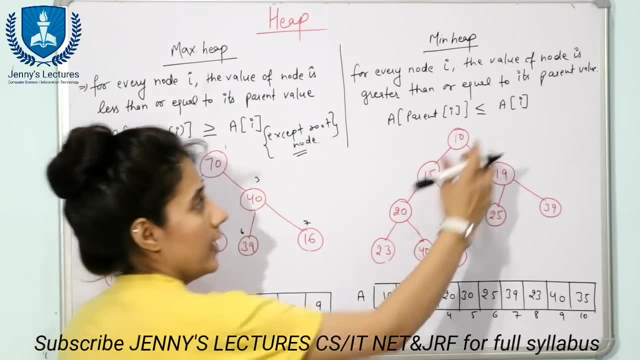 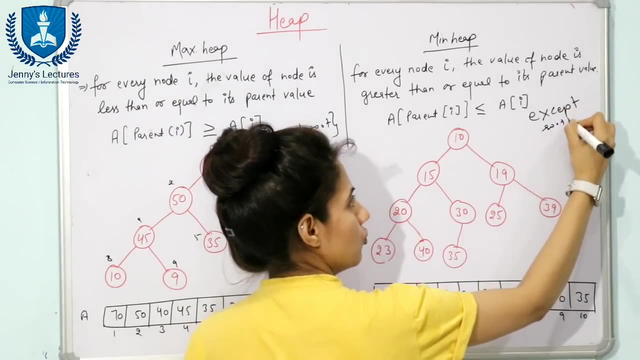 to its parent value. fine, so this condition should be held: a of parent should be less than equal to a of i. here, a of parent i would be greater than equal to a of i and same. this condition is true for all the nodes, but not for root node, except root node. why so? because root node is not having. 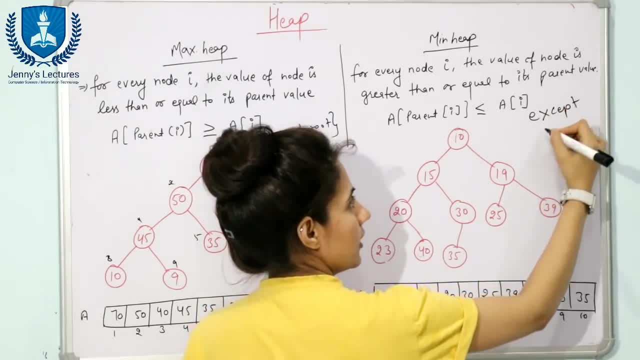 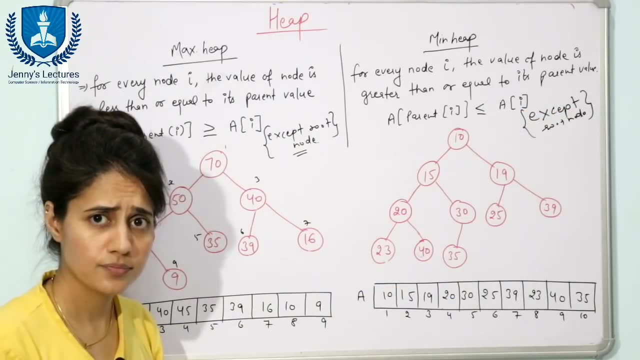 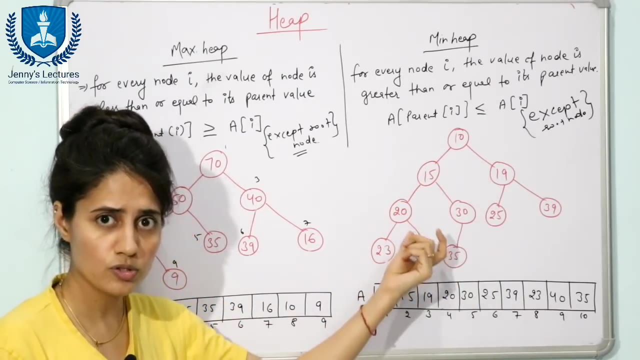 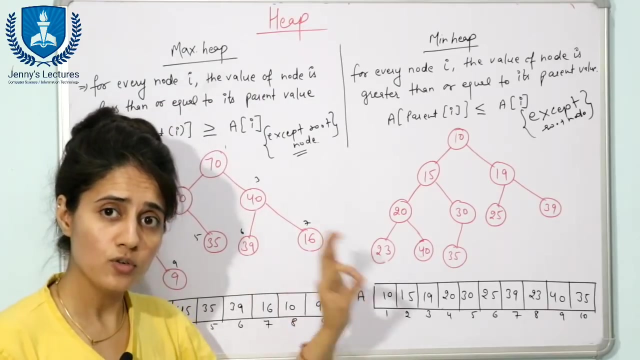 is true for all the nodes, but not for root node, except root node. why so? because root node is not having a any parent. fine, so for all the i i means the ith index, because we are going to store these uh nodes, these values, in the array and this is the i th index: 1, 2, 3, 4, up to 10. fine, so for every node, i. 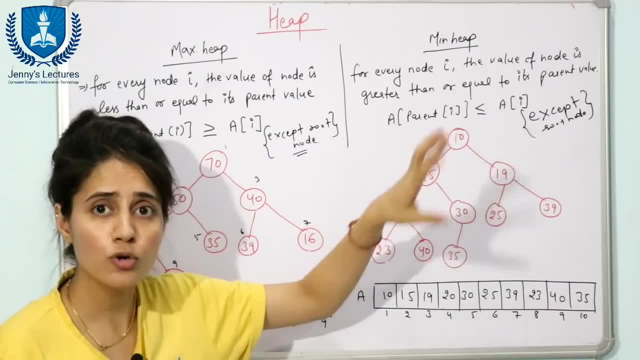 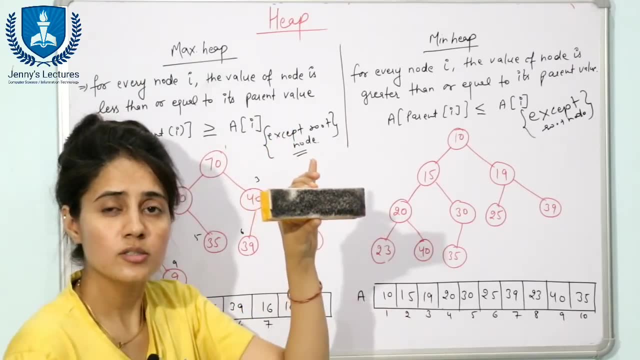 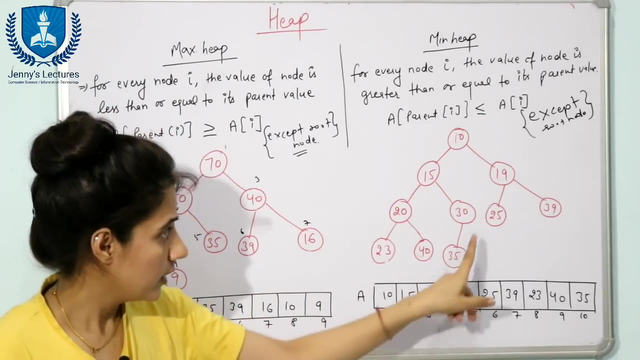 the value of that node would be either greater than or equal to its parent node, or another word you can say: the parent value should be less than or equal to its, less than or equal to its child node. so here, equal to m writing. that is why here duplicates are allowed. fine, say, see here, 30, here. also you can write 30, fine, because it's less than or equal to 10, and this is a lastly one. so we can divide by 30 all these values which i have here, and each of them should be less than or equal to to its child node. so here, for example, i am writing: that is why here duplicates are allowed. fine, see here 30. 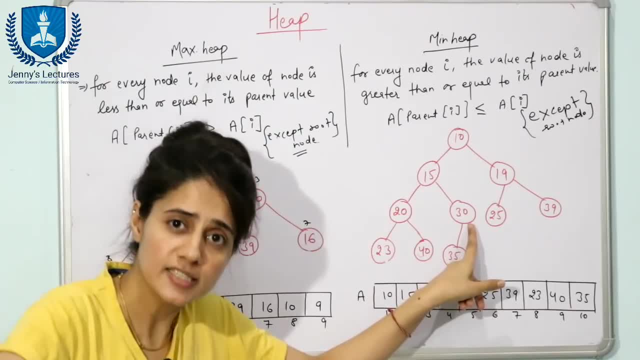 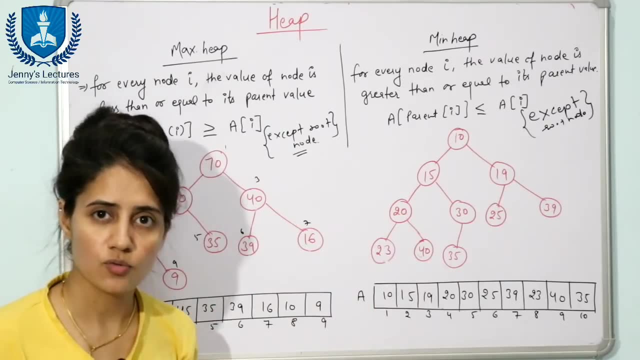 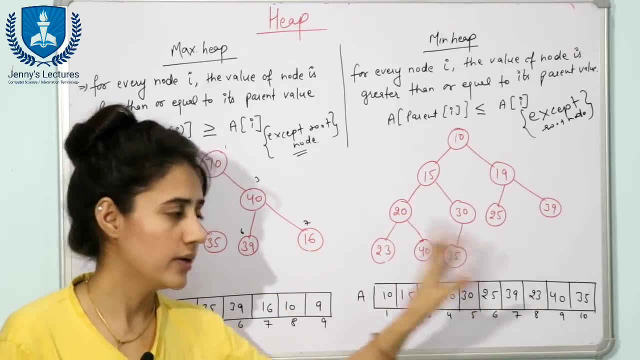 because the parent node would be should be either less than or equal to child node. here parent node should be greater than or equal to its child node. fine, so in min heap the root element would always be the minimum element among the array. here you can check: 10 is the minimum among all these. 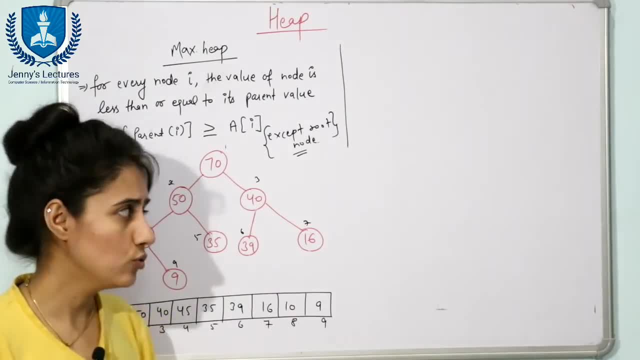 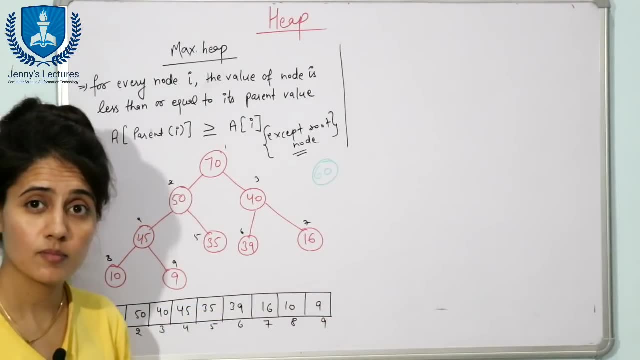 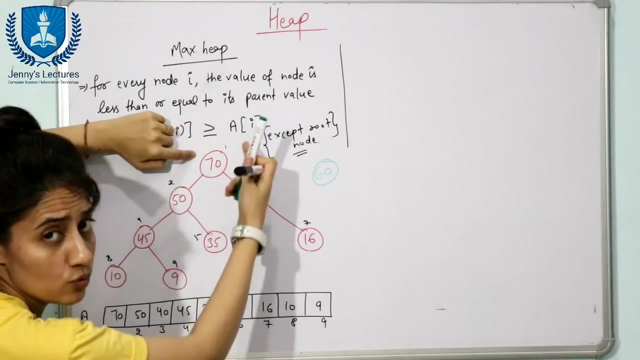 now see how to insert data in max heap. let us suppose we are going to insert a data, suppose, and data is 60.. fine, i want to insert 60 in this case. now simply what students will do? they'll check, they'll compare 60 with 70, or this 60 is less than in max heap. obviously root. sorry. 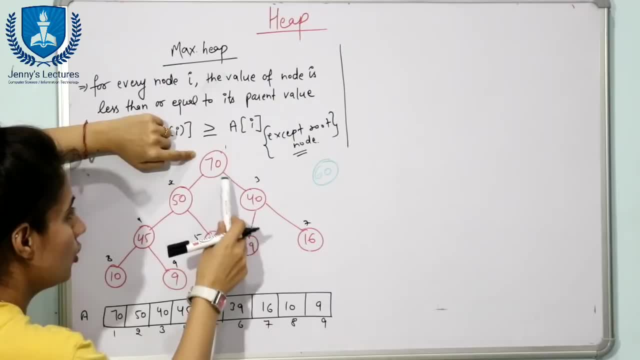 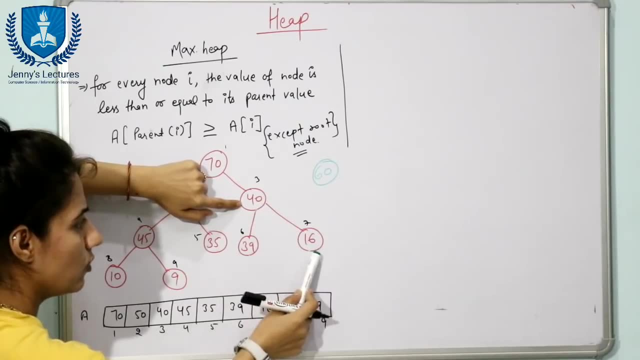 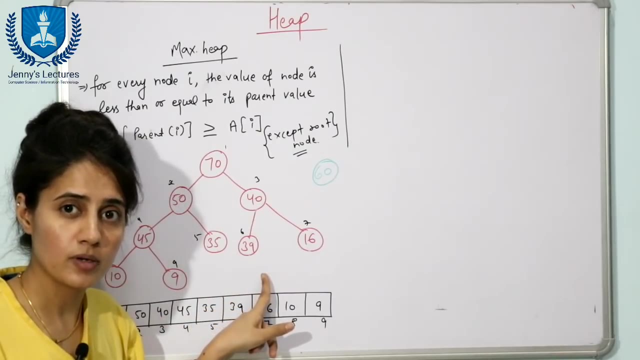 the parent value should be greater than or equal to its child value. so yeah, here 60, we cannot write so 50 and 40. minimum is 40. so we insert 60 here, 40 would go down and 16 would go down. but in that case it will not follow that complete binary tree property. 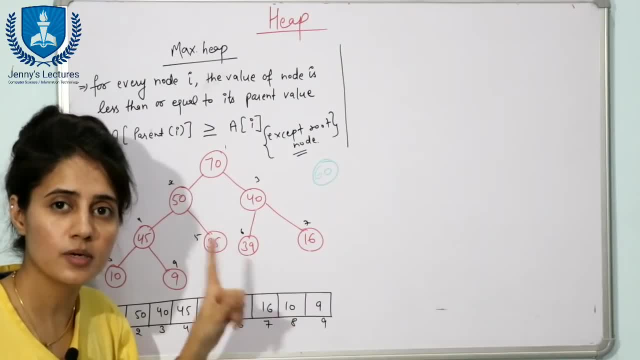 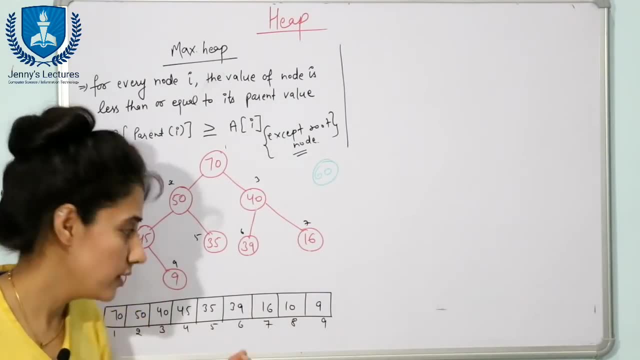 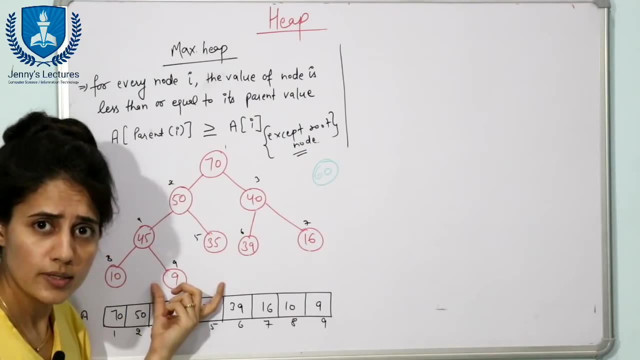 you have to take care of that thing also. heap heap is always a complete binary tree, fine. so see, you cannot insert from root. always the data would be inserted from leaf node. that is very important point. so in the leaf node we are going to insert the data, fine, and you have to check that. 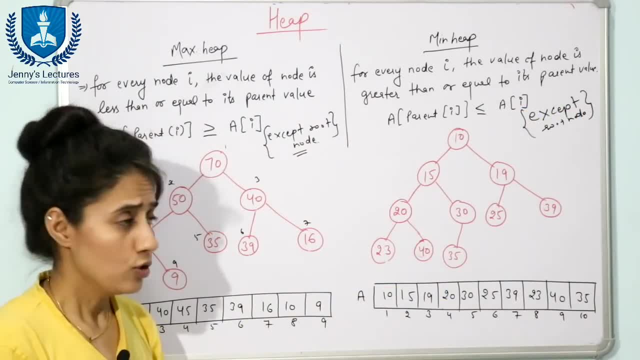 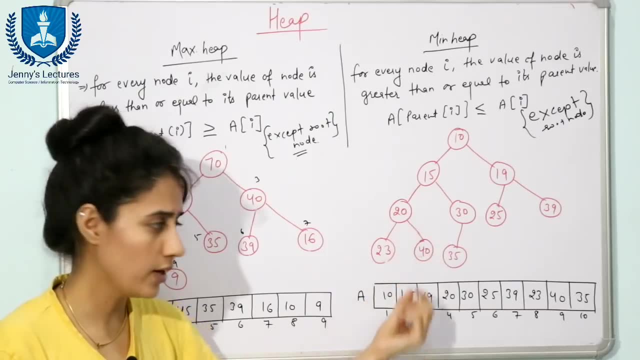 any parent, fine. so for all the i, i means the i-th index, because we are going to store these nodes, these values, in the array and this is the i-th index: 1, 2, 3, 4, up to 10. fine, so for every node. 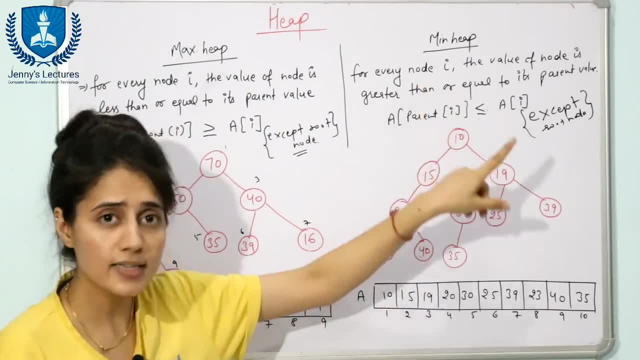 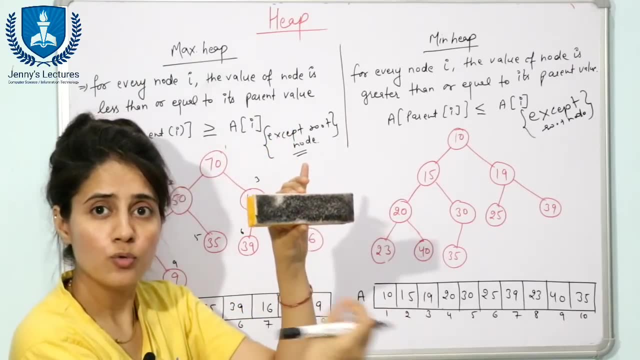 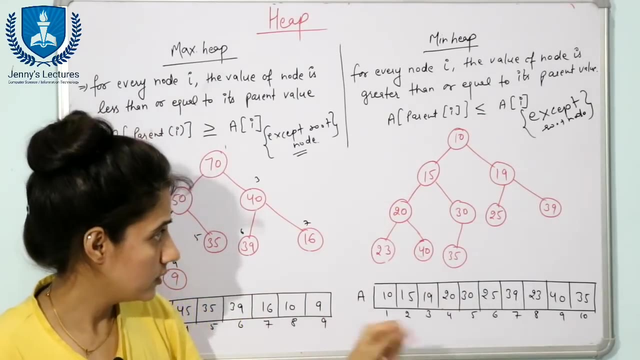 i, the value of that node would be either greater than or equal to its parent node, or in another word you can say the parent value should be less than or equal to its, less than or equal to its child node. so here equal to. i am writing. that is why here duplicates are allowed. fine, see here 30. 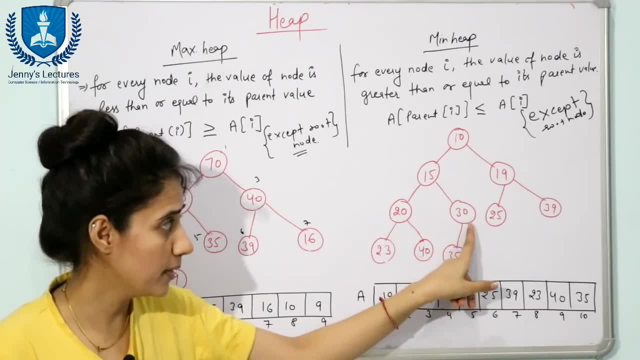 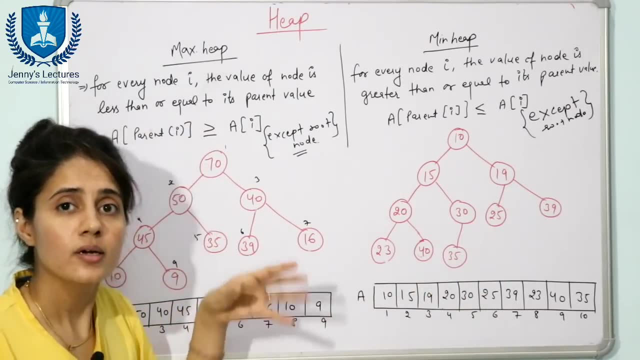 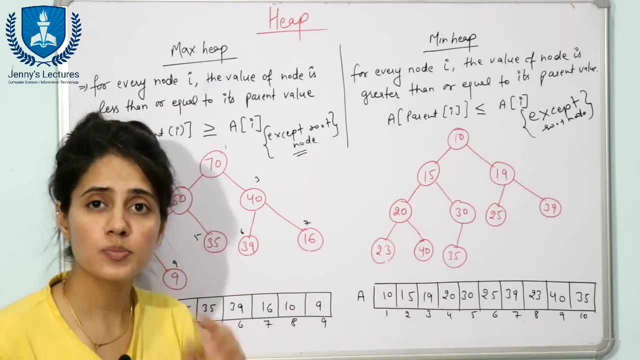 here also you can write 30. fine, because the parent node would be: should be either less than or equal to child node. here parent node should be greater than or equal to its child node. fine. so in min heap the root element would always be the minimum element among the array. here you can check, 10 is the minimum among all these. 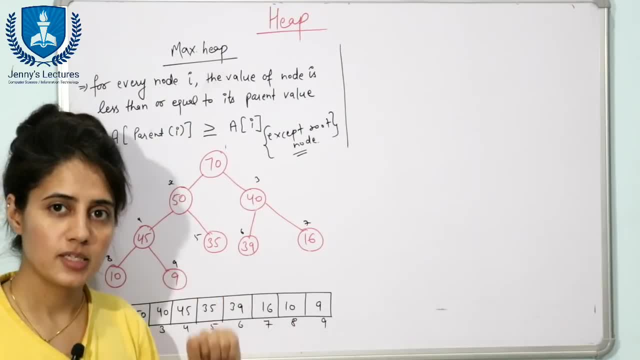 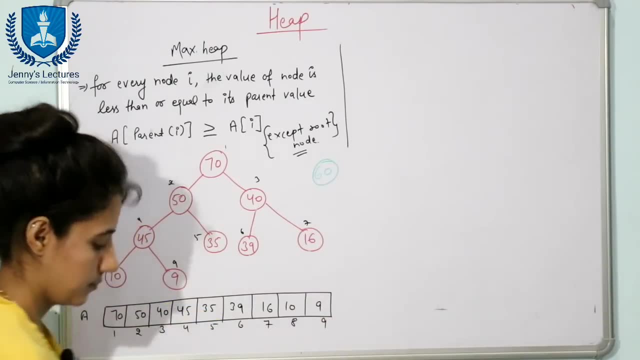 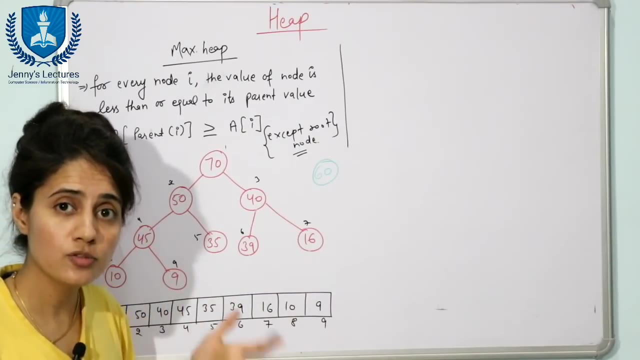 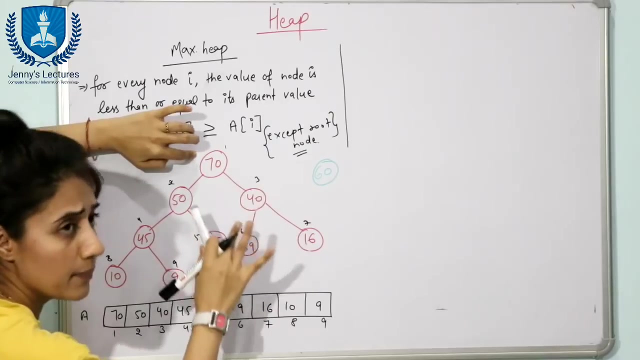 now see how to insert data in max heap. let us suppose we are going to insert a data. suppose in data is 60, fine, i want to insert 60 in this case. now simply what students will do. they'll check, they'll compare 60 with 70, or this 60 is less than in max heap, obviously root. sorry the parent. 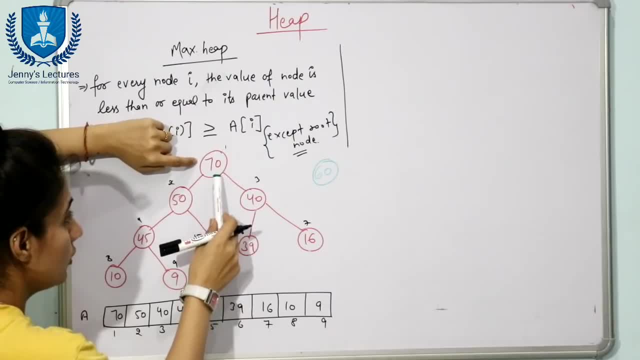 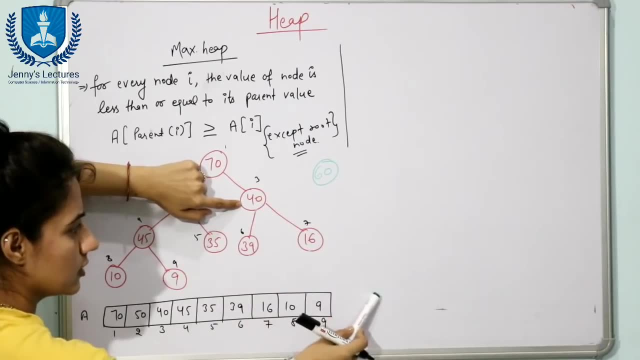 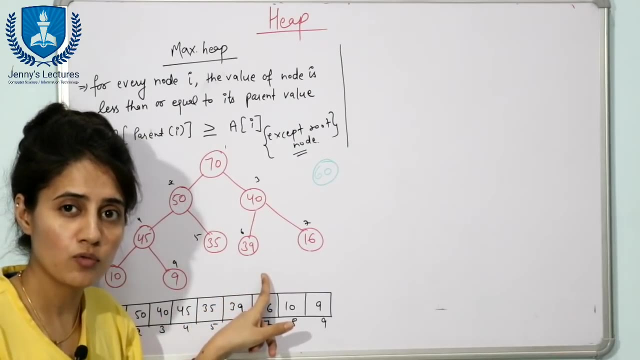 value should be greater than or equal to its child value. so yeah, here 60, we cannot write so 50 and 40. minimum is 40. so we insert 60 here 40 would go down and say 16 would go down. but in that case it will not follow that complete binary tree property you have to take. 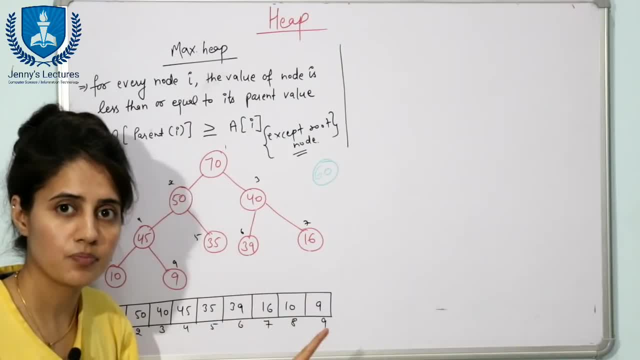 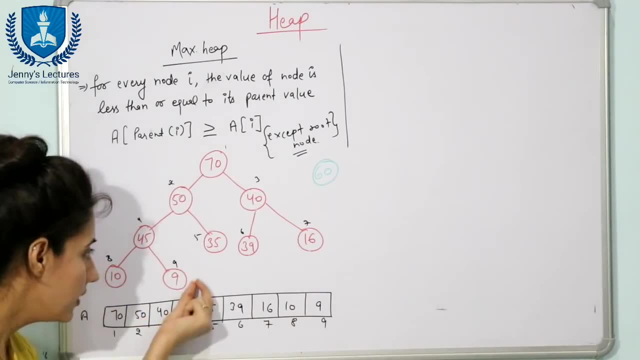 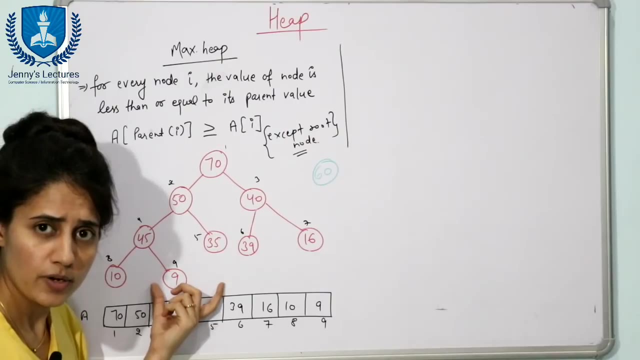 care of that thing. also. heap heap is always a complete binary tree, fine, so see, you cannot insert from root always. the data would be inserted from leaf node. that is very important point. so in the leaf node we are going to insert the data, fine, and you have to check that after. 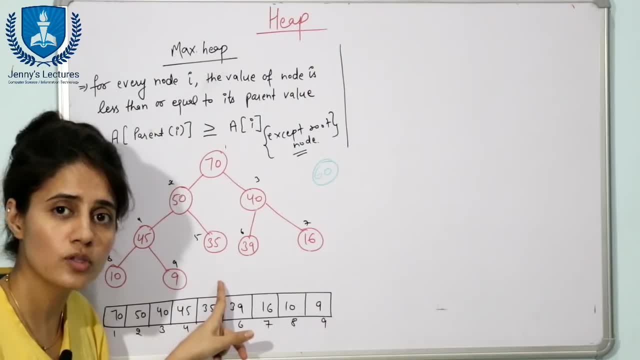 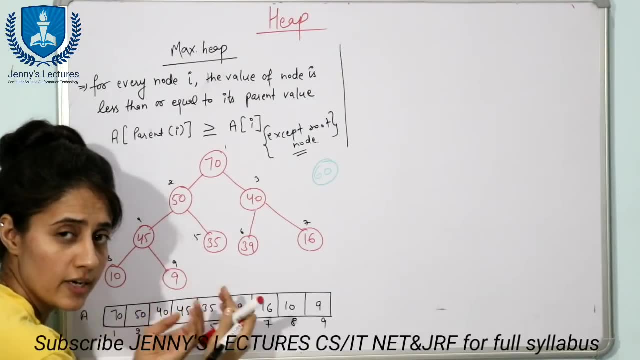 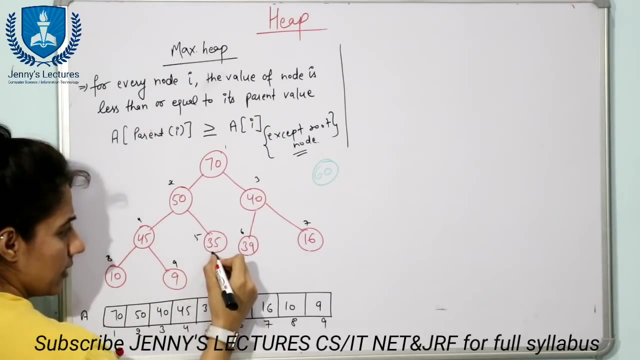 inserting this data in the leaf node, that tree should follow the property of constant value. so before inserting this data, we are going to check the property of absence, which retains your data in the complete binary tree. as we said, this data is actuated. here we have to. 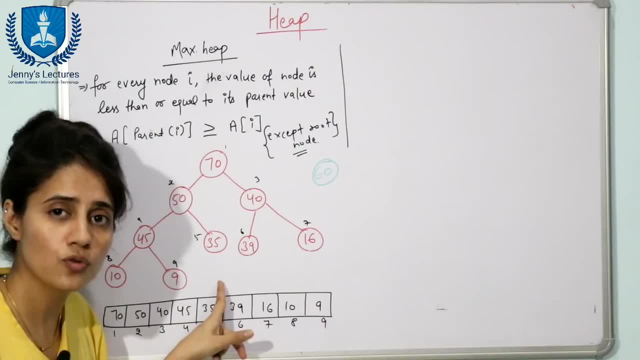 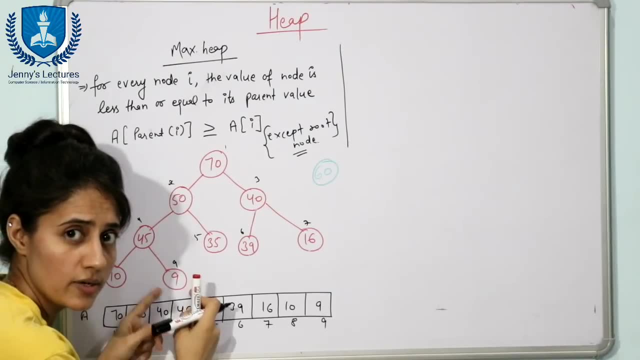 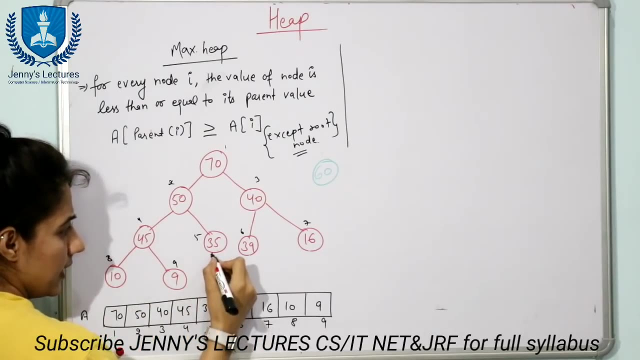 after inserting this data in the leaf node, that tree should follow the property of complete binary tree. fine, in complete binary tree in the last level we can, we can insert data as left as possible. we have to insert data as left as possible so we can insert 60 here to the left of 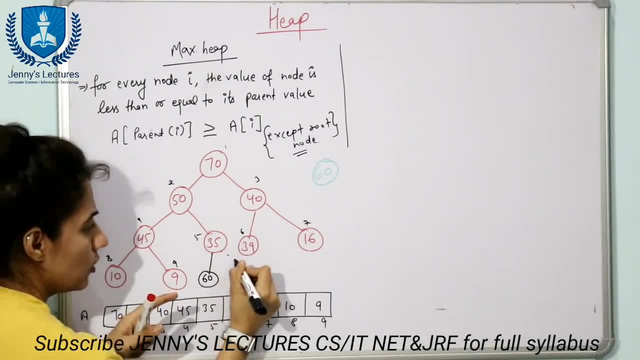 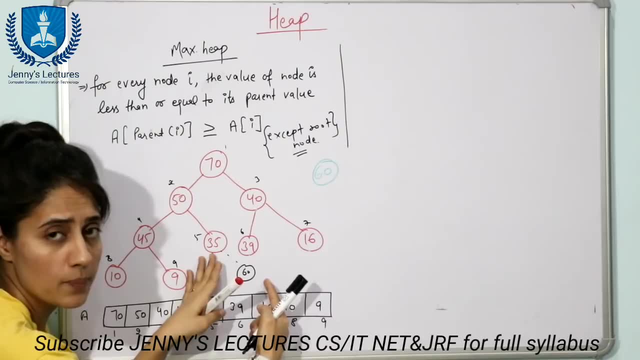 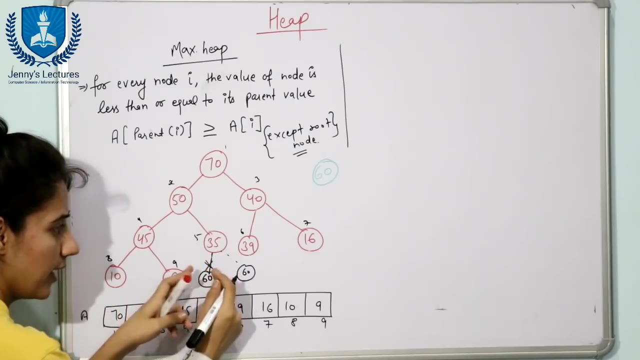 35. see, we cannot insert to the right of 60, 35 here, 60 no, because this will not. this will violate a property of almost complete binary tree. the data at the last level should be as left as possible. so you cannot leave, leave this blank and insert to the right side. you have to first of all fill left position, left child. 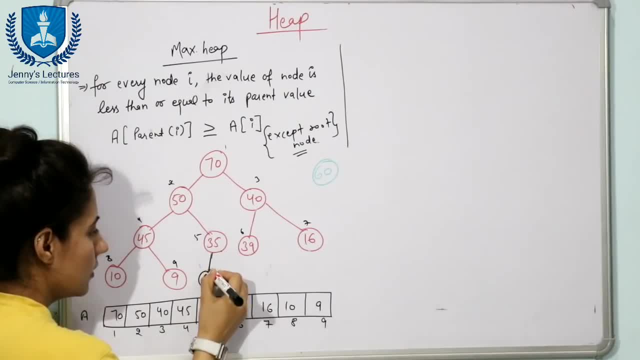 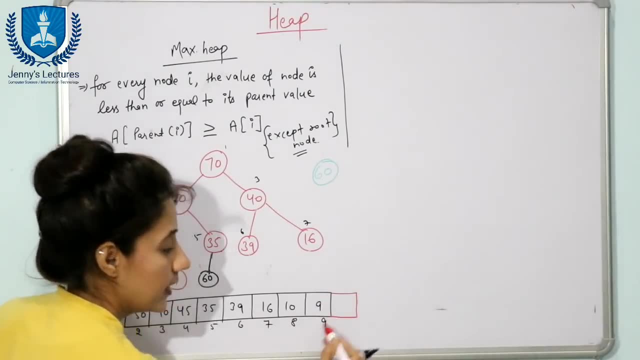 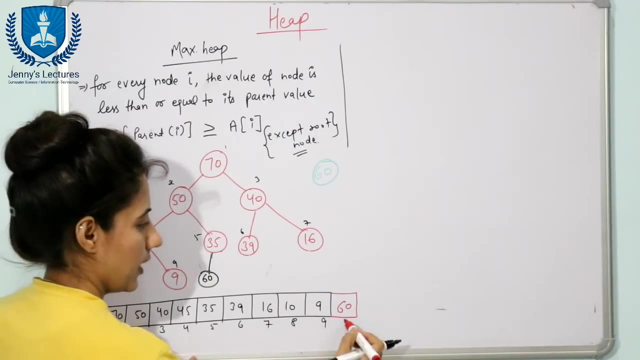 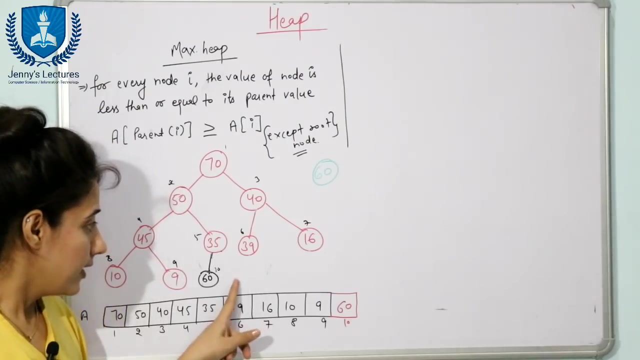 fine. so here we are going to insert 60 at this place. fine, and in array, where you will insert this, you will increase the size. size is n to n plus 1, and here i am going to insert 60 at 10th index. it is 10th index, it is not done. now see, it is satisfying the property of complete. 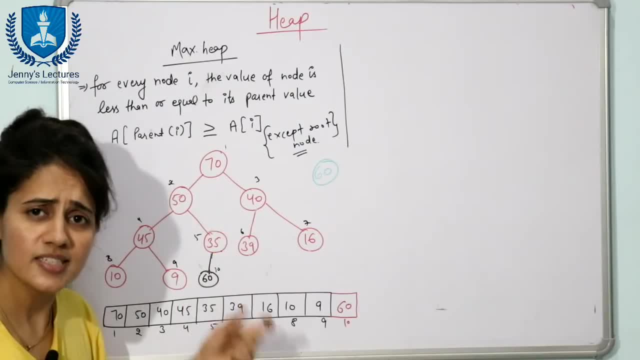 binary tree. but second thing is: it is max heap. is it satisfying the property of max heap after, after inserting the 60, you have to check that thing also. now, how to check that thing? see now 60. you have to check. you have to compare the 60 with its parent value. and what parent value should be in max. if parent value should be either greater than or equal to this 60, fine. now check: parent of the 60 is 35, fine, 35 is less than 60. so that is not allowed in max heap. parent should be greater than or equal to child node. so what? what will be done here? swapping? 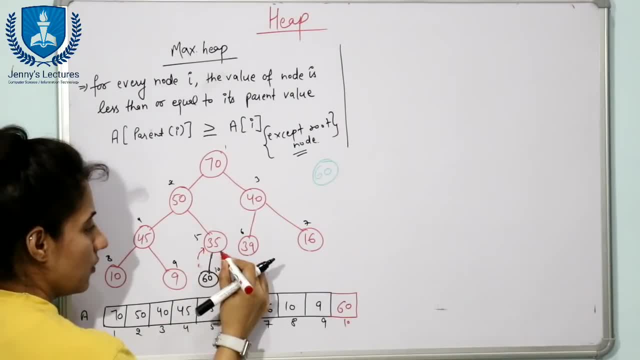 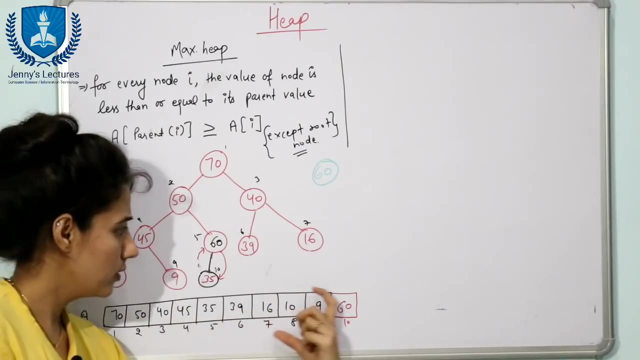 would be done: 60 would go up and 35 would go down. so here we will write 60 and here we will write what, 35. now, here i am making changes in this tree, but in in code. when you are writing a code, then this array would be there with you. this is just. 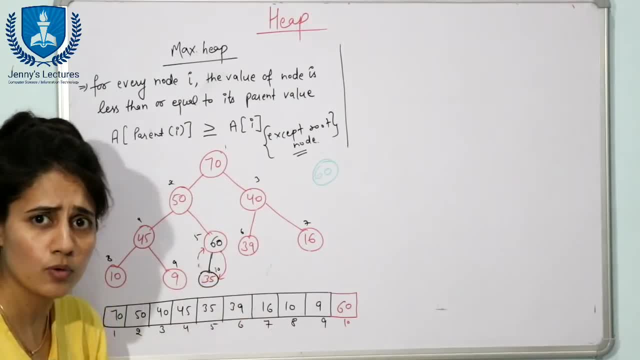 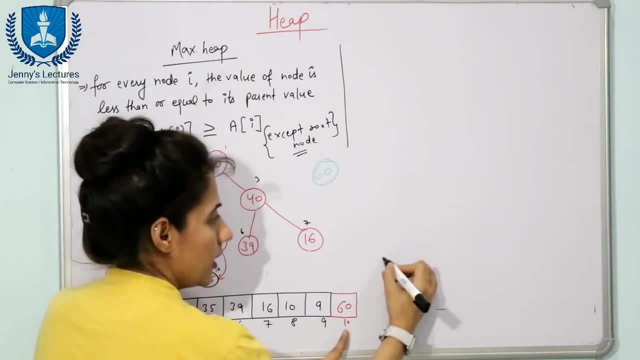 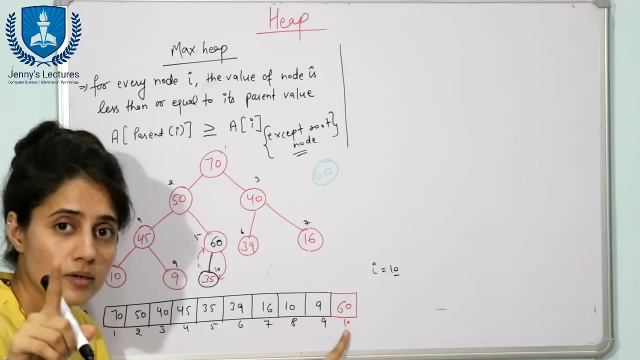 a pictorial representation. we cannot draw this thing when you are writing a program. so in program how it will be done, see 60 is at 10th index. so here you can say: i is equal to 10. now find out parent of this one. how to find out parent? i have just discussed the formula. formula is: 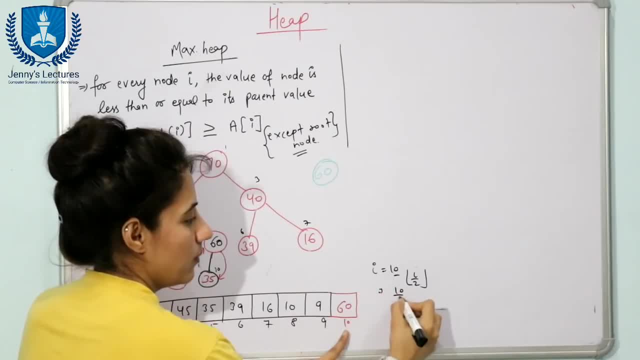 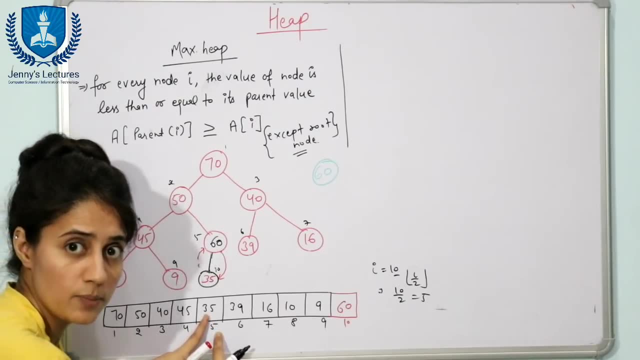 i divide by 2 and floor value. so 10 divided by 2 that is 5. so go to the index 5. at index 5 here it is 35. it means 35 is parent of 60 and 35 is less than 60. so that is not allowed. 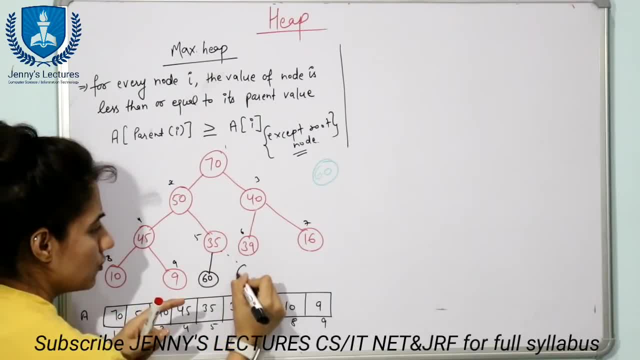 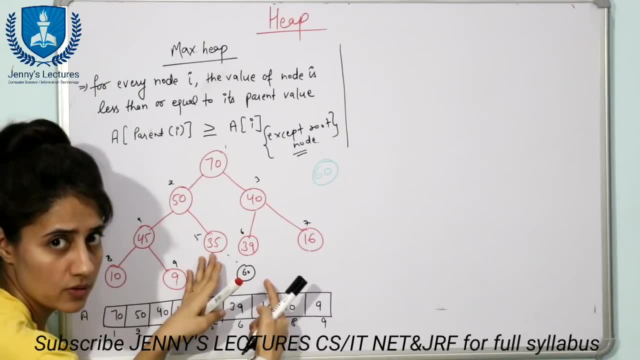 check that all data is 2018K. so we have to say: is this data is taken or is gathered in complete binary tree? right, and this data rereaders we can easily insert here. this data relies for communicating data through complet été tree. that way you can move 자본成 Clint. 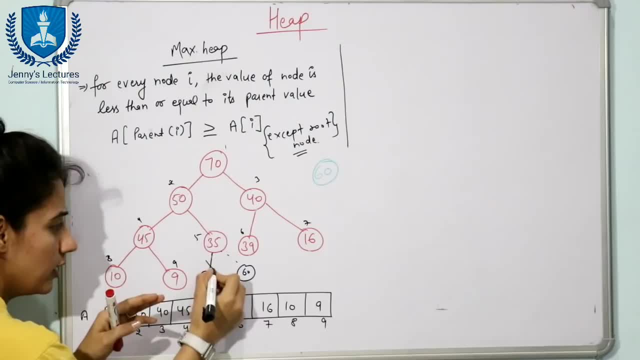 institute of complete binary tree: fine, in complete binary tree, in the last as possible. so you cannot leave. leave this blank and insert to the right side. you have to first of all fill left position, left child- fine. so here we are going to insert 60 at this place, fine, and in. 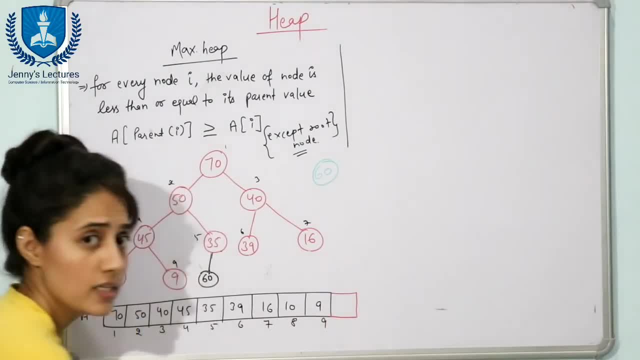 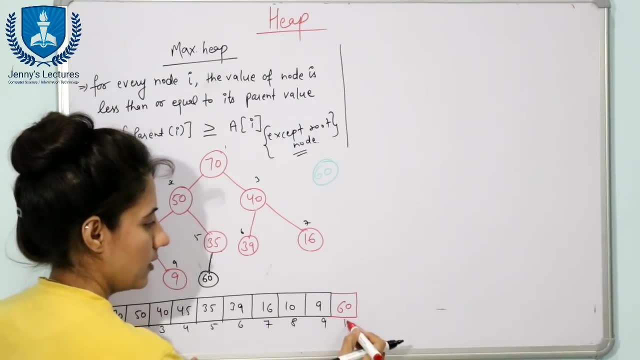 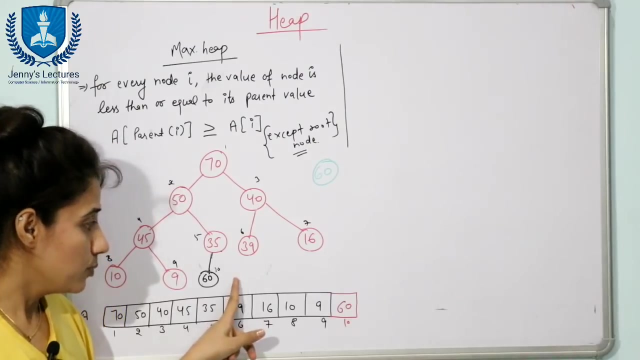 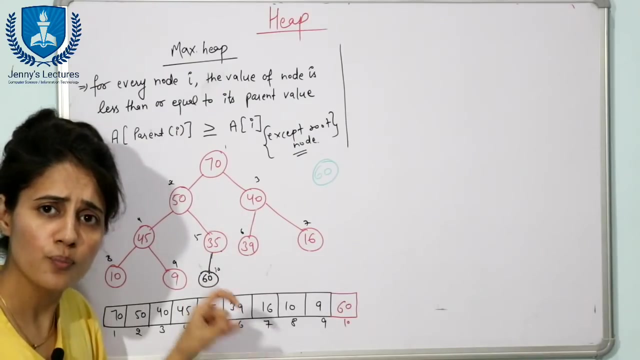 array where you will insert this, you will increase the size. size is n to n plus 1, and here i am going to insert 60 at 10th index. it is 10th index. it is not done. now see, it is satisfying the property of complete binary tree. but second thing is, it is max heap. is it satisfying the property of max? 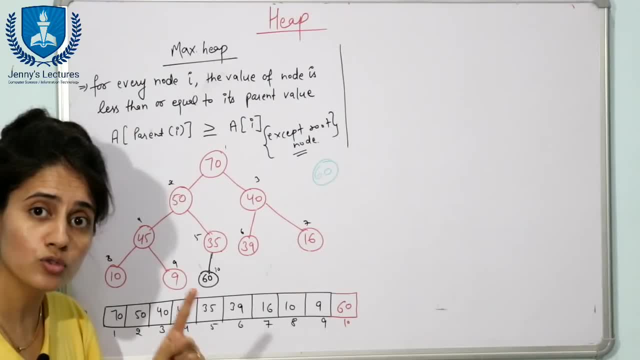 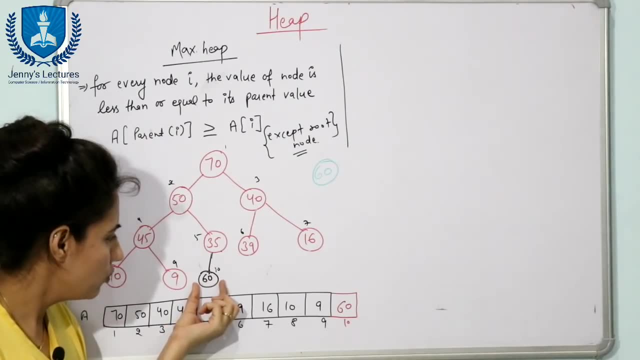 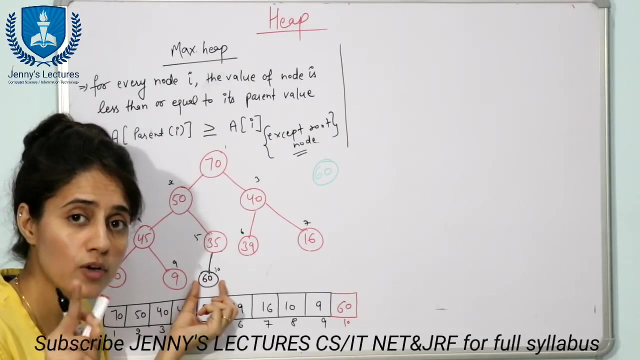 heap after, after inserting the 60, you have to check that thing also. now how to check that thing? see now 60. you have to check, you have to compare the 60 with its parent value and what parent value should be in max heap. parent value should be either greater than or. 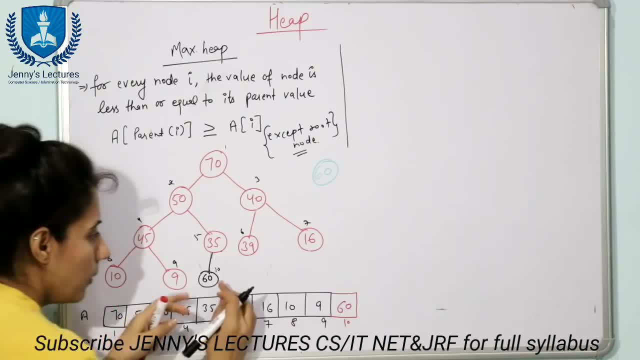 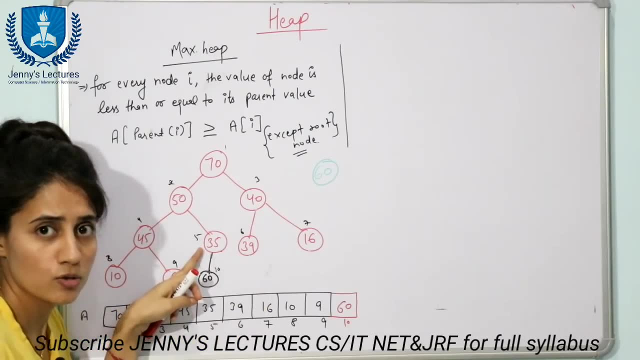 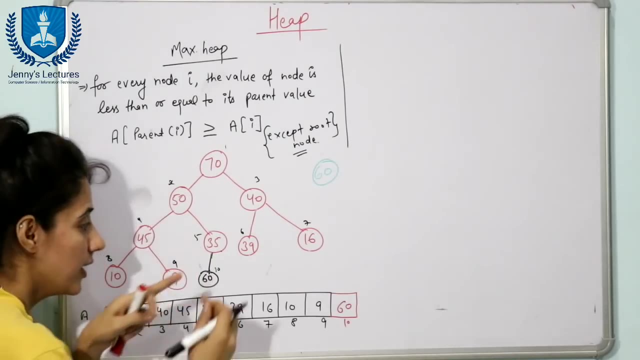 equal to this: 60- fine. now check parent of the: 60 is 35, fine, 35 is less than 60, so that is not allowed. in max heap, parent should be greater than or equal to child node. so what? what will be done here? swapping would be done: 60 would go up and 35 would go. 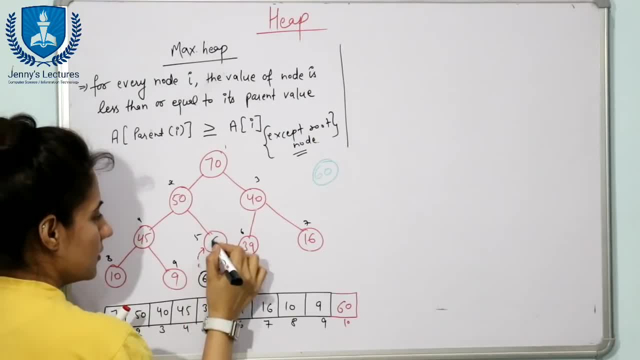 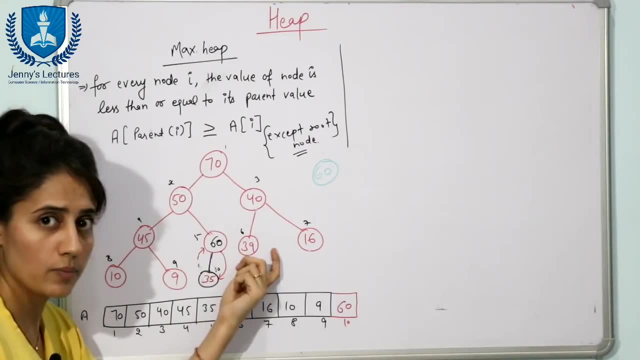 60 would go up and 35 would go down. 60 would go up and 35 would go down down. so here we will write 60 and here we will write what, 35. now, here i am making changes in this tree, but in in code. when you are writing a code, then this array would be there with you. 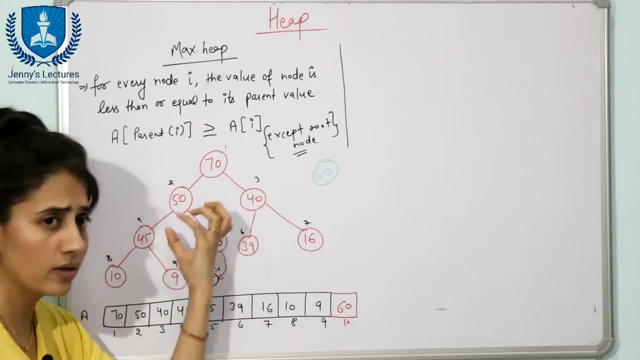 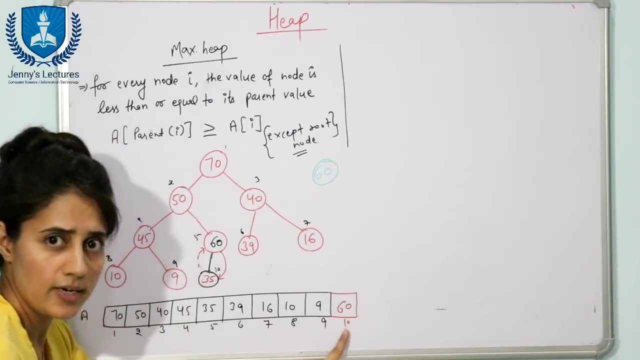 this is just a pictorial representation. we cannot draw this thing when you are writing a program. so in program how it will be done, see 60 is at 10th index. so here you can say: i is equal to 10. now find out parent of this one. how to find out parent? i have just discussed the formula. formula is: 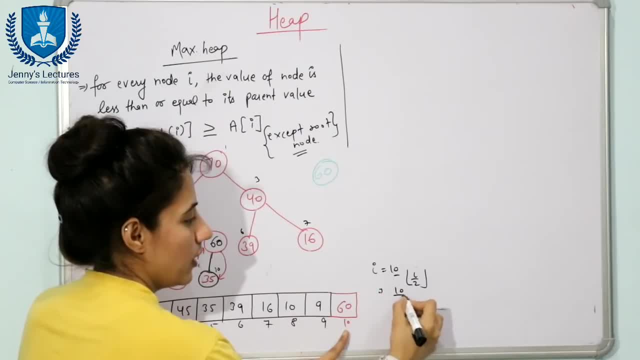 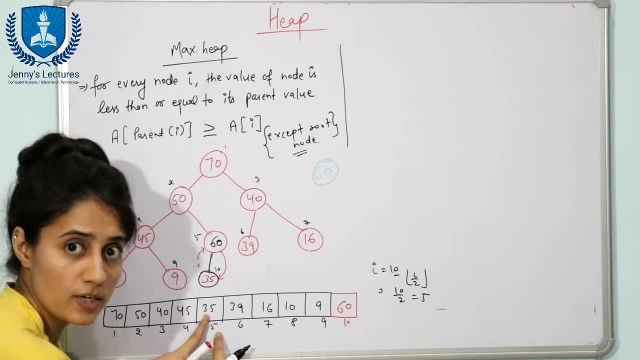 i divide by 2 and floor value. so 10 divided by 2 that is 5. so go to the index 5. at index 5 here is 35. it means 35 is parent of 60 and 35 is less than 60. so that is not allowed in. 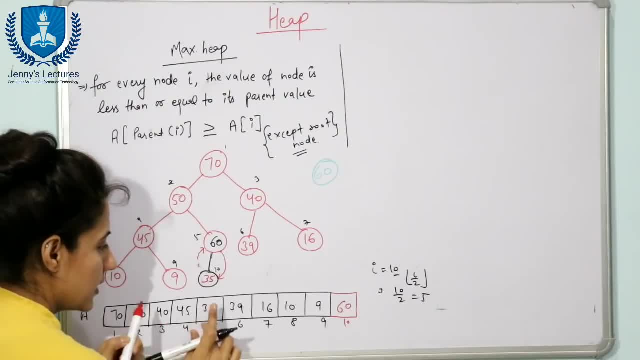 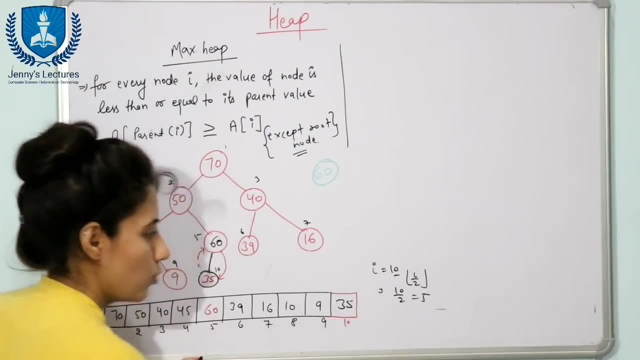 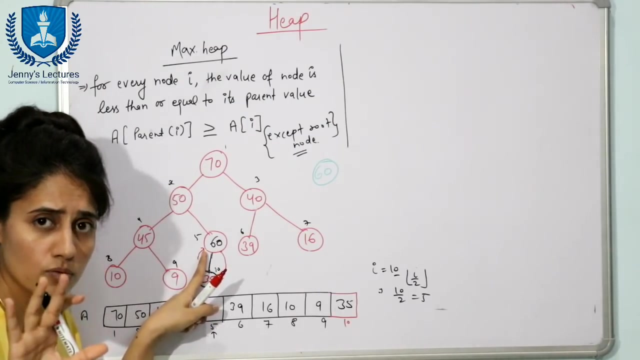 max heap now in array. what will be done? the 60 would go here and 35 would go to main array and we just need to have the 6th, 8th and we have this 1 plus this, 1 plus this two and we have 6th, 6th and we have 6th, 3rd and we have 7th, which is the step 1,, 2,, 3rd step. 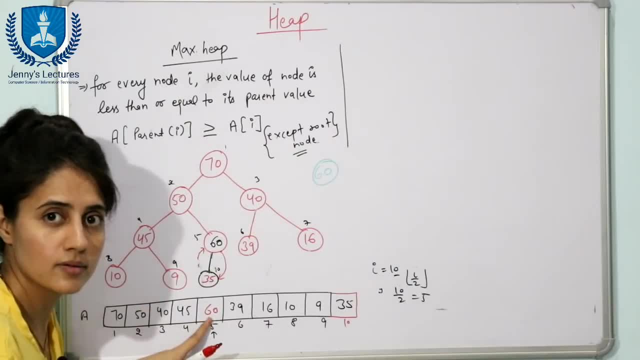 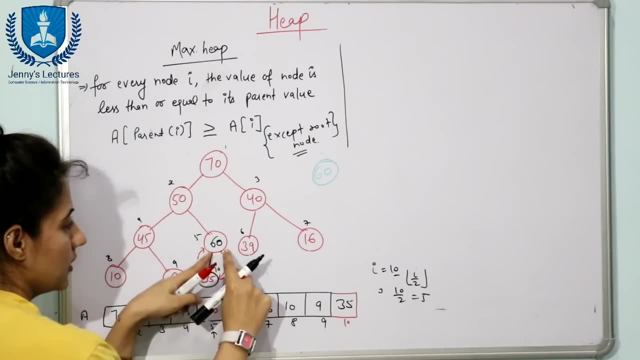 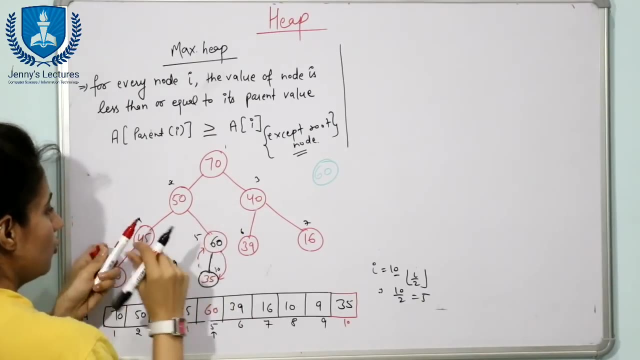 but distance between two 드묽은- 1, 2 and 2 is the step Z and we can write the same. so we can write counter-rotate over 3 times and we can write 50. so parent is less than 60. now again swapping would be done, 60 would go up and this 50 would go. 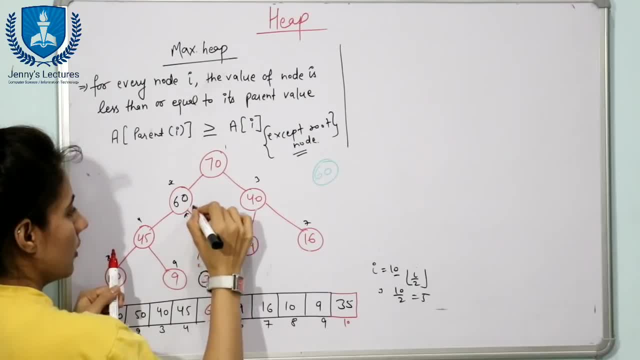 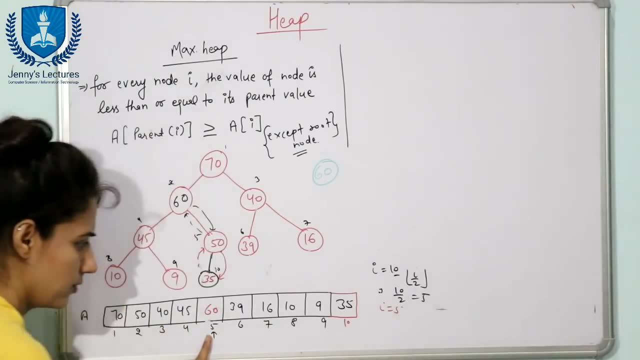 down. fine swapping would be done here in this case. now, here i value is. now i value is 5. now find out parent 5 divided by 2 and floor value means 2.5. if you are taking floor value, then 2, so go to the index 2. here we have 50. it means 50 is parent of 60, but 50 is less than 60. that 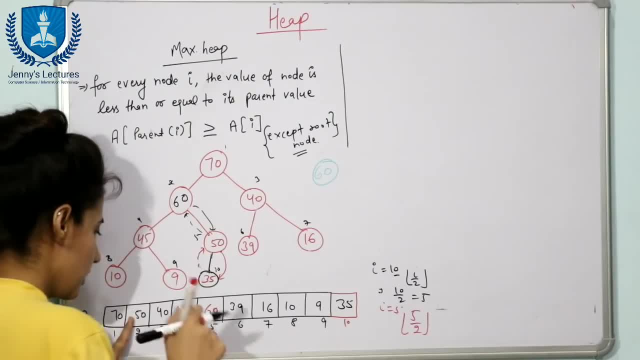 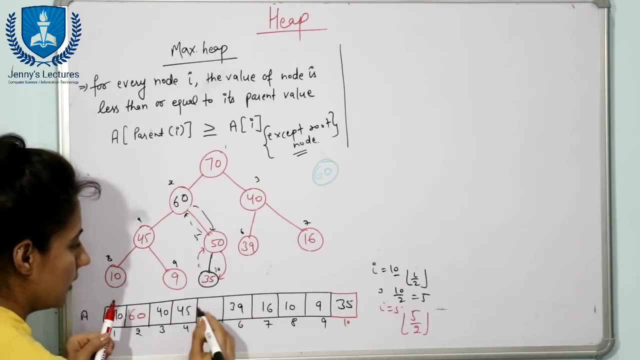 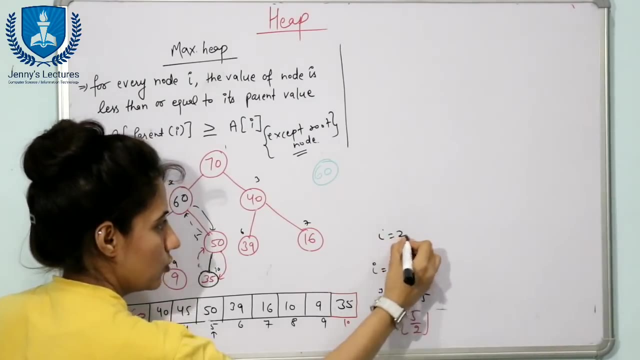 is not allowed in max heap, that is not following the max heap property, max heap property. so swapping would be done. so here we will write 60 and here we will write in the array 50. fine, now i value is 2. now i value is 2. again we have to check parent, parent till we, till we reach. 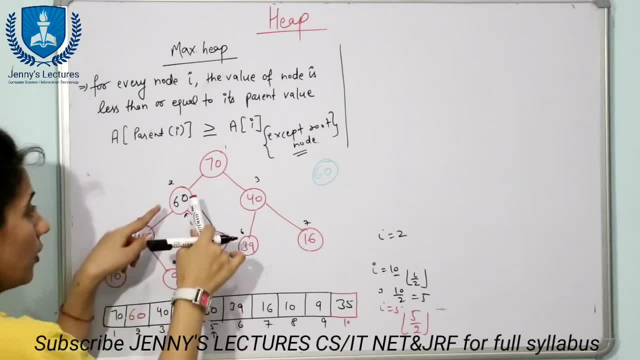 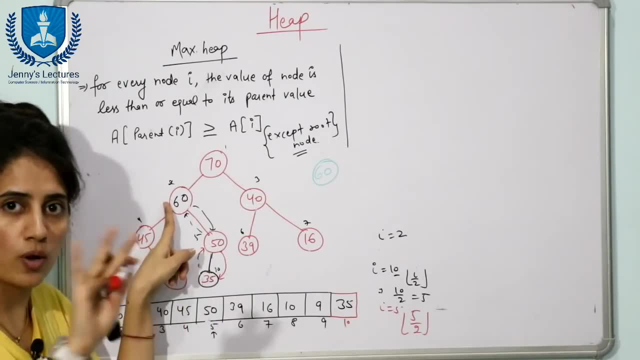 i value is 2. now i value is 2 again. we have to check parent, parent till we, till we reach i value to 1 means to the root. now here, check with parent. parent is 70, 70 is greater than 60. that is satisfying maxi property. now no swapping would be done. fine, now this is done. now in array in this: 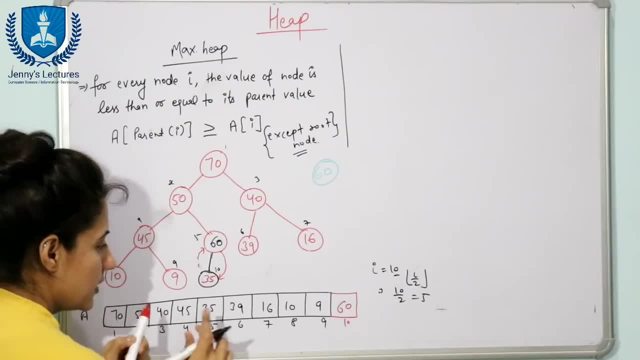 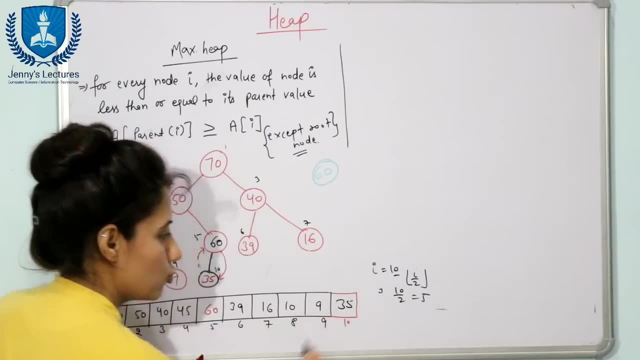 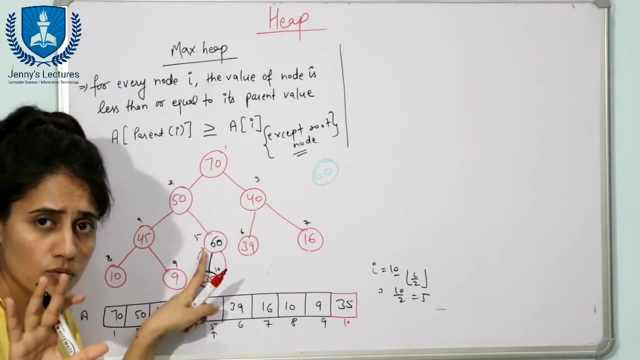 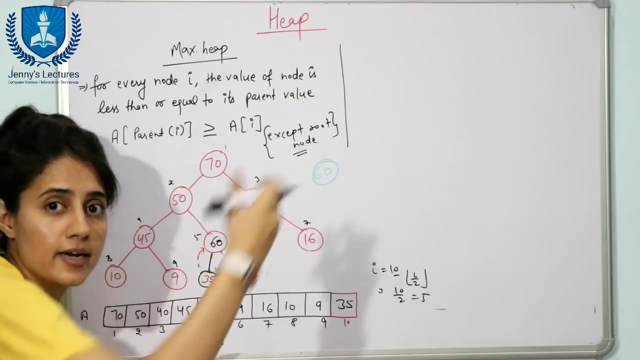 in max heap. now in array, what will be done? the 60 would go here and 35 would go there means swapping. fine, now here we have 60, but it is not done now because again we are going to check, again, we are going to compare the 60 with its parent. fine, till we reach to the root node. 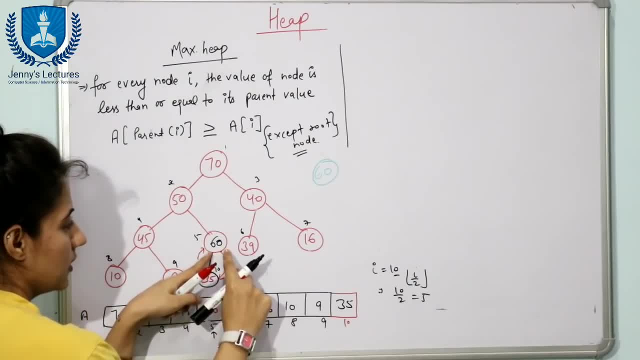 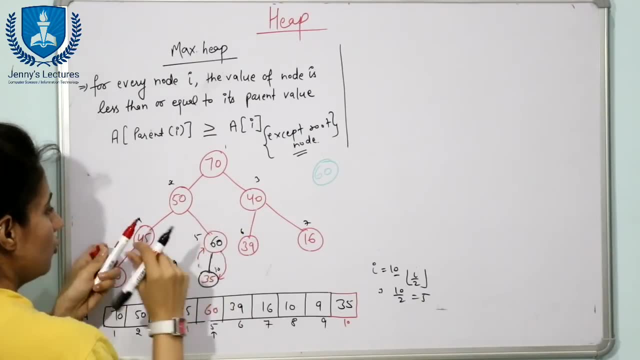 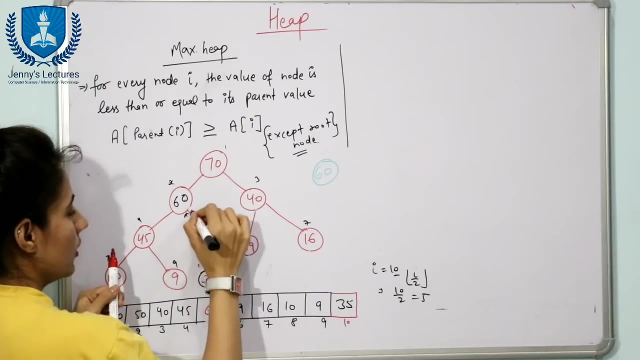 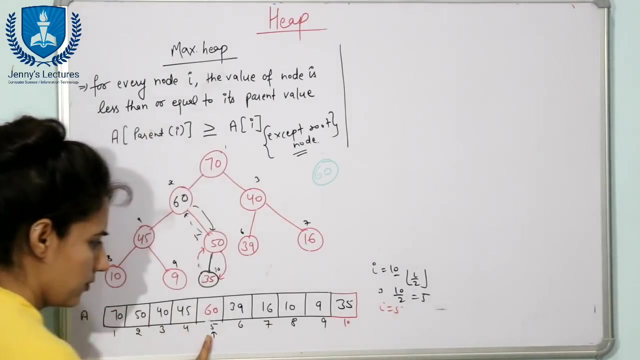 fine, now, see now in check here: 60 parent of 60 is 50, so parent is less than 60. now again, swapping would be done. 60 would go up and this 50 would go down. fine, swapping would be done here in this case. now, here i value is: now i value is 5. 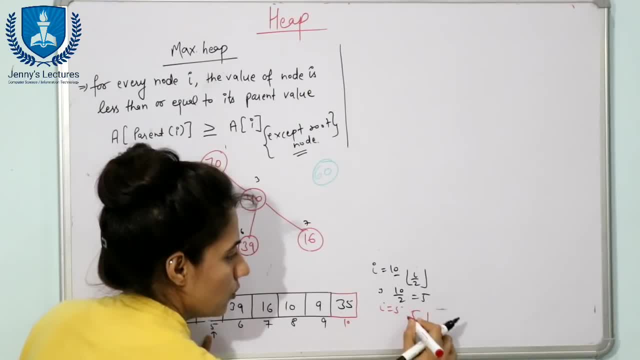 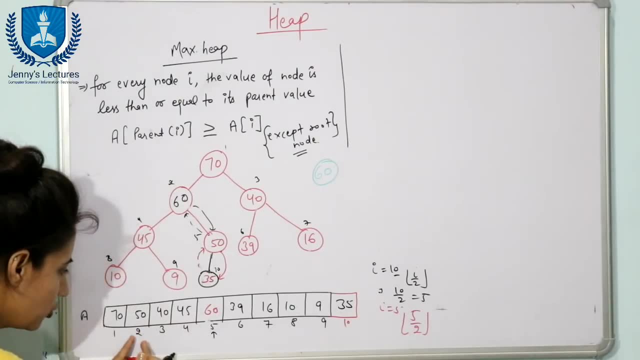 now find out: parent 5 divided by 2 and floor value means 2.5. if you are taking floor value, then 2. so go to the index 2. here we have 50. it means 50 is parent of 60, but 50 is less then 0 was applied. so if you add ainda 2, you can see: 5 divided by 2 means 2 is less than 60. so blue 2 is less than 25. yes, 3ile 50 divide by 2 would be down 1 if you are taking floor value. ah, so do you see? 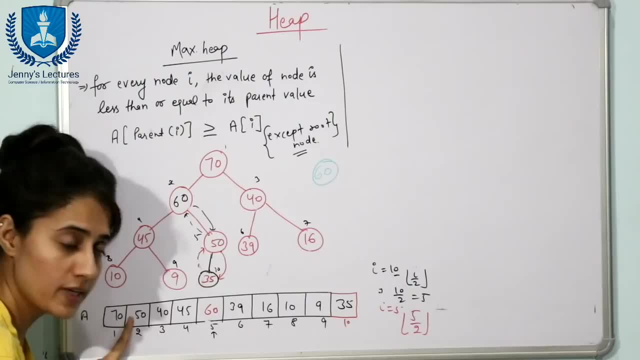 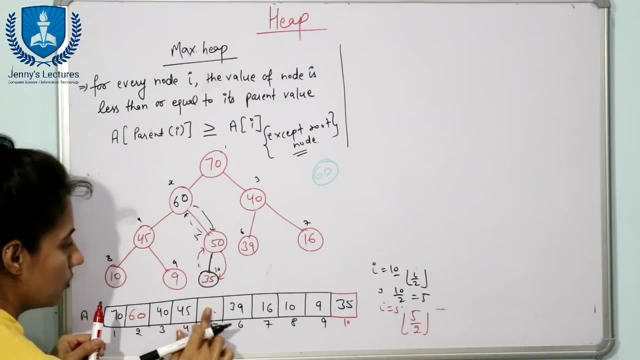 Less than 60. That is not allowed in max heap. That is not following the max heap property. So swapping would be done. So here we will write 60. And here we will write in the array 50.. Fine, Now i value is 2.. 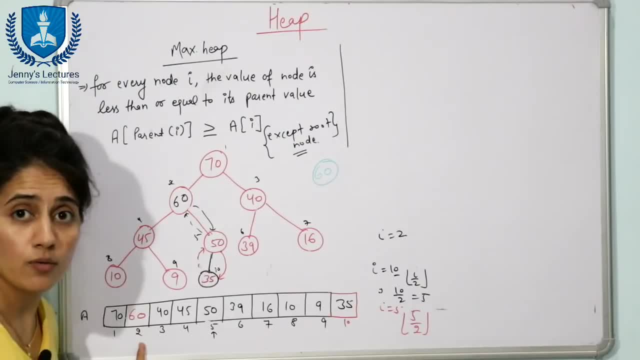 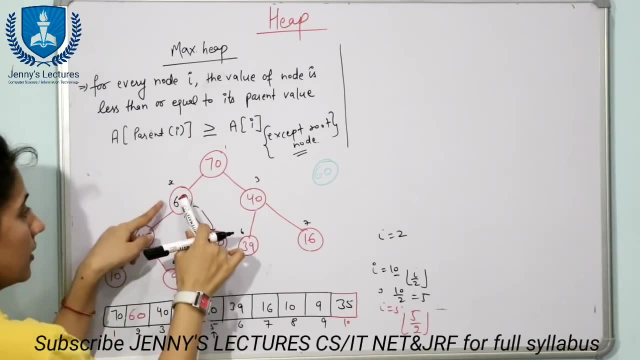 Now i value is 2.. Again, we have to check parent Till we reach i value to 1. Means to the root. Now here check with parent. Parent is 70. 70 is greater than 60. That is satisfying max heap property. 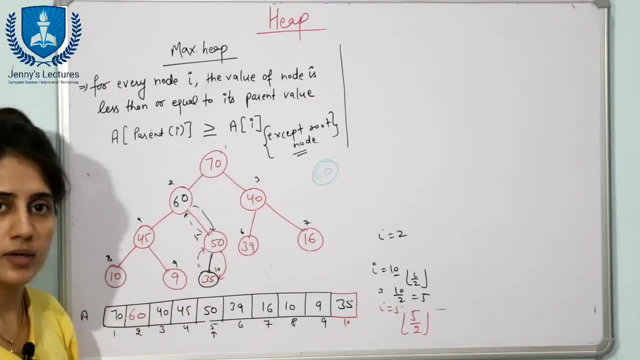 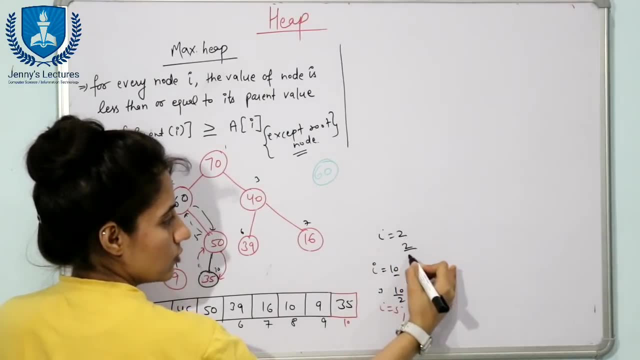 Now, no swapping would be done. Fine, Now this is done. Now in array. In this array, representation check i is 2.. Now find out: root 2 by 2. i divided by 2. Floor value: That is 1.. 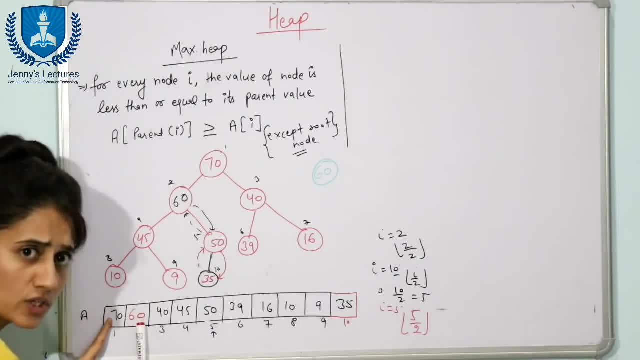 Go to the index 1. At 1 we have 70. Means 70 is parent of 60. Right 70 is greater than 60. So that is fine. No swapping would be done. Fine, So this is done now. 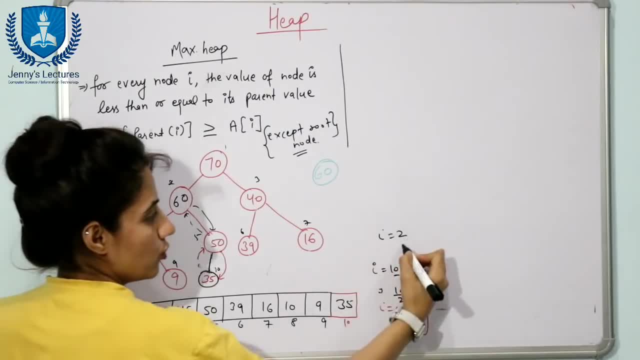 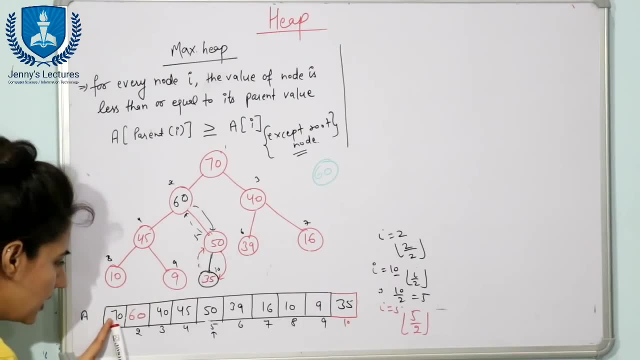 array representation. check: i is 2. now find out root 2 by 2. i divided by 2, floor value, that is 1. go to the index 1 at 1 we have 70 means 70 is parent of 60 right. 70 is greater than 60, so that 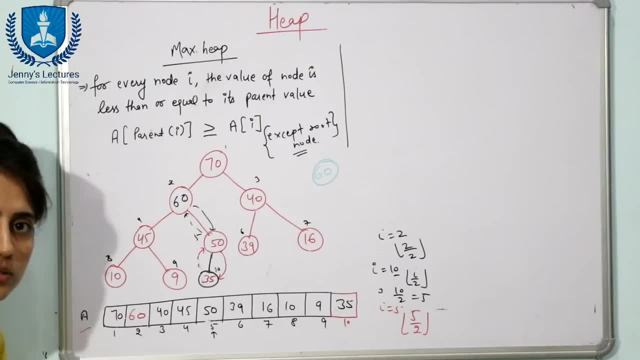 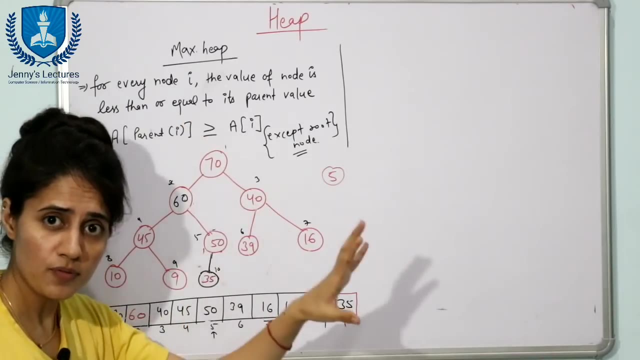 is no swapping would be done. fine. so this is done. now insertion of 60 is done. after insertion, the array would be something like this and tree would be something like this: now suppose i want to insert an element having value 5. now we cannot insert from root. simple funda is insert data from the. 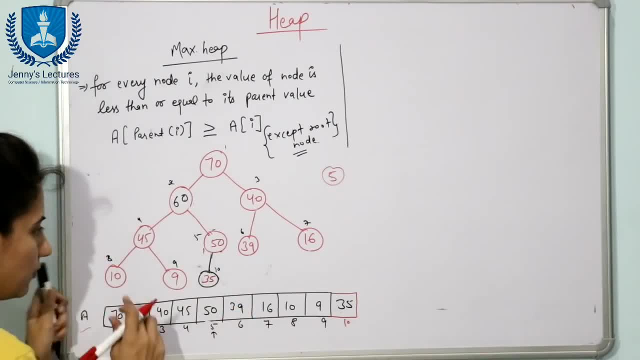 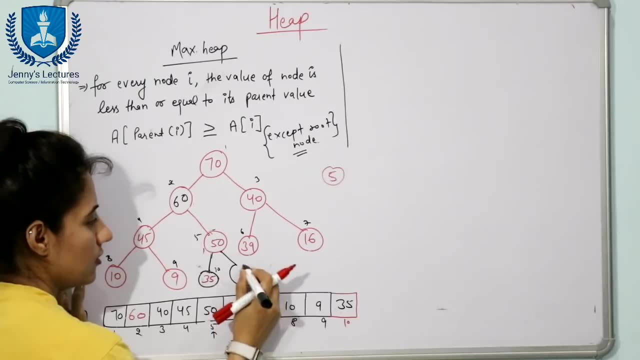 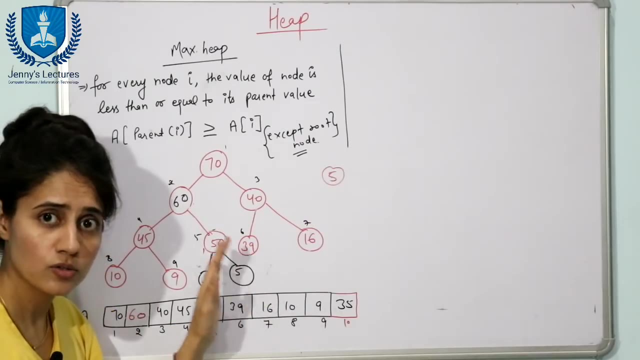 leaf node in the tree. fine, in the leaf node where i can insert, i can insert to the this: to the right of 50. I can insert 5. you have to take care of that thing also. after inserting this 5 in the leaf, note that that tree holds the, still holds the property of complete binary tree. fine. 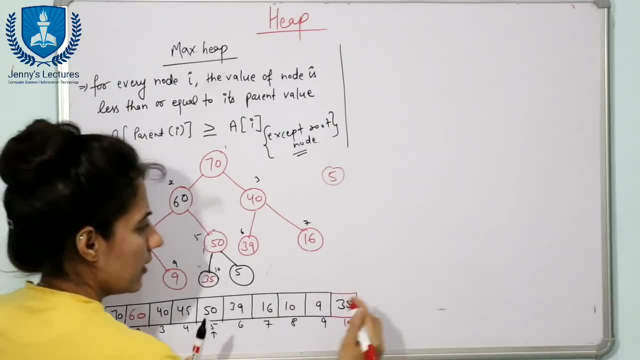 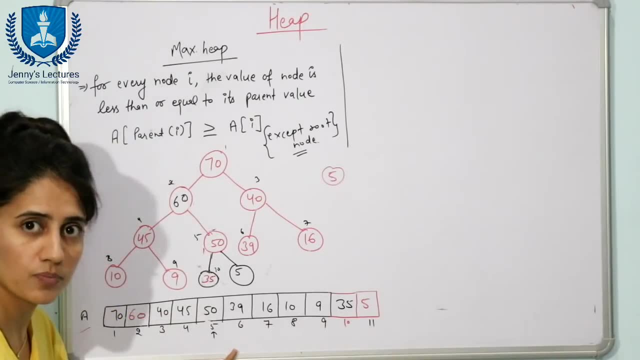 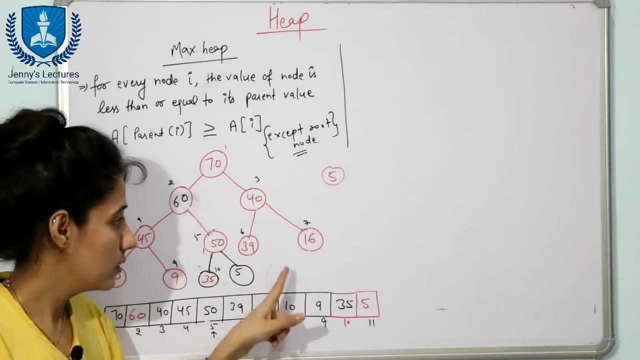 now the 50, sorry 5. now here we are going to increase the size of array and that would be here. we will insert 5 and index is 11th index. now check, we have to check. it is satisfying the maxi property, maxi property or not. now you have to check. after inserting this 5. is this satisfying the maxi property or not? now find out. parent of this node. the index is 11. parent of this node is 50. 50 is greater than 5, so this is satisfying maxi property. no swapping would be done now. in this case, only one comparison is there and no swapping. 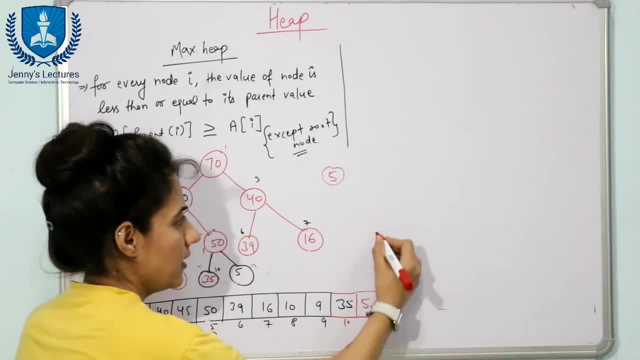 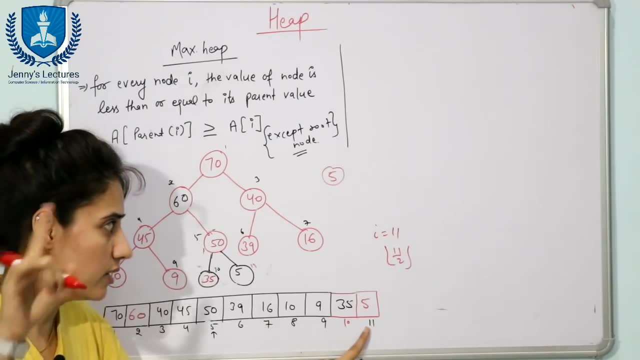 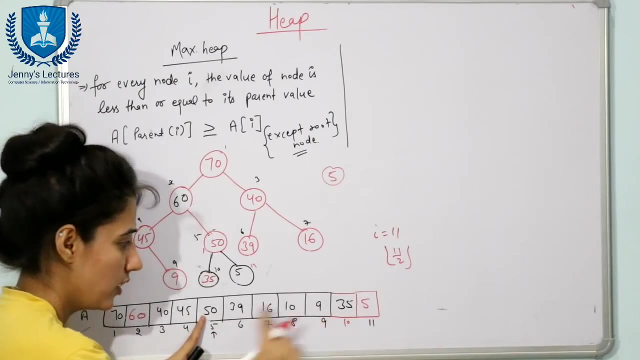 is done. here you can find out. see it is at ith index i is equal to 11, parent of this node. so the parent would be 11 by 2. floor value means 5.5. that is index 5. go to index 5. here we have 50. 50 is parent of 5. it means 50 is parent of 5. 50 is greater than 5. so 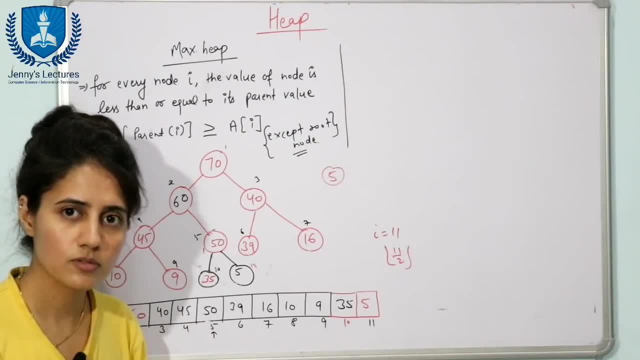 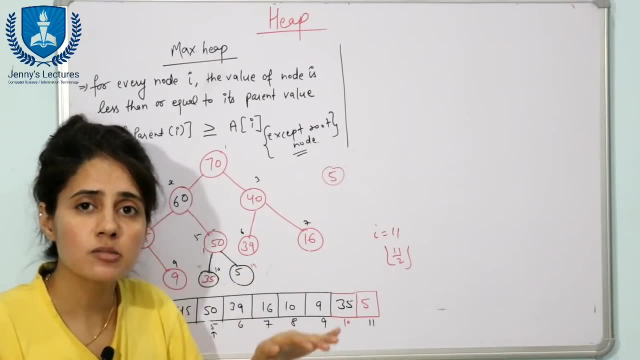 no swapping would be done, so that is done fine. so see, in this case, only one comparison was there, no swapping is done, but maximum, maximum. how many comparisons can be there? previous case like previous case, one is this one, one is this one and one is this one, and 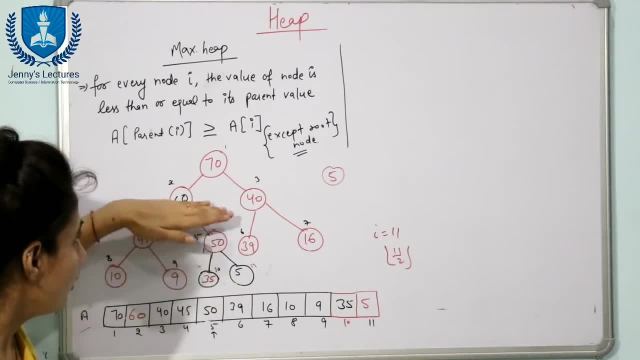 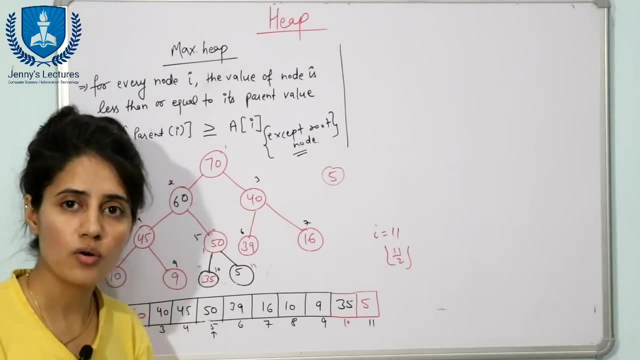 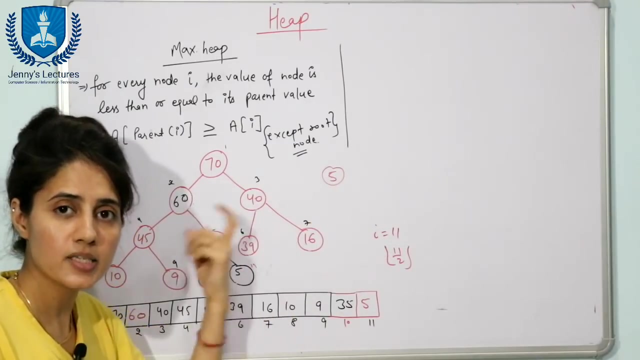 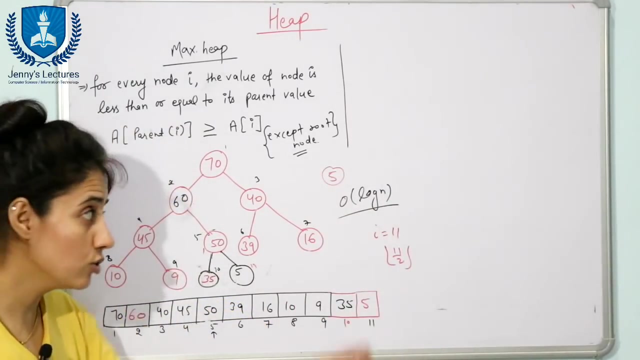 one is this one: how many the according to the height of the tree? fine, and height of a complete binary tree is always log n. so the time complexity, the time taken to insert any element in a max heap is order of log n. insertion operation will take a time order. 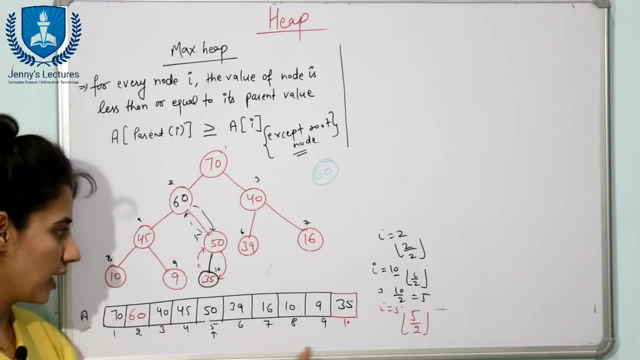 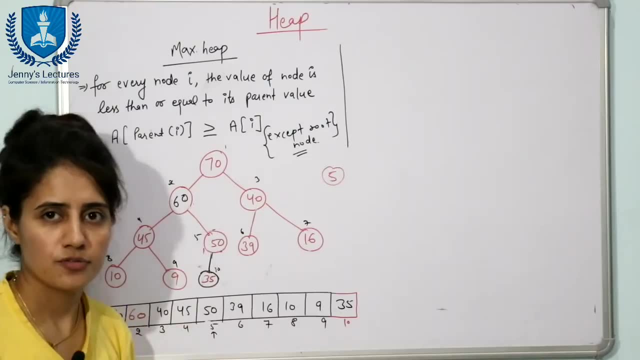 Insertion of 6 days Done After insertion, the array would be something like this And tree would be something like this: Now suppose i want to insert an element having value 5.. Now we cannot insert from root. Simple funda is insert data from the leaf node. 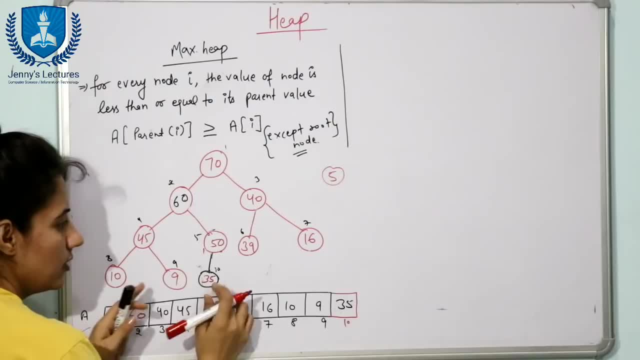 In the tree. Fine, In the leaf node where i can insert, I can insert to the right of 50. Here i can insert 5.. You have to take care of that thing. So, after inserting this 5 in the leaf node, 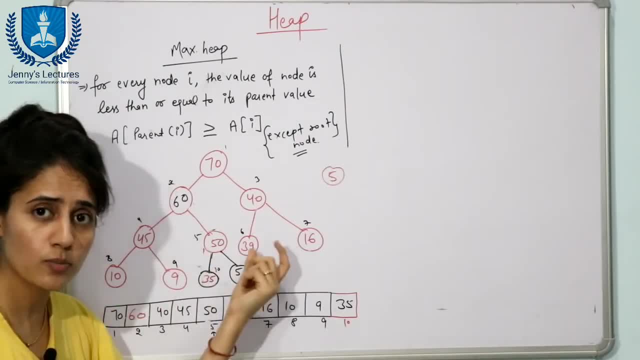 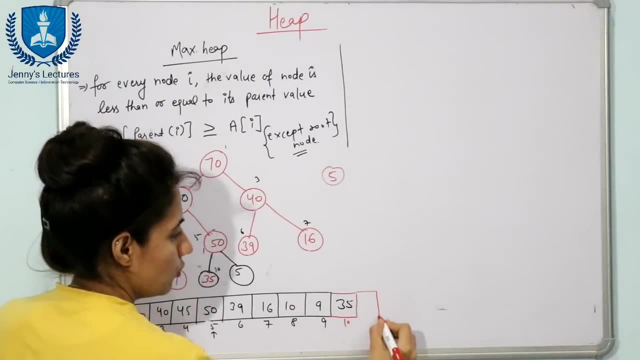 That tree still holds the property of complete binary tree. Fine, Now this 50.. Sorry, 5.. Now here we are going to increase the size of array, And that would be here. we will insert 5 and index is 11th index. 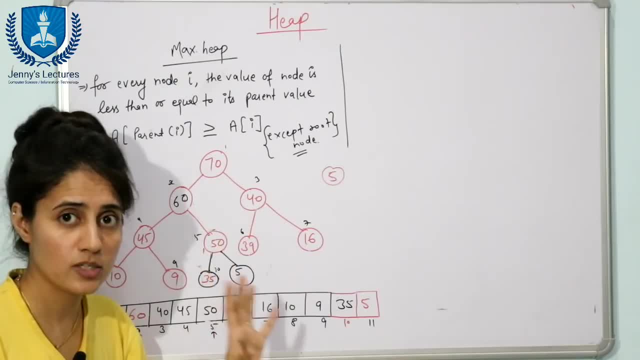 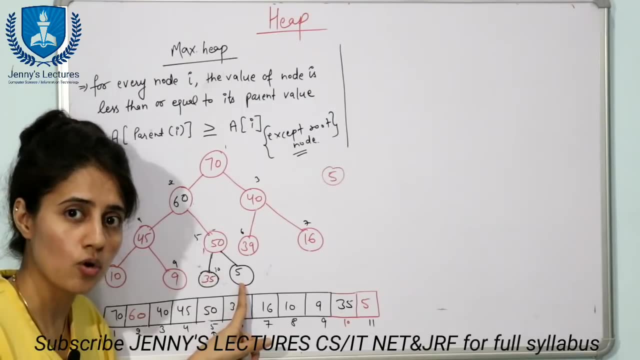 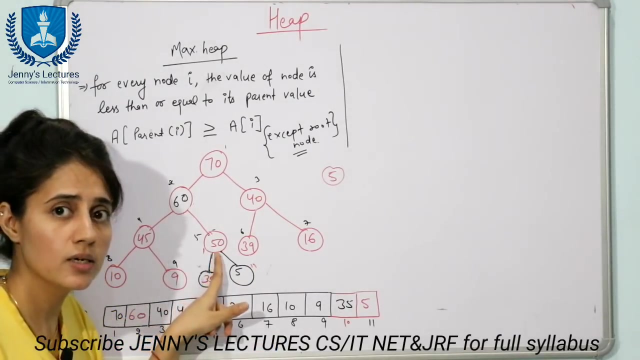 Now check. We have to check. it is satisfying the maxi property or not. Now you have to check. after inserting this 5.. Is this satisfying the maxi property or not? Now find out. parent of this node. The index is 11. parent of this node is 50. 50 is greater than 5.. 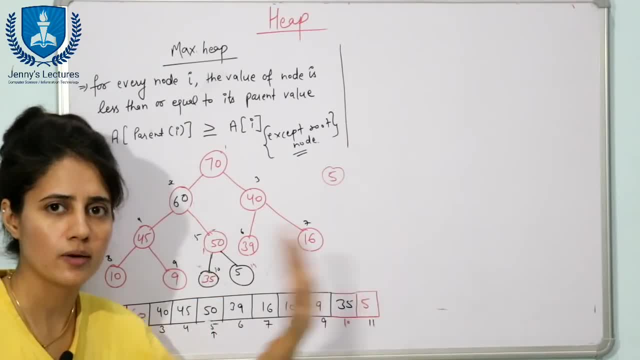 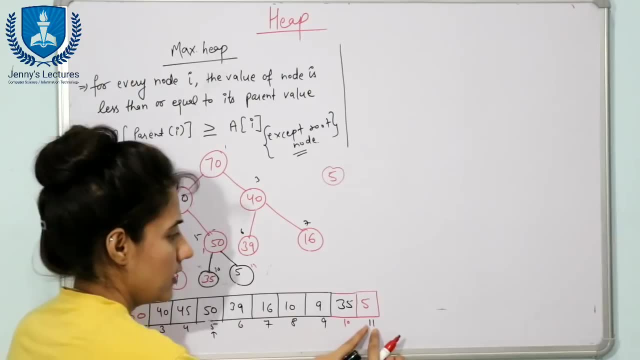 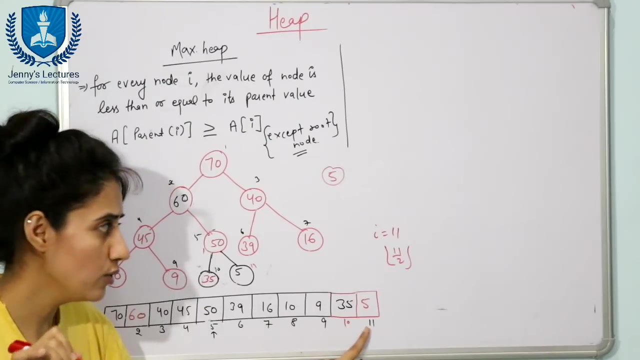 So this is satisfying maxi property. no swapping would be done. Now, in this case, only one comparison is there and no swapping is done. Here you can find out. see it is at ith index i is equal to 11. parent would be 11 by 2. floor value means 5.5. that is index 5. go to index 5. here we have 50.. 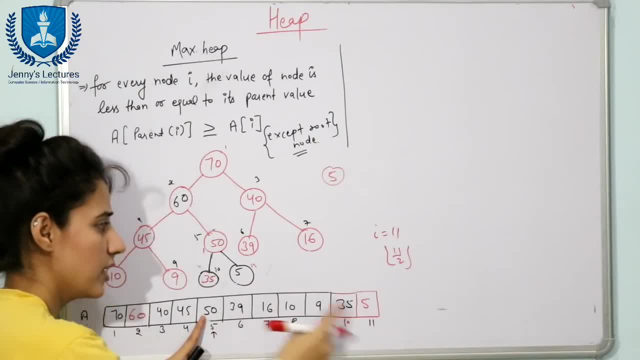 50 is parent of 5, it means 50 is parent of 5, 50 is greater than 5. so no swapping would be done, so that is done, Fine. So see, in this case only one comparison was there. no swapping is done, but maximum, maximum. how many comparisons can be there? 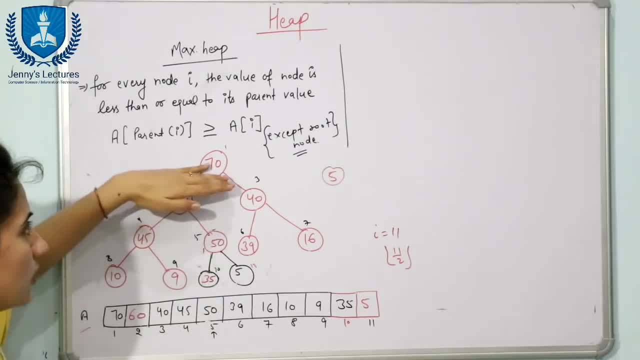 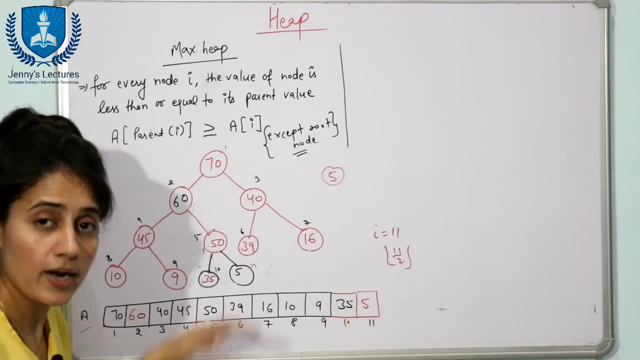 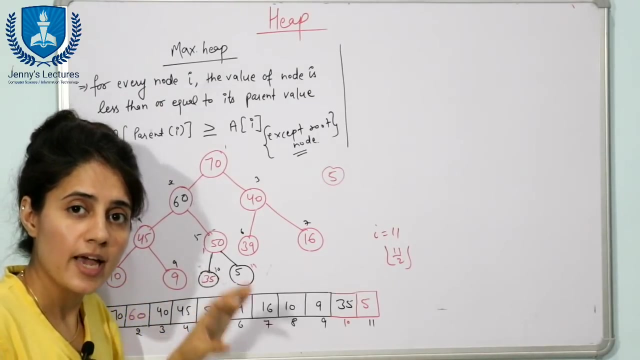 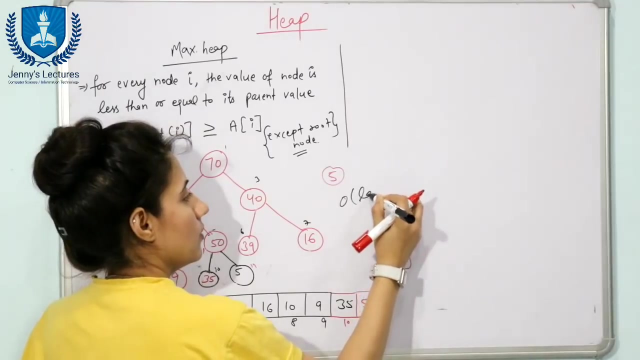 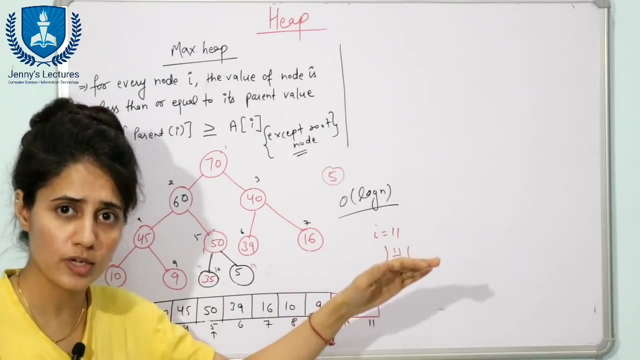 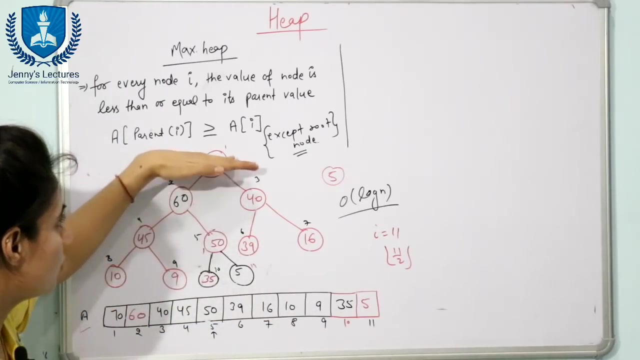 Previous case. like previous case, one is this one, one is this one and one is this one. how many The according to the height of the tree, Fine, And height of a complete binary tree. And height of a complete binary tree is always log n. so the time, complexity, the time taken to insert any element in a max heap is order of log n. insertion operation will take a time. order of log n maximum I am going to take, because in this case only one comparison is there, no swapping is done, but maximum. how many comparisons can be there with this one, with this one and this one, up to the height of the tree? 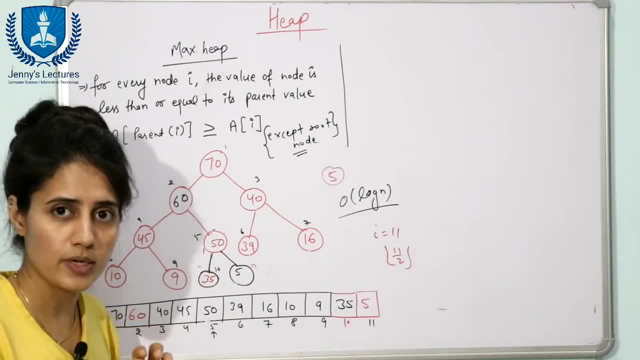 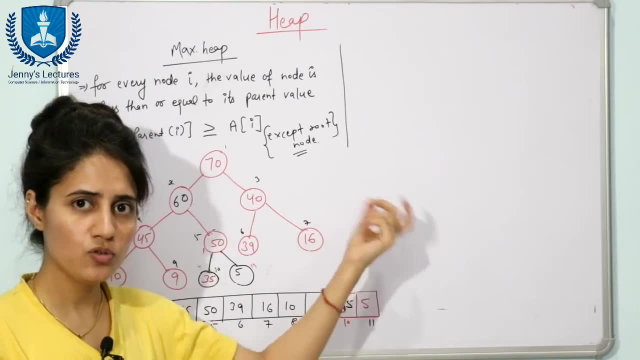 And height is always log n, so order of log n. time would be taken. Fine, this is how we are going to insert a data in max heap. Now I'm going to write, you know, a piece of code for this: insert heap function. see, I'm going to take a function. 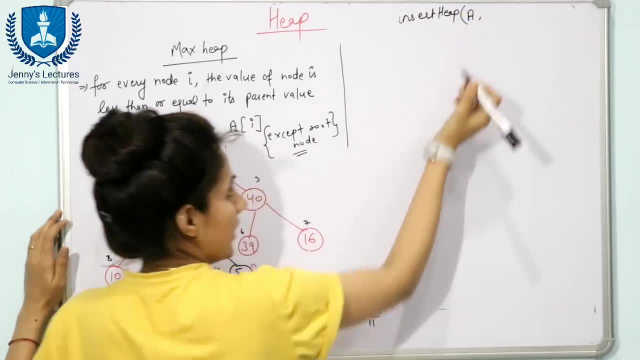 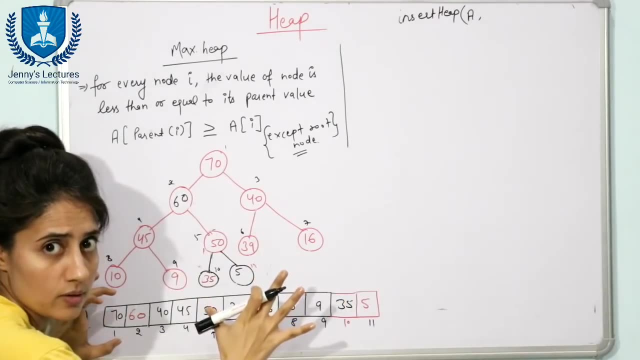 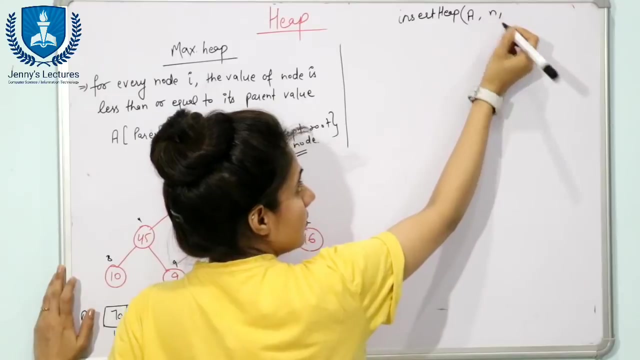 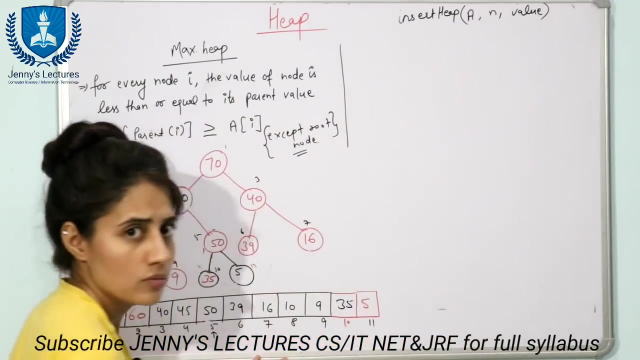 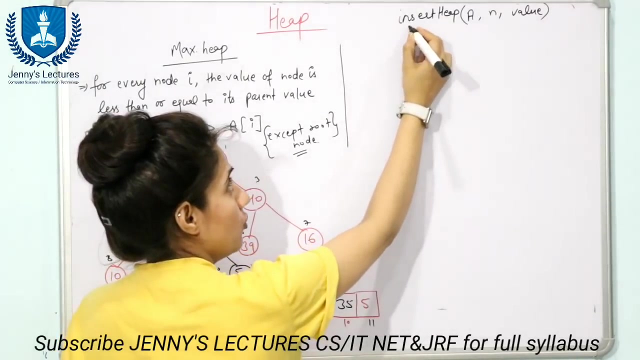 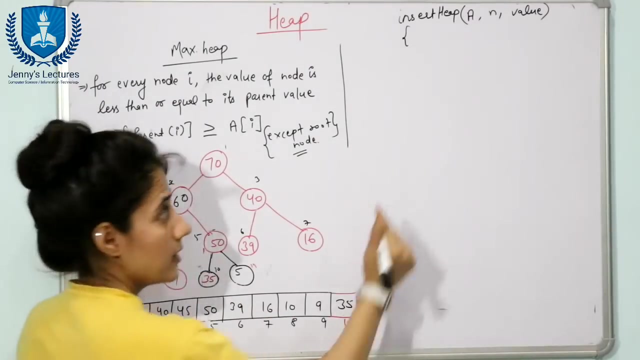 Insert heap. And here I'm going to pass array a, fine, because we are. we are having this representation in our program. we are not having this tree, Fine, so I'm, I'm working with this array only Now. array: total number of elements: n. and next is which value the data you want to insert. you can say value, fine, which value you want to insert? okay, obviously you have to take care of this data type also. here I'm not writing the correct one, I'm just going to tell you the logic. now, next thing is we are going to increase this size means n is equal to n plus 1.. 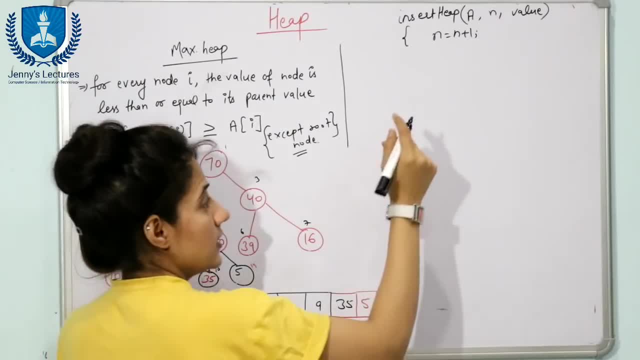 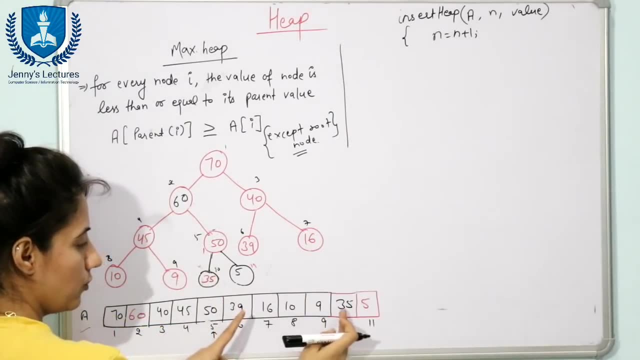 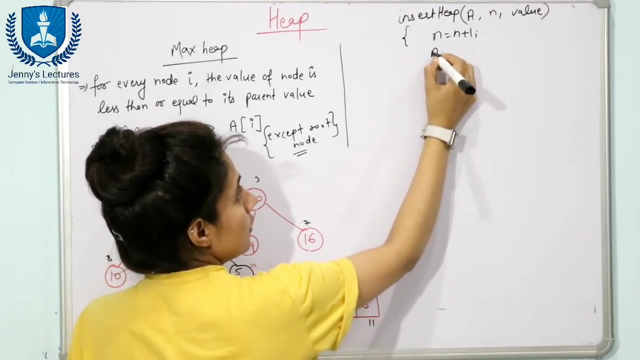 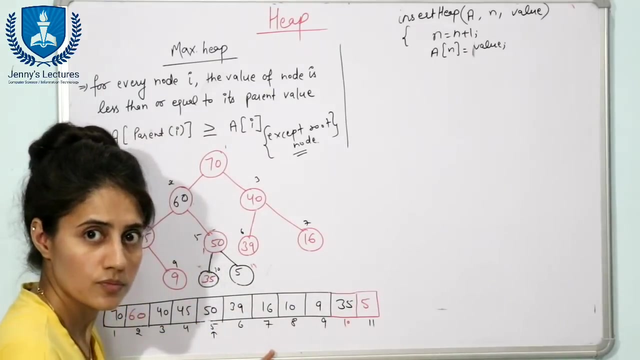 Right Now. next thing is: in the last, in the last free space, we are going to insert that key value, because at starting we are going: we, we have inserted that 60, so we have inserted 60 at this place, fine, so now we are going to insert at array of n, we are going to insert that value, fine, and we are going to take one variable that will point to this side. 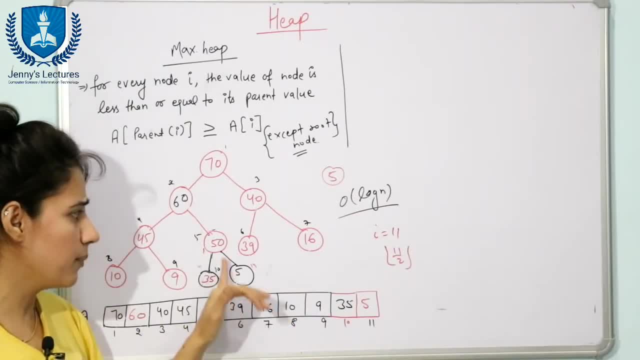 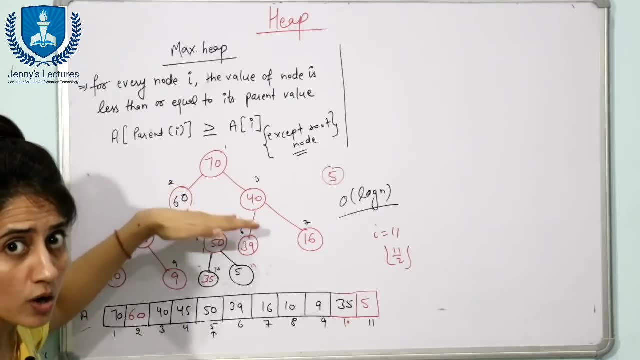 of log n maximum i am going to take, because in this case only one comparison is there, no swapping is done, but maximum. how many comparisons can be there with this one, with this one and this one? up to the height of the tree, and height is always log n. so order. 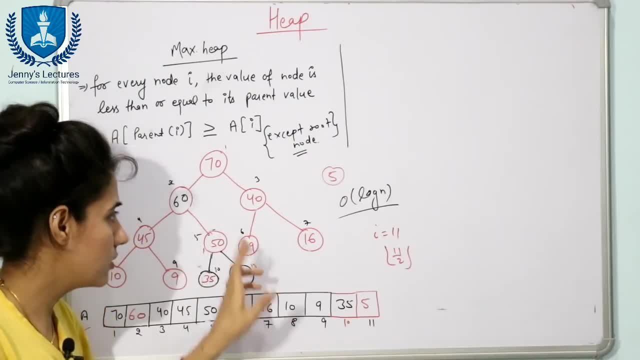 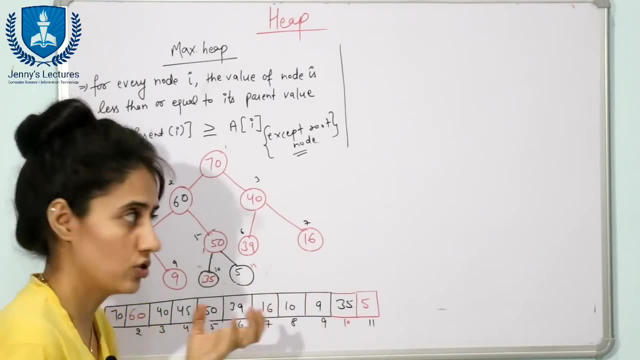 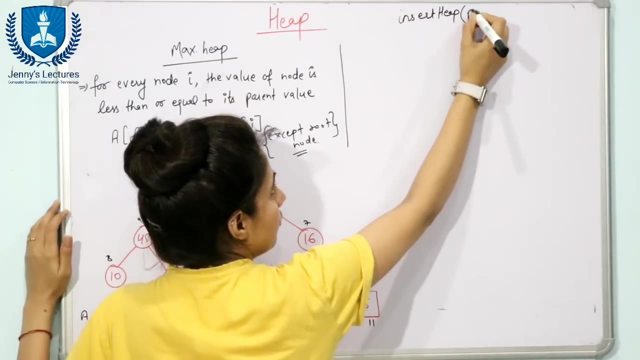 of log n time would be taken. fine, this is how we are going to insert a data in max heap. now i am going to write a- you know a piece of code for this insert heap function. see, i am going to take a function, insert heap, and here i am going to pass array. a fine, so 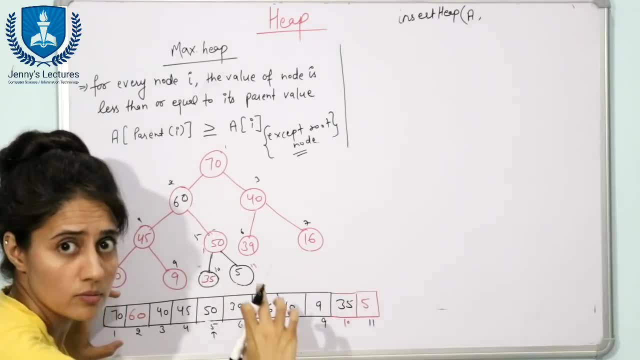 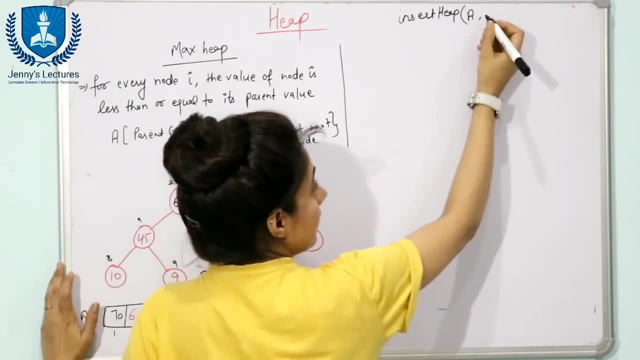 we are going to insert here at t. we are going to leave a value to say that we are going to insert. value is less than value is less than maximum one and领 to be a very reference value. That is the value that i am going to insert. i am going to leave it here by. i am going 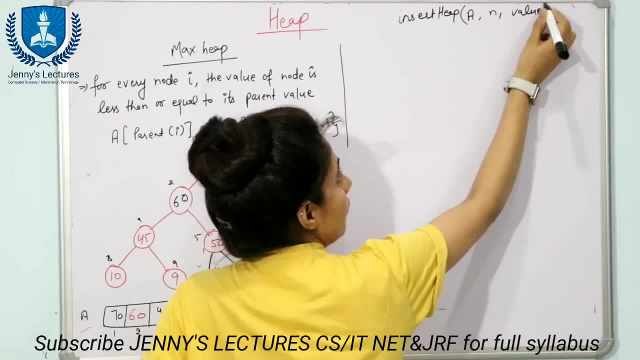 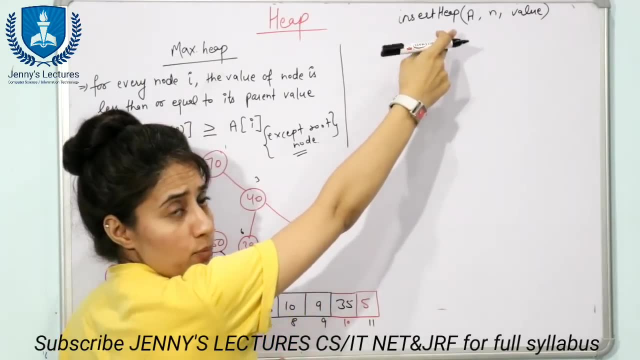 to insert the value of this tree, because we are. we are having this representation in our program. we are not having this tree. fine, so i am. i am working with this array only now. array: total number of elements: n, and next is which value the data you want to insert. 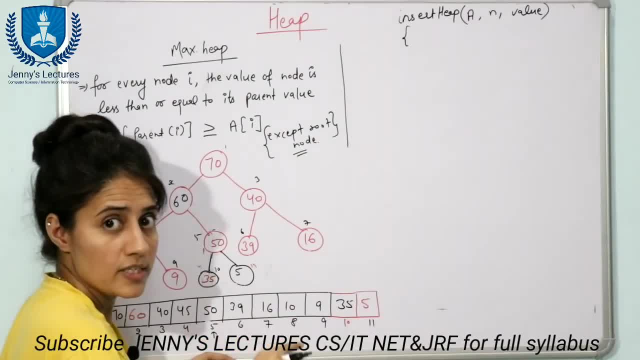 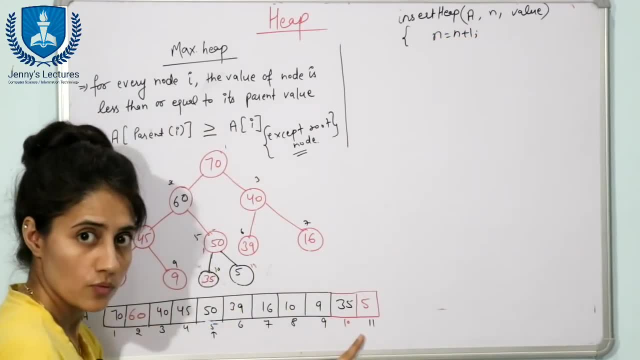 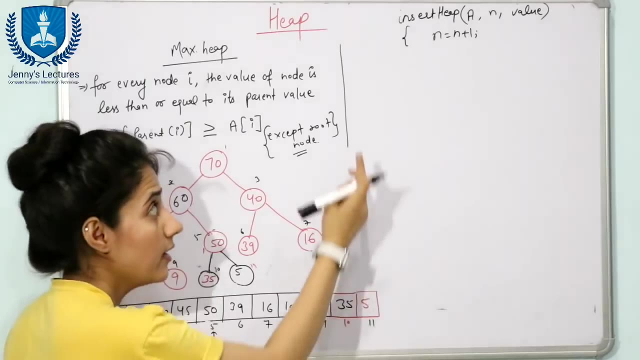 you can say value, fine, which value you want to insert, ok, obviously you have to take care to tell you the logic. now next thing is we are going to increase this size. means n is equal to n plus 1. right now, next thing is: in the last, in the last free space, we are going to insert that. 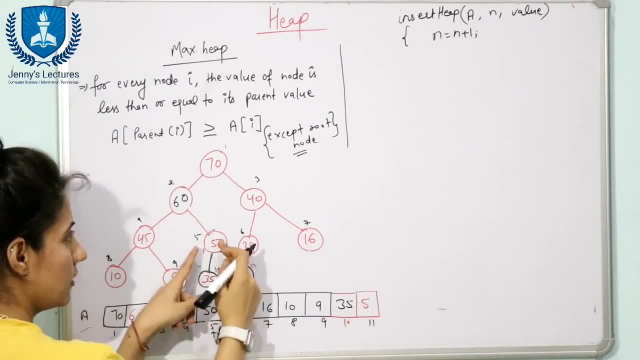 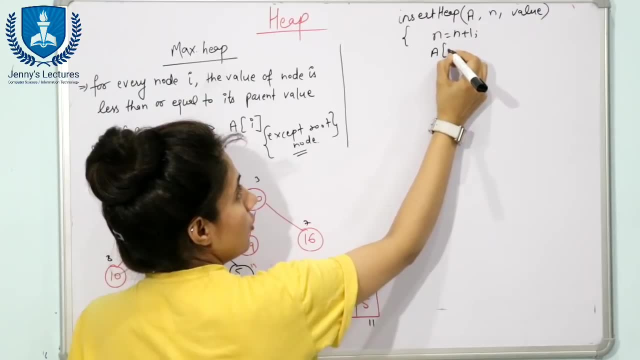 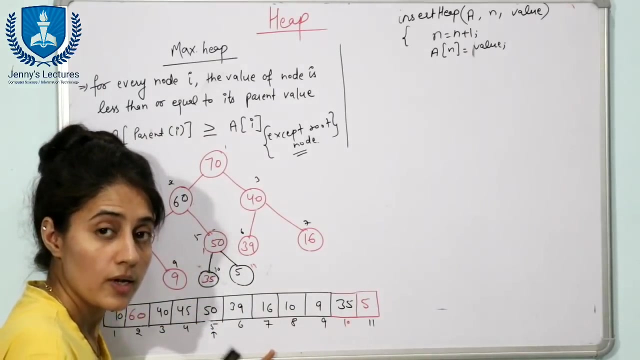 key value, because at starting we are going, we have inserted that 60, so we have inserted 60 at this place, fine, so now we are going to insert, at array of n, we are going to insert that value, fine, and we are going to take one variable that will point to this side, because obviously we are. 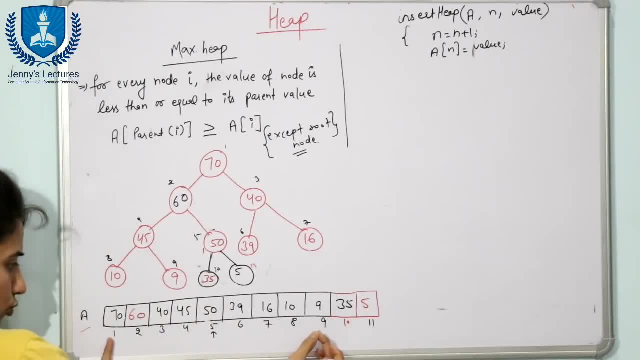 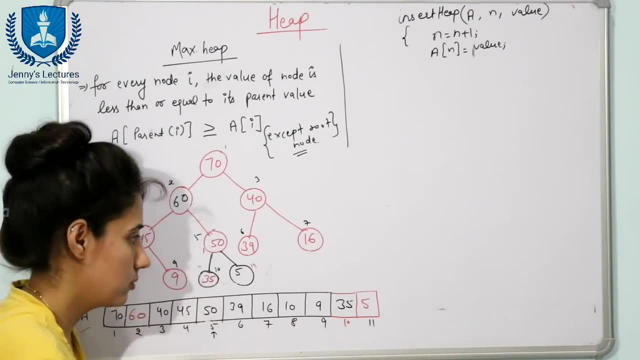 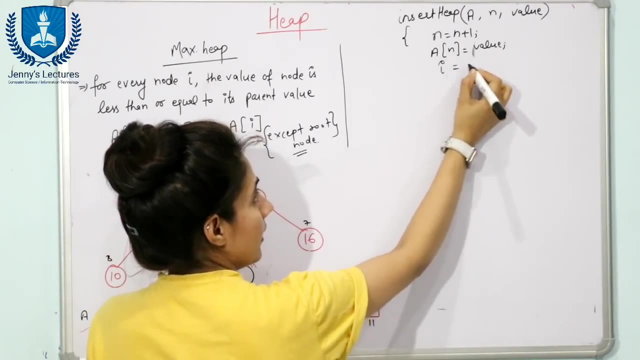 going to compare this with its parent, then again its parent, till we reach to the location 1, so we have to take care of one variable and we are going to, you know, insert a loop here, you, so one variable would be there. suppose i am taking i and i is equal to n. i would be at this place. 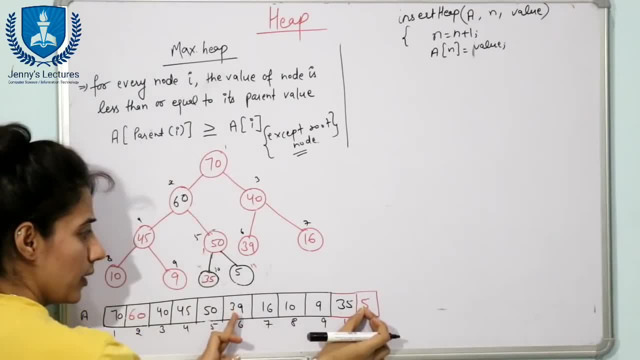 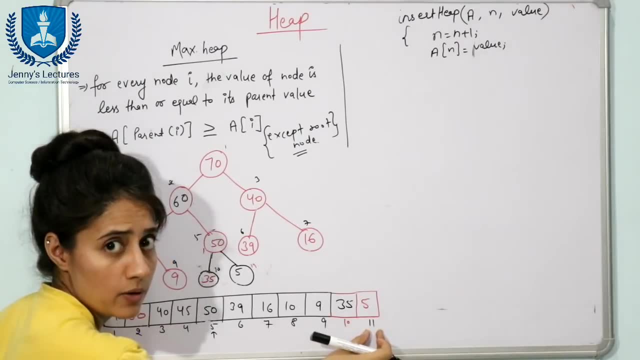 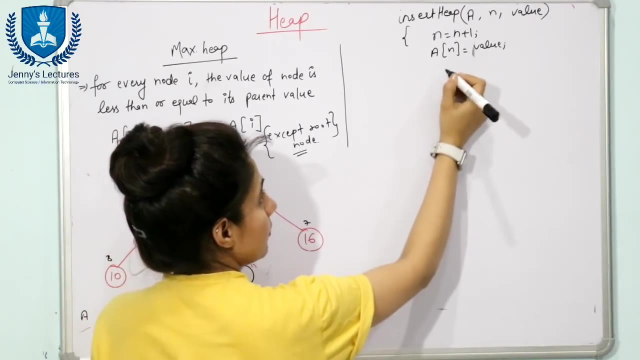 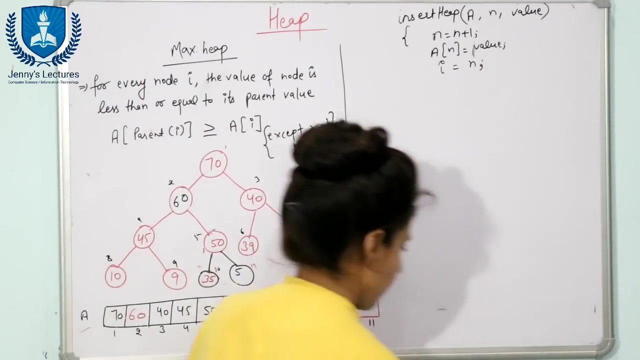 This side, Because obviously we are going to compare this with its parent, then again its parent, till we reach to the location one. so we have to take care of one variable and we are going to, you know, insert a loop here, so one variable would be there. suppose I'm taking I and I is equal to n, I would be at this place, at this place only so, after inserting this five here, 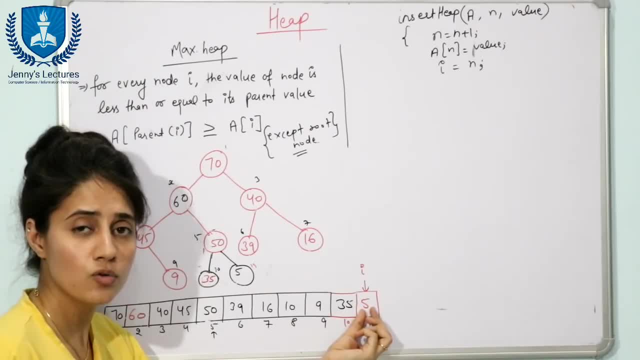 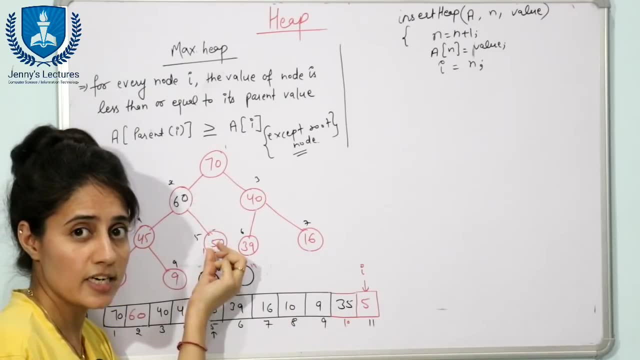 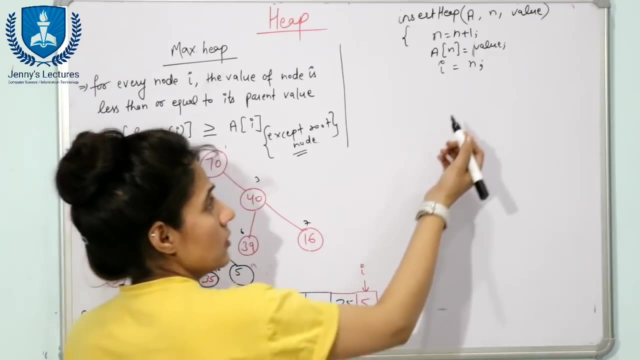 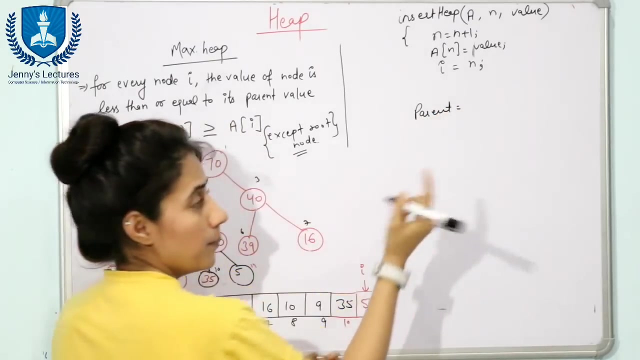 At last, At last, what we have done. we have computed parent value of this five. and why parent value? because we have to compare this value with its parent. is it still satisfying the maxi property or not? is parent is greater than this inserted node or not? fine, so what we have done? so suppose we are going to calculate parent value. now parent, how parent is to be calculated. I divided by two, so now how parent is to be calculated. 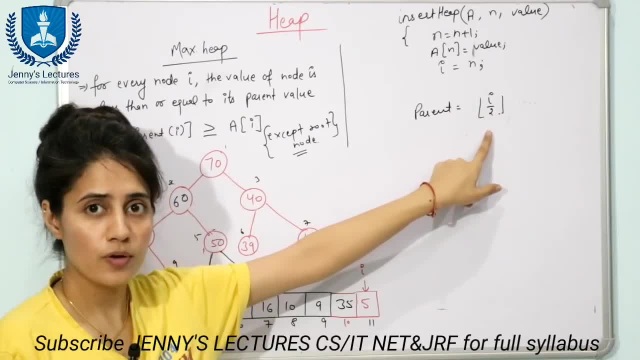 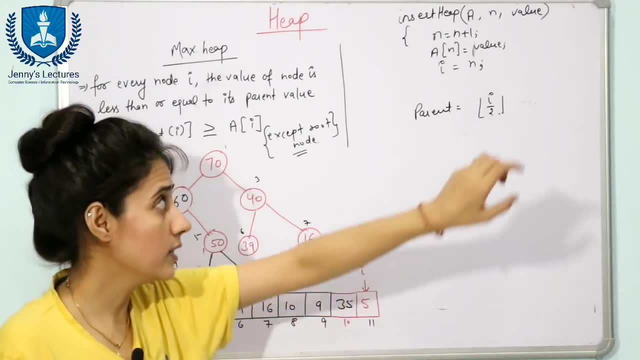 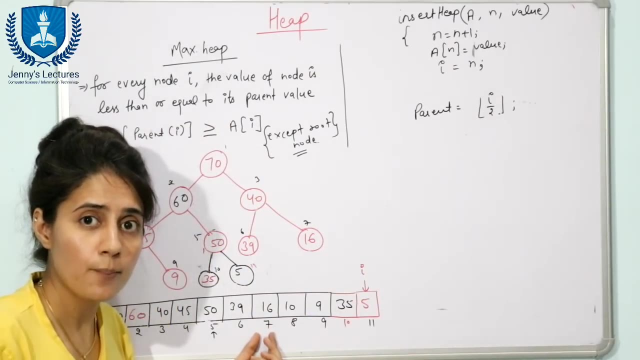 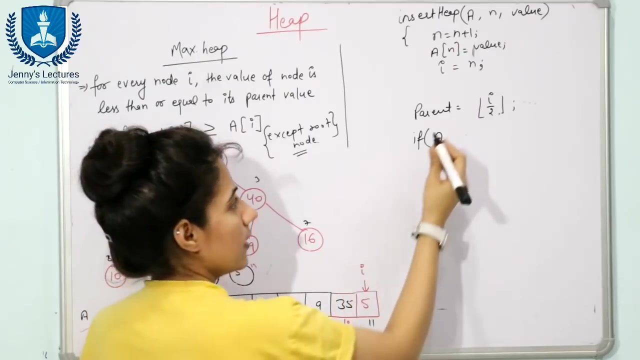 How parent is to be calculated. I divided by two its and its floor value. I simply just write down the that symbol. okay, but when you are going to code this thing, then you will write that floor function. okay, now. next is after calculating parent value. you will compare this with parent. so now you will compare if, if array name is a. 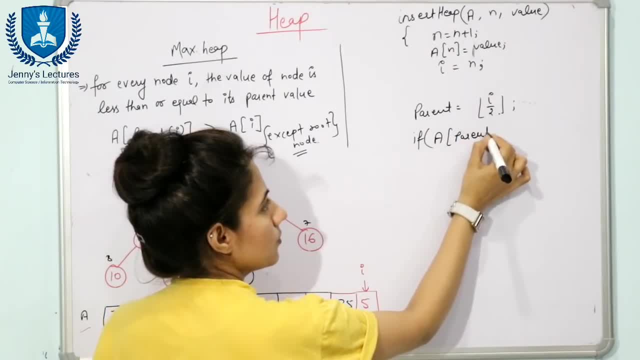 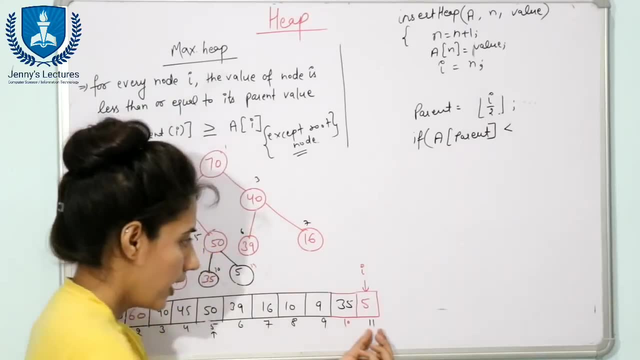 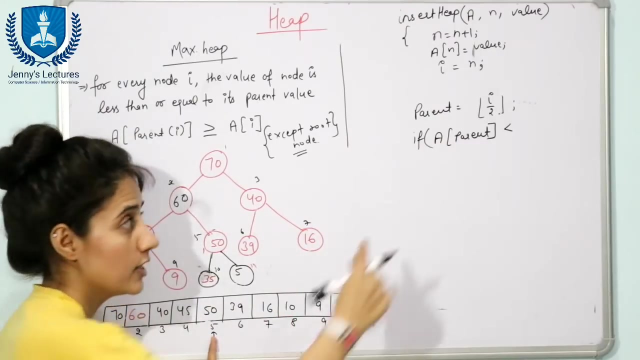 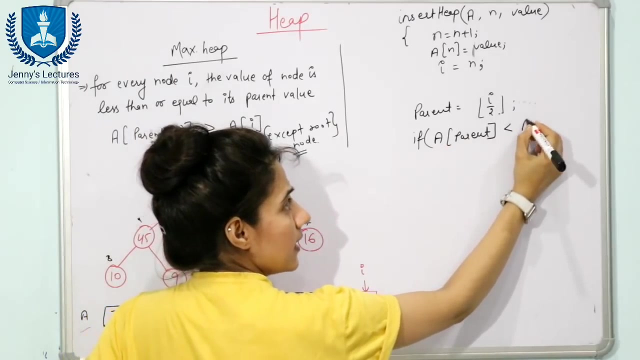 A of This Parent. so now this parent value, parent value, A of parent: I divided by two means I means here eleven. eleven by two floor value, that is five. so in parent we have five. so we will check A of five. A of five is fifty, it means fifty. so here in fifty is less than A of. 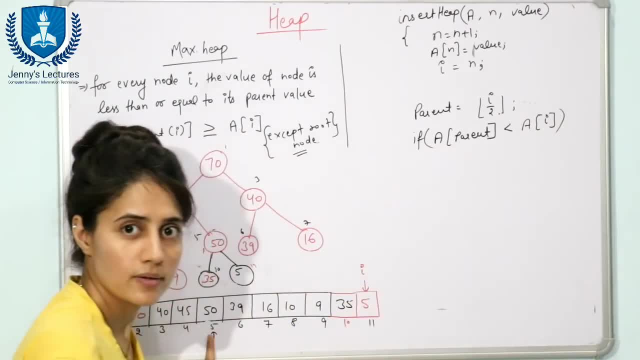 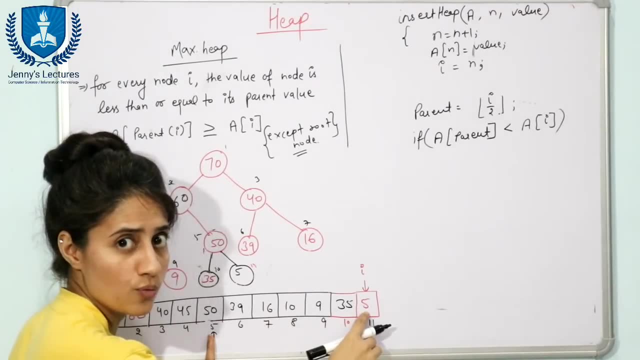 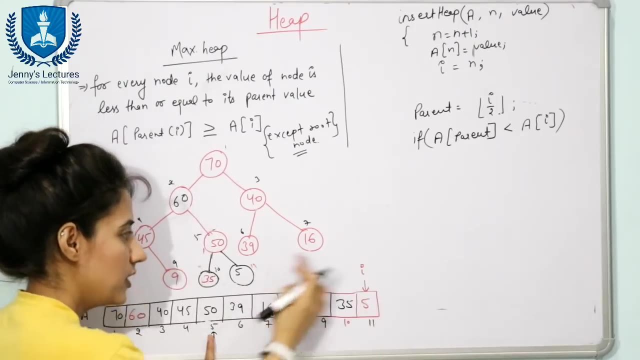 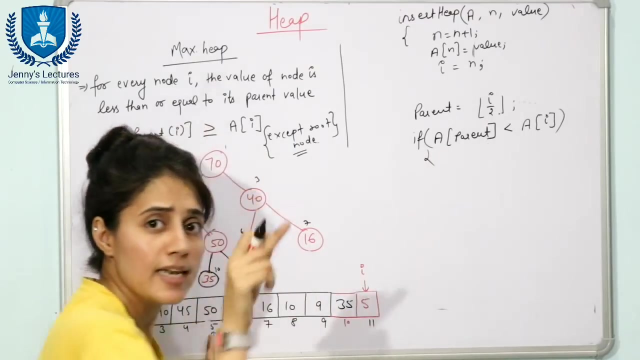 I, I is at this place, fine. so is fifty less than five? So No, Fine, If it would have, it would be less than five. then what? what we will do? we will swap these elements, like we have done when we were inserting sixty. fine, so if this parent is less than the inserted node, then we will do what swapping. 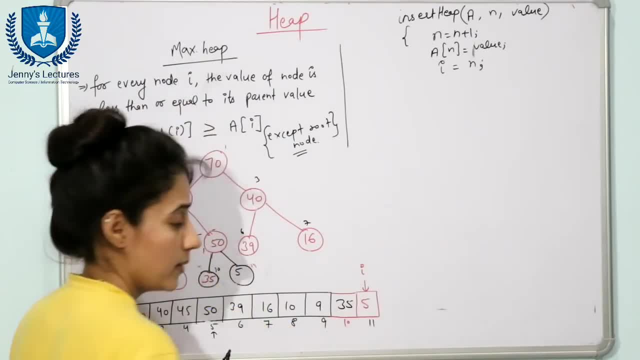 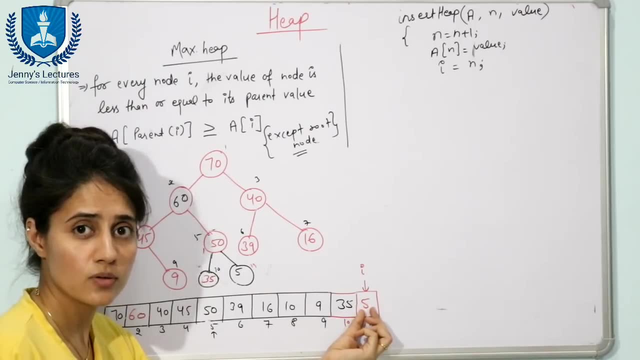 at this place only so, after inserting this 5 here at last, what we have done? we have computed parent value of this 5, and why parent value? because we have to compare this value with its parent. is it still satisfying the max c property or not? is parent is greater than this? 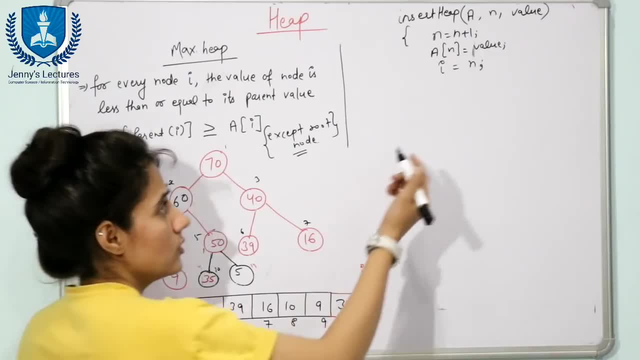 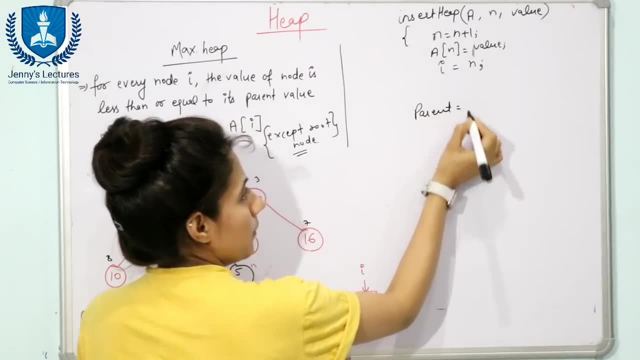 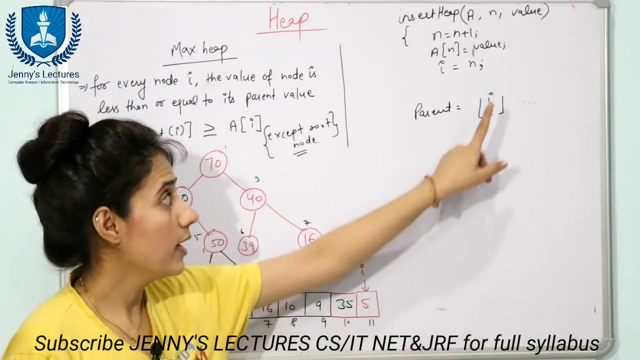 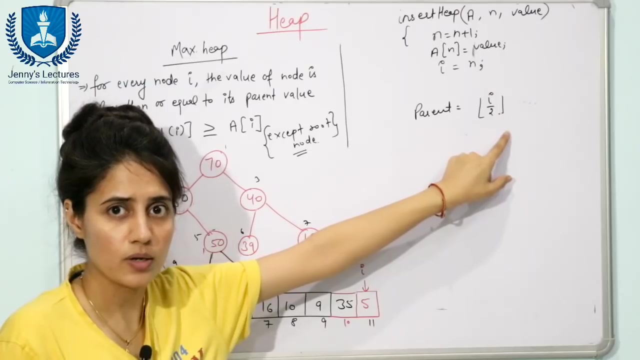 in, in, in, in. we have inserted node or not, fine, so what we have done? so suppose we are going to calculate parent value. now, parent, how parent is to be calculated: i divided by 2. so now how parent is to be calculated, i divided by 2 its and its floor value. so i simply just write down the that symbol. okay, 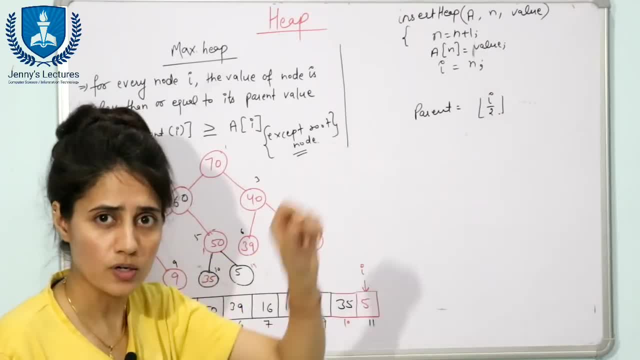 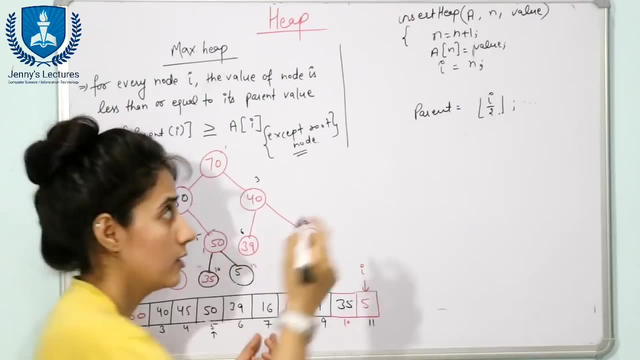 but when you are going to code this thing, then you will write that floor function. okay, now you are going to write down that symbol? okay, but when you are going to code this thing, then you will. next is after calculating parent value. you will compare this with parent. so now you will compare. 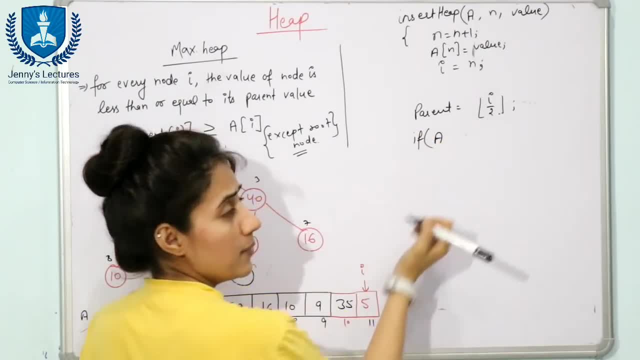 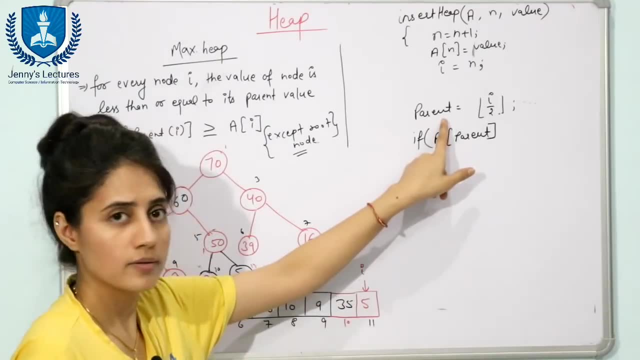 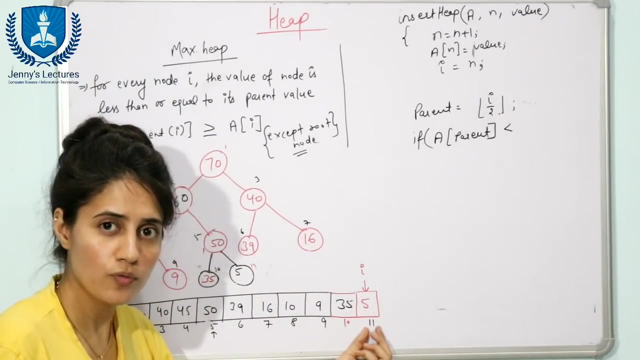 if, if array name is a a of this parent, so now this parent value, parent value a of parent. i divided by 2 means i means here 11, 11 by 2 floor value, that is 5. so in parent we have 5. so we will check a of. 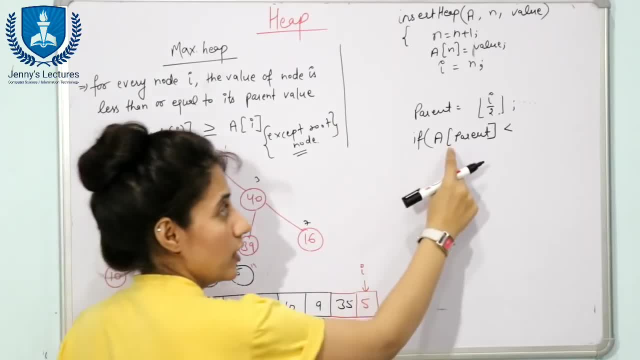 5. a of 5 is 5, so we will check a of 5, so we will check a of 5, so we will check a of 5, so we will. this is 50, it means 50, so here in 50 is less than a of. 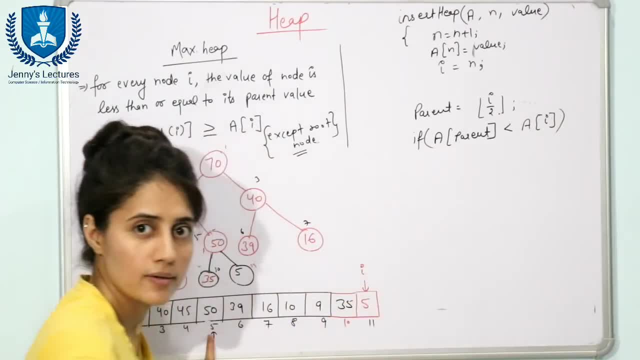 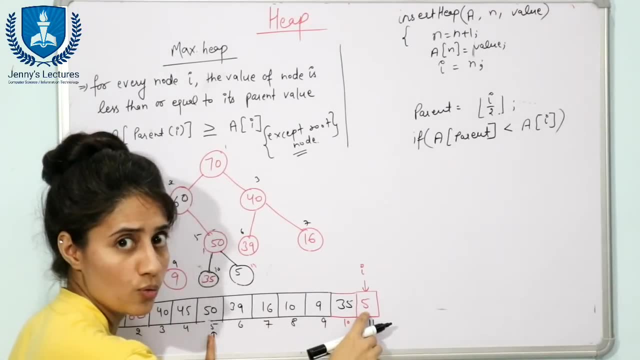 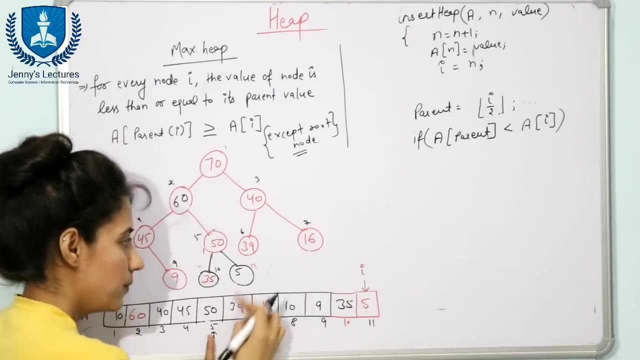 i. i is at this place, fine, so is 50 less than 5? no, fine, if it would have, it would be less than 5. then what will do? will swap these elements, like we have done when we were inserting 60. fine, so if this parent is a of i, then what will do? then? we will swap these elements, like we have done when we 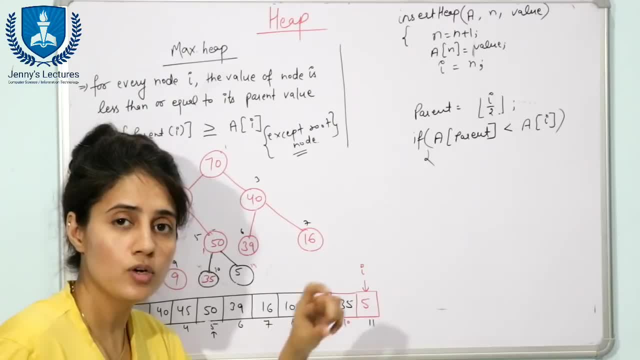 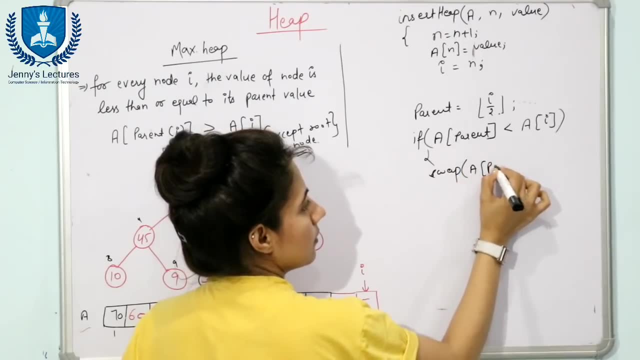 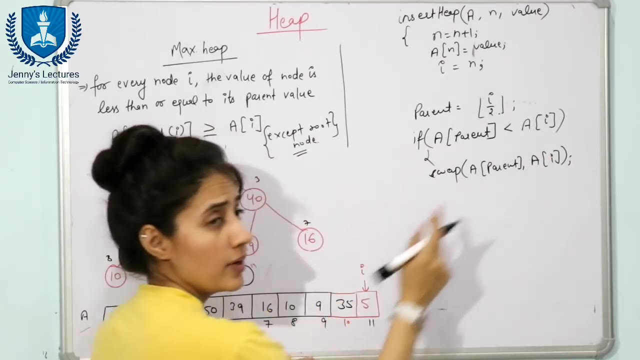 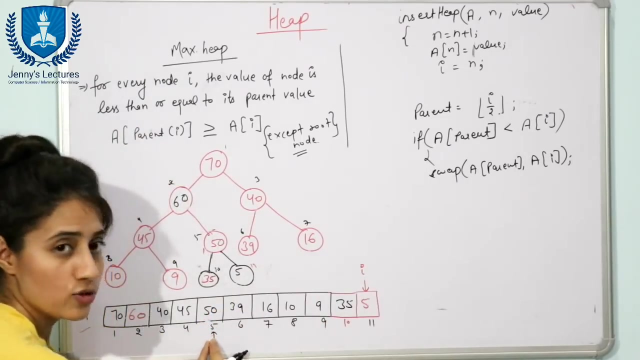 is less than the inserted node, then we will do what swapping. so swap a of parent and a of i, and after swapping, after swapping what we will do, we will move this i also fine, and that i would be at the place of parent now. so i is equal to now that i, i pointer, would 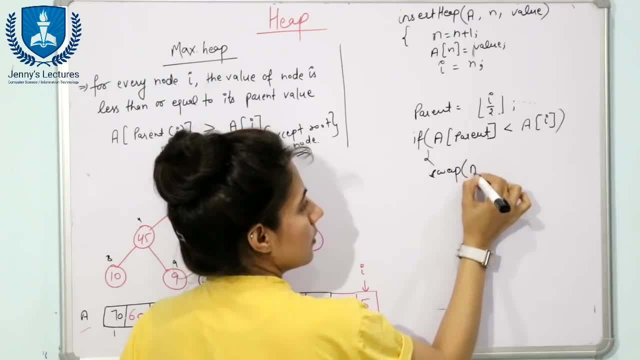 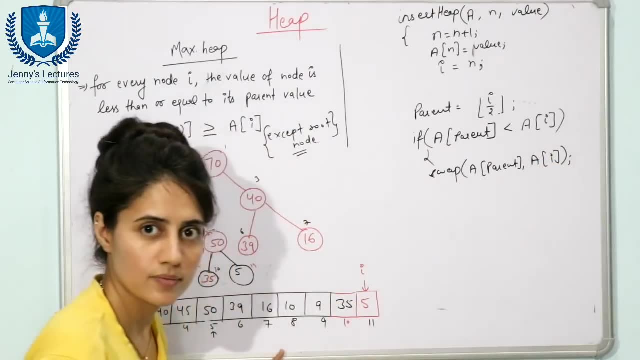 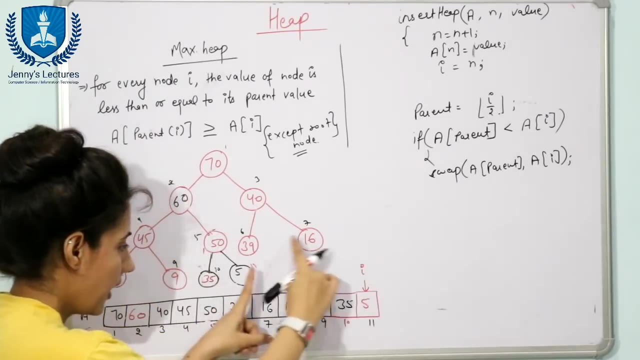 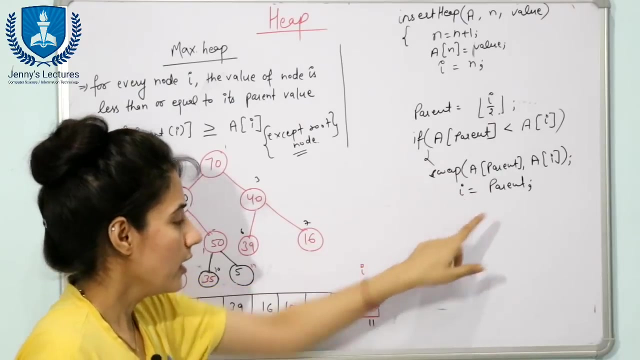 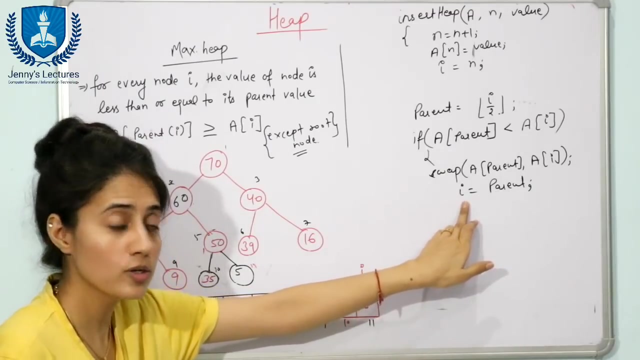 So swap A of parent and A of I, And after swapping, after swapping what we will do, we will move this I also fine, and that I would be at the place of parent now, so I is equal to Now that I- I pointer- would be moved, I value would be moved and that parent value would be at, would be stored in I. why so? because, again, we are going to check with its parent, with parent, till we reach to the root, till we reach to the 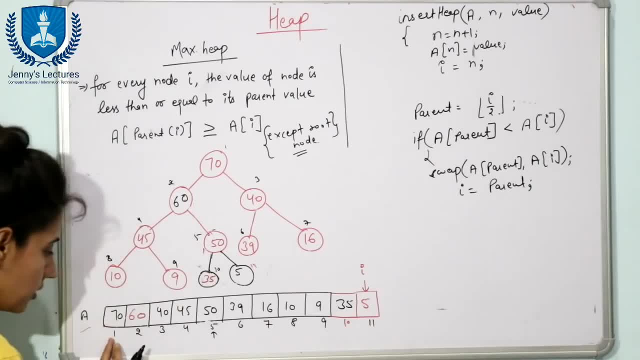 Location: one till we reach I is equal to one. So If this thing thing is true, then swapping would be done. else Else you will do what Return? See, we are going to continue this process until what We reach to this place. 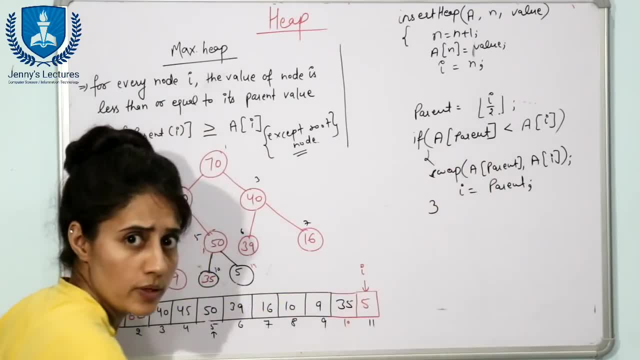 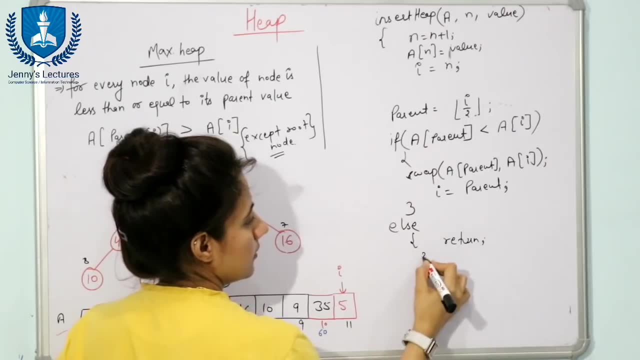 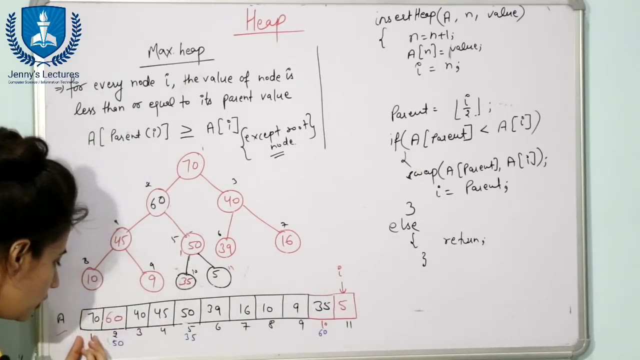 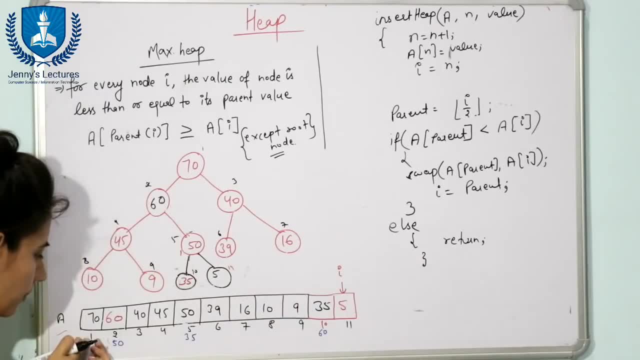 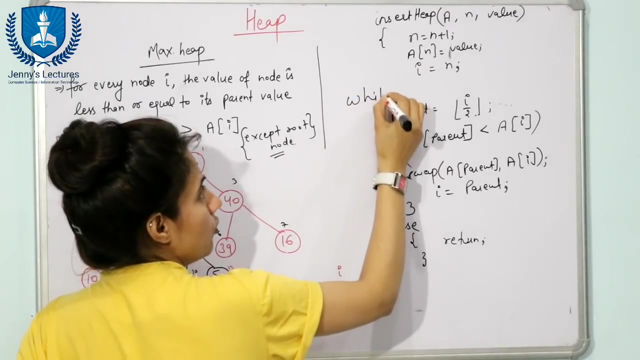 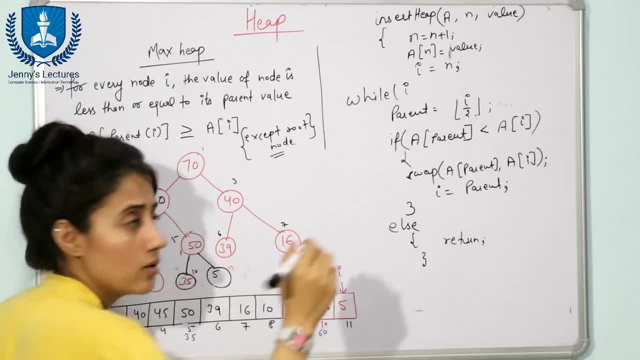 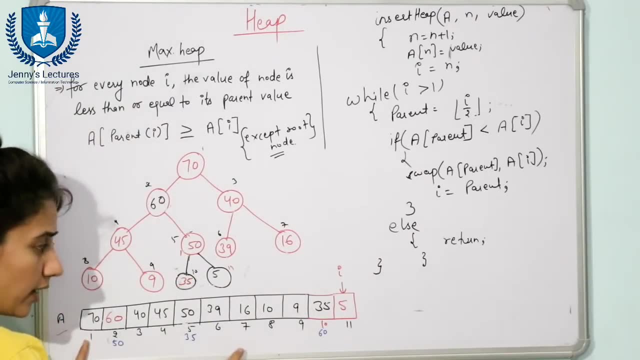 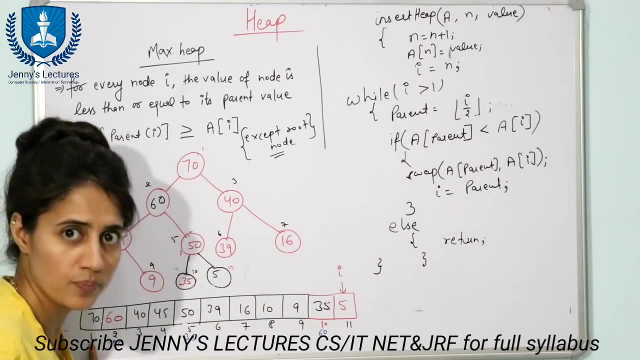 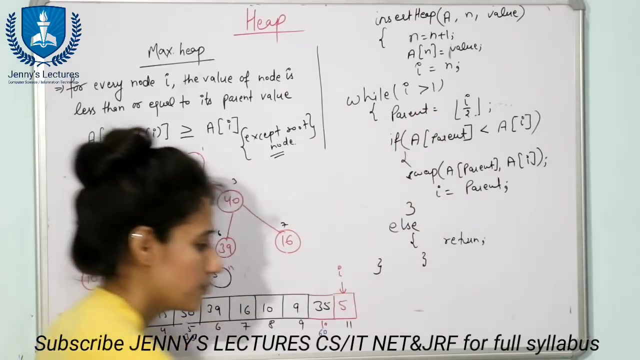 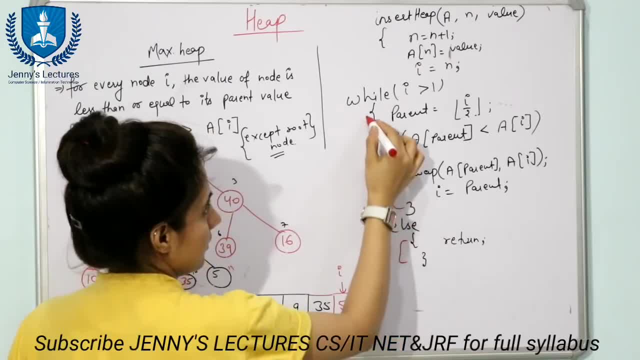 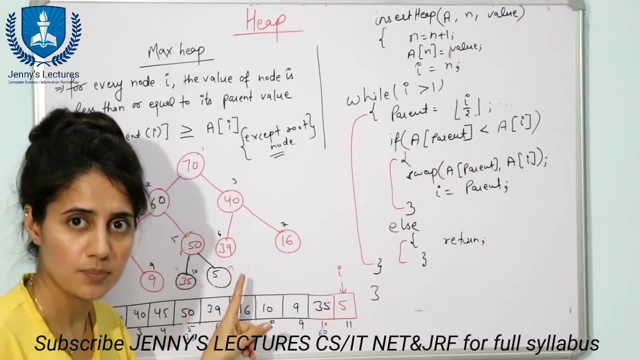 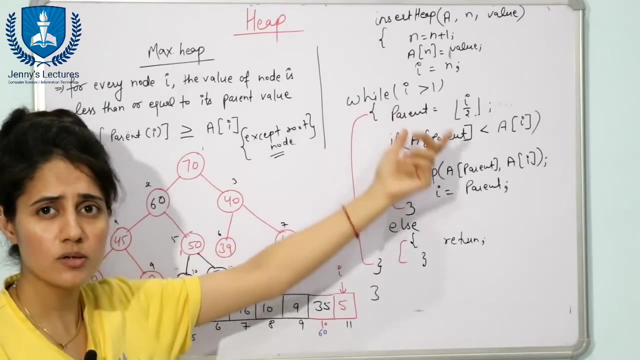 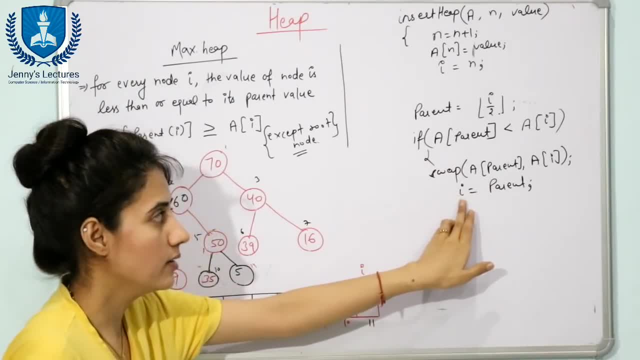 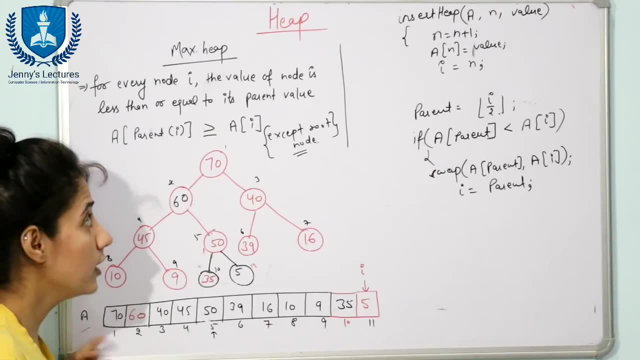 be moved, i value would be moved and that parent value would be at would be stored in i. why so? because, again, we are going to check with its parent, with parent till we reach to the root, till we reach to the location, one till we reach i is equal to one, so 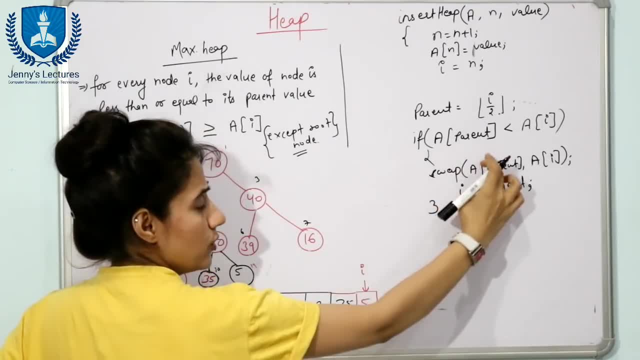 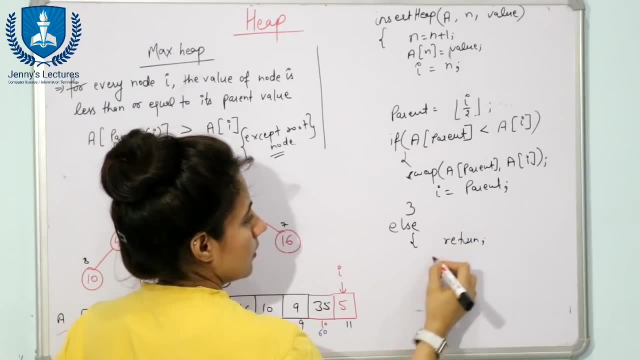 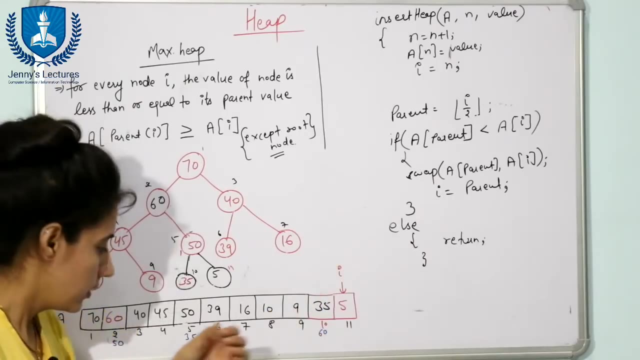 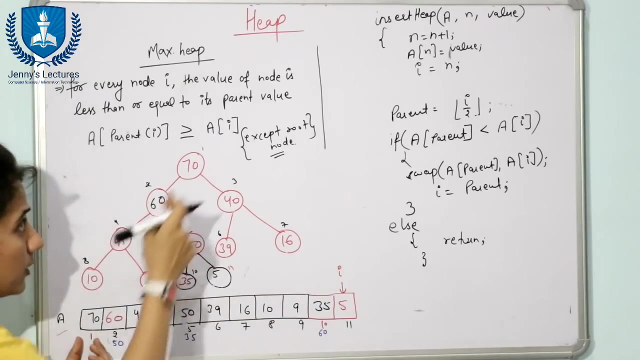 so, so, so. so if this thing thing is true, then swapping would be done, else else you will do what return. see, we are going to continue this process until what we reach to this place. when this i vary, when this i variable- reach to the place one, it means this is the root node. 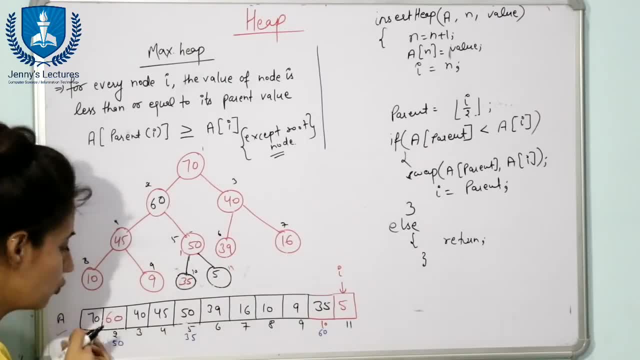 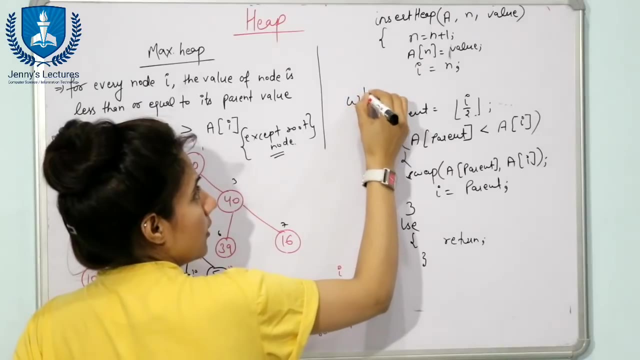 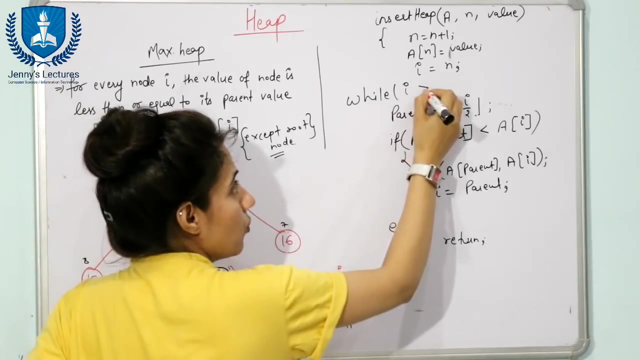 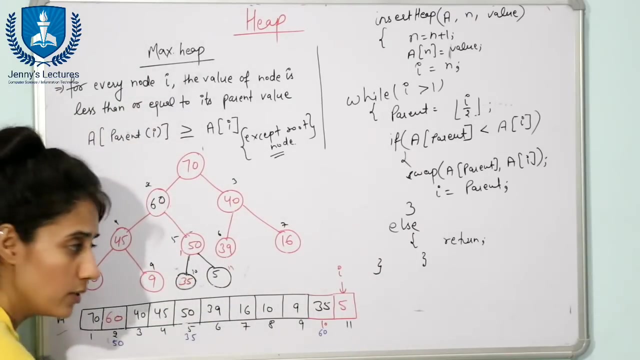 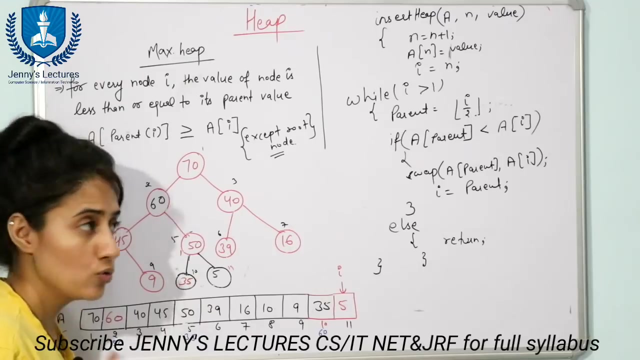 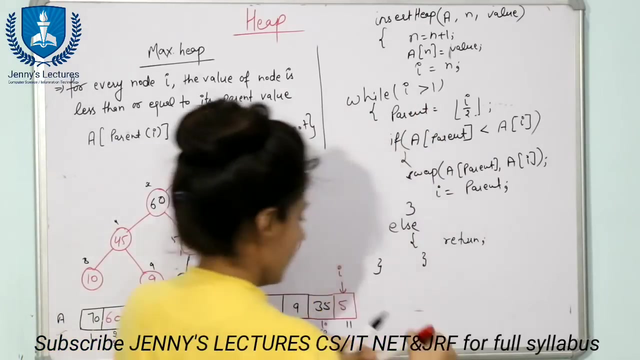 root node is don't having any parent node. so that is why we are not going to find parent node an Flight. and when i reached to 1, it means we have reached to the root node. so you have to stop this thing. so because root is don't having any parent, no need to calculate parent. okay. so now this is if. 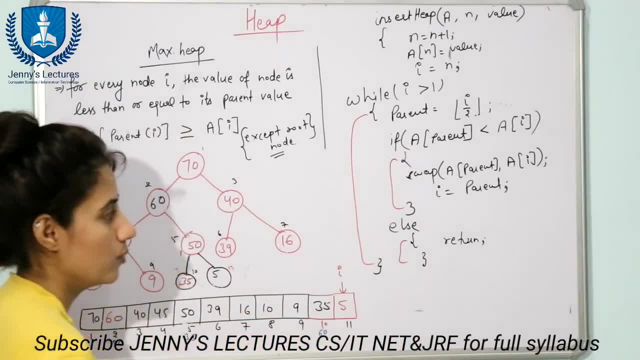 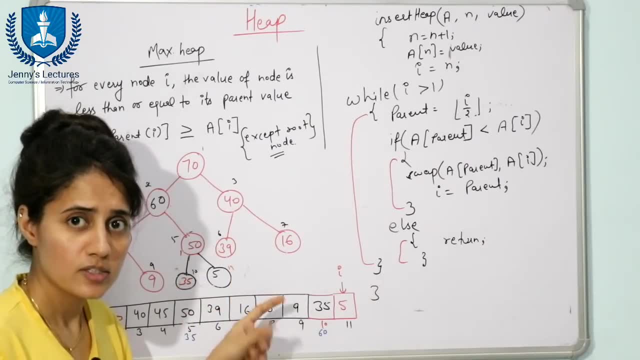 this is your else and this is your while loop. so this is how we are going to implement this insert operation in the max heap. fine, simply, you have to modify a little bit and you can write down how to insert. you can write down insert heap function for a main heap. this condition would 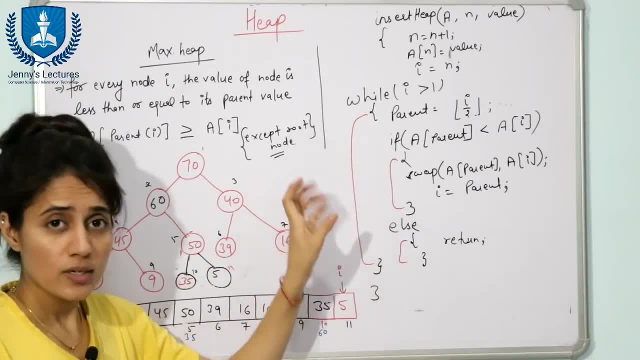 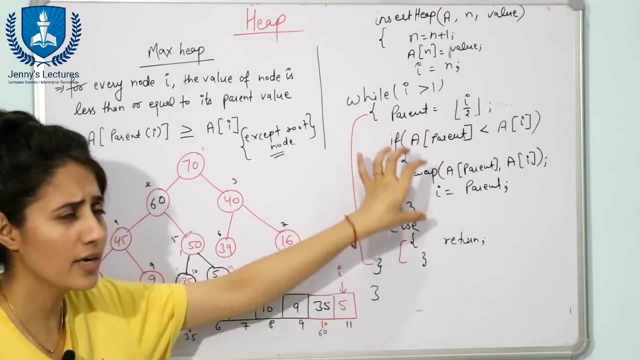 be changed in that case. see, this is. i am not saying that this is the exact code and there there would be no error. obviously there would be some error, but this is how, this is the main logic. this is how you are going to implement this thing. okay, now let's see how the data is to be deleted. 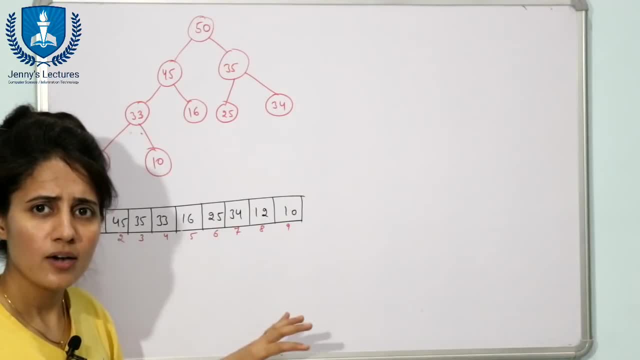 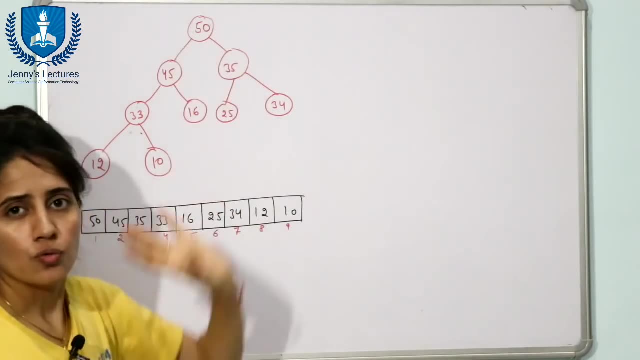 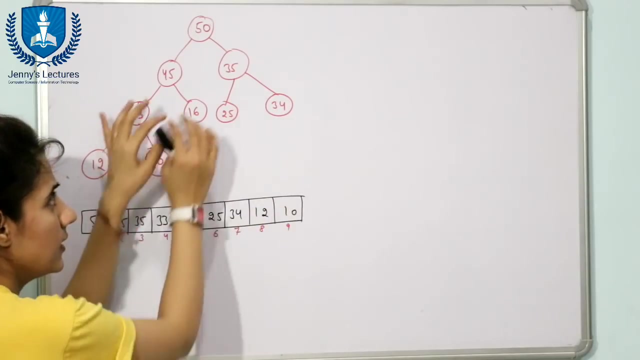 from max heap. so in this case it is not like that you can delete any data like 16, you can delete the 16.. no, you can only delete the root node. that is the condition, that is the rule. fine, so here what you can delete is, if you you want to implement a delete operation in this max heap, then the only 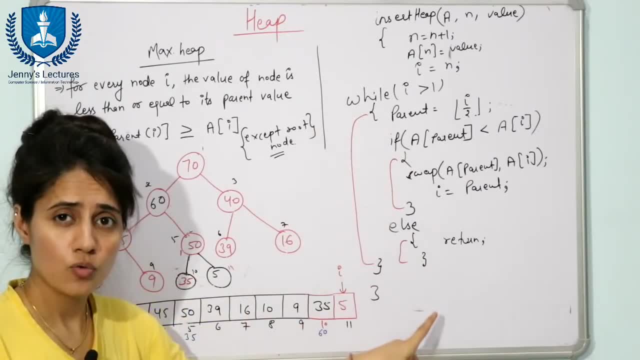 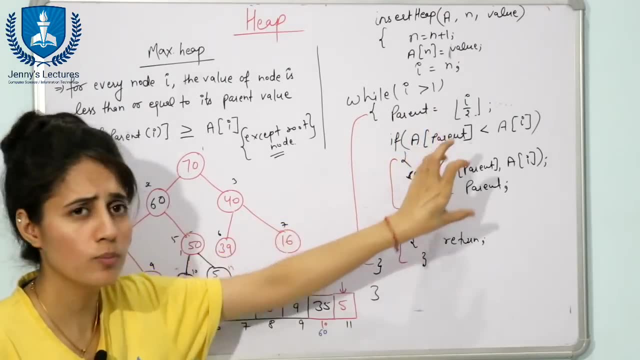 see this is. i am not saying that this is the exact code and there would be no error. obviously there would be some error, but this is how, this is the main logic, this is how you are going to implement this thing. okay, now let's see how the data is to be deleted from max heap. so in this, 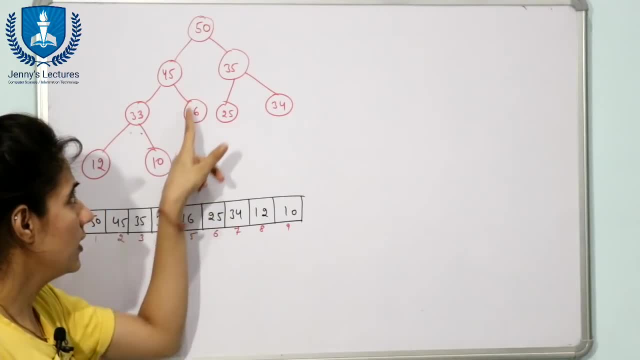 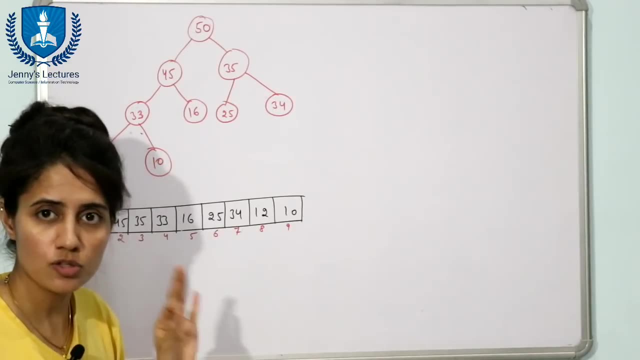 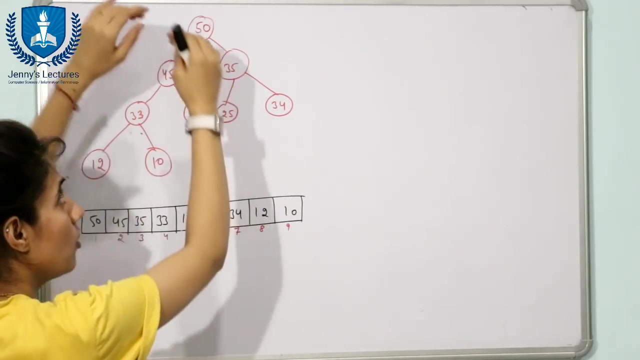 case. it is not like that you can delete any data like 16, you can delete, that's the 16. no, you can only delete the root node. that is the condition, that is the rule. fine, so here, what you can delete is, if you you want to implement a delete operation in this max heap, then the only way is you can. 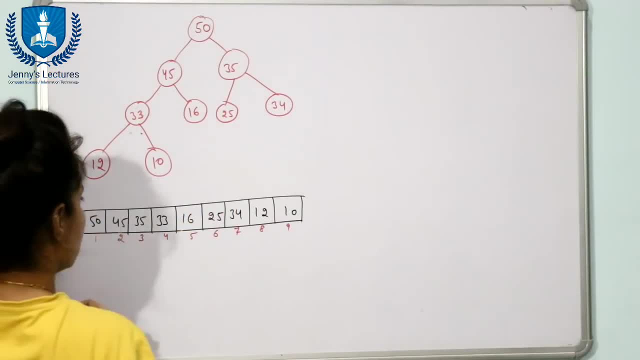 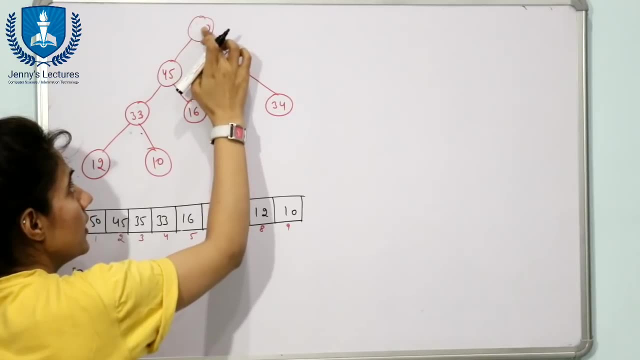 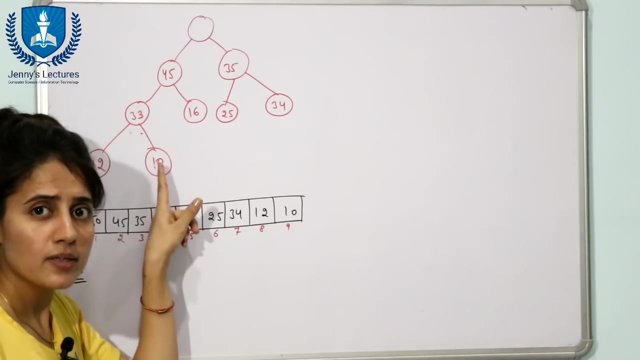 delete this 50 first of all. fine, so suppose you want to implement a delete operation. in this case, you have deleted this 50.. now, at the place of 50, this place is empty. now, what you will do? which data, which data is to be here? so, the last element, the last element, you can say the last. 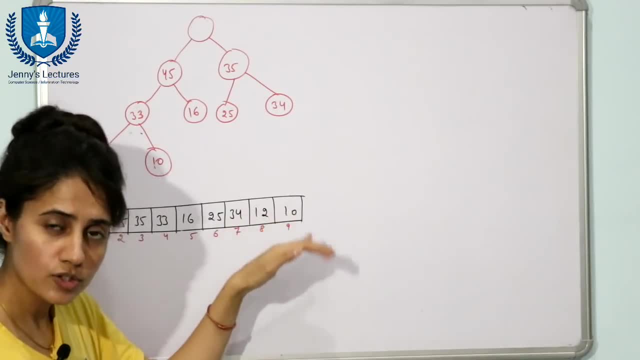 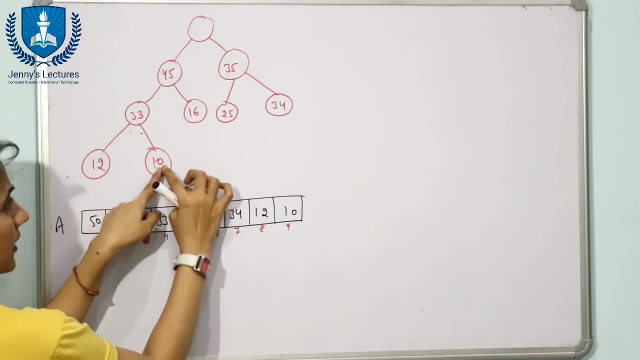 element in the array would be shifted to the root node because we have deleted this root node. so the last in the tree you can see, the last data is what: 10. in the area also, you can see the last is what- 10. so here what you will do this: 10, 10 would be deleted from here and 10 would be. 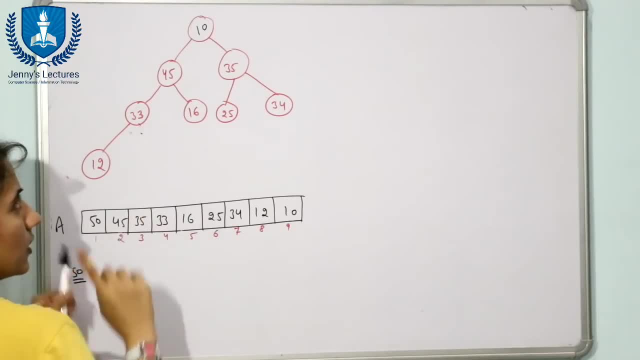 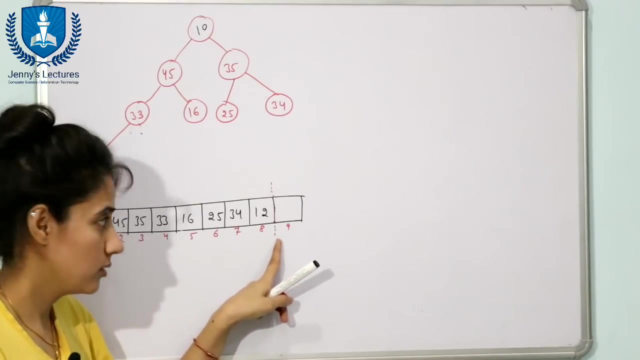 inserted at the place of root. now this is our heap. so in this case also, we have deleted this 10 from here and we have inserted 10 here. only here is now 10. now heap is up to this point: n minus 1 at starting. n is what, 9 now, n is what. 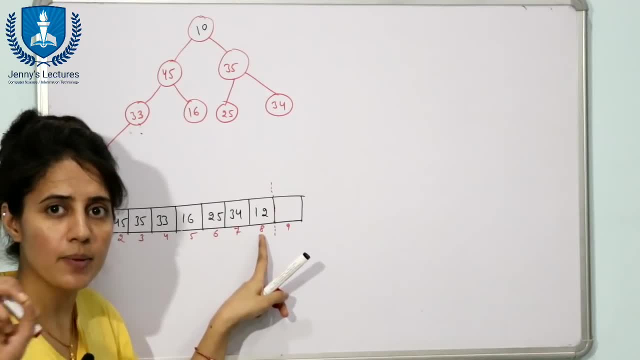 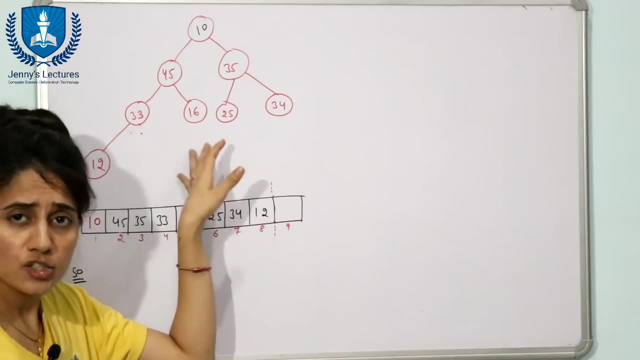 after one deletion: n is what 8. so heap is now till n minus 1. one size has been reduced now see, now you have to check after deletion: is it still satisfying the maxi property? it is not like that you have deleted 50 and you are done with with the deletion. no. 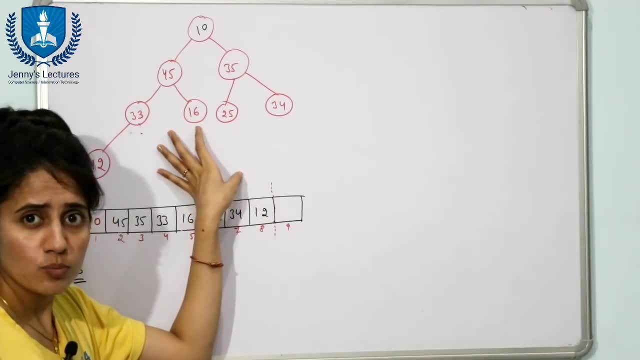 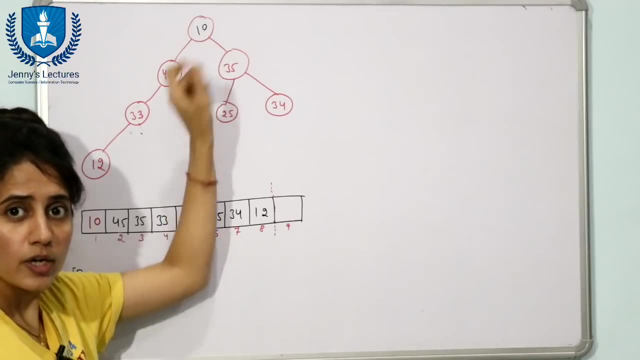 you have to check after deletion: is it still satisfying the maxi property? it is not like you have to check this is satisfying maxi property or not. how you will check. now we have, we have, uh, we have shifted the last node to the root node. now you have to check, you have to. 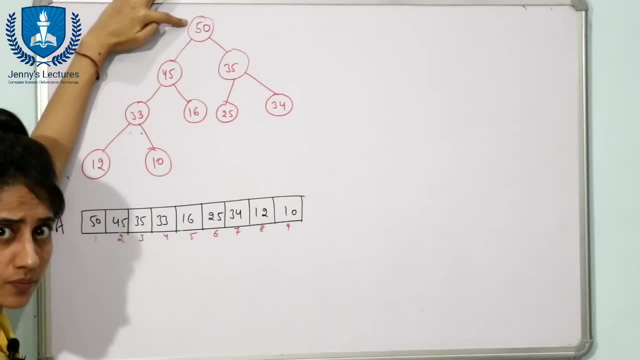 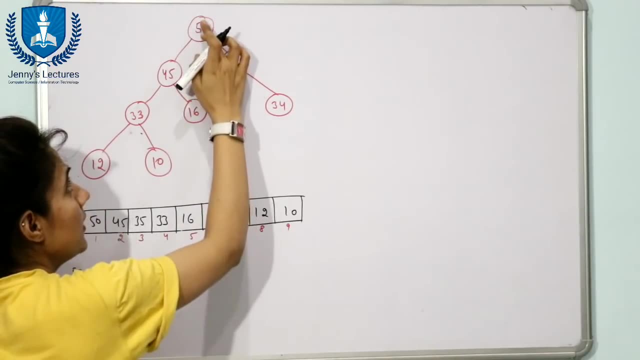 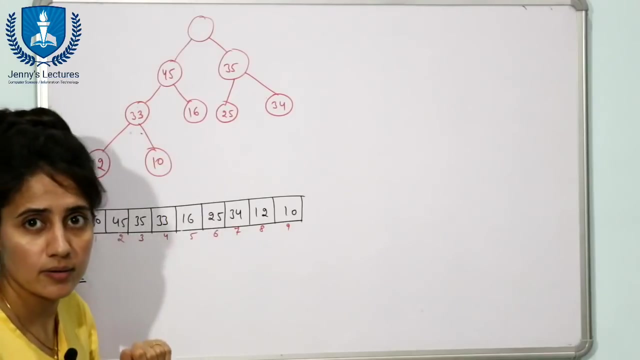 way is you can delete this 50 first of all. fine, so suppose you have deleted this 50 now at the place of 50. this place is empty. now, what you will do? which data? which data is to be here? so the last element, the last element, or you can say the last element in the array would be: 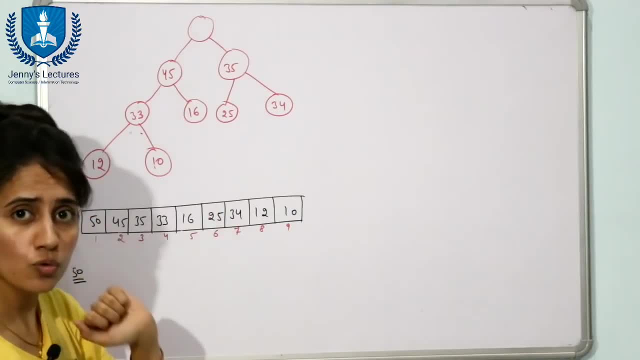 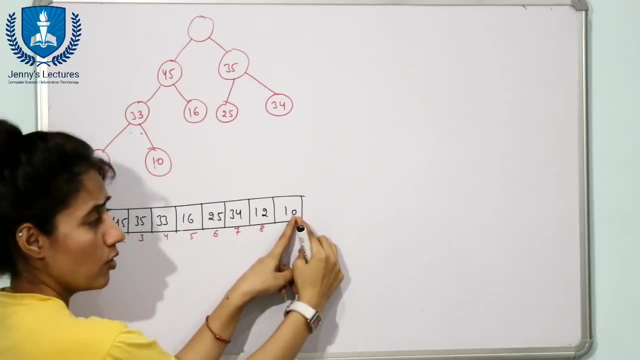 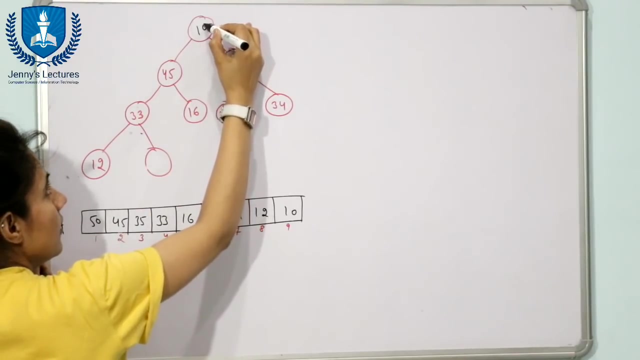 shifted to the root node because you have deleted this root node. so the last in the tree you can see the last data is what: 10. in the array also you can see the last is what- 10. so here what you will do this: 10- 10 would be deleted from here and 10 would be inserted at the place of root. 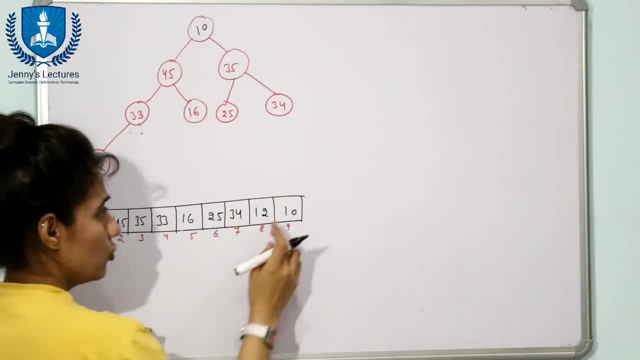 now the. this is our heap. so in this case also, we have deleted this 10 from here and we have inserted 10 here. only. here is now 10. now heap is up to this point. n minus 1 it's starting. n is what? nine now? 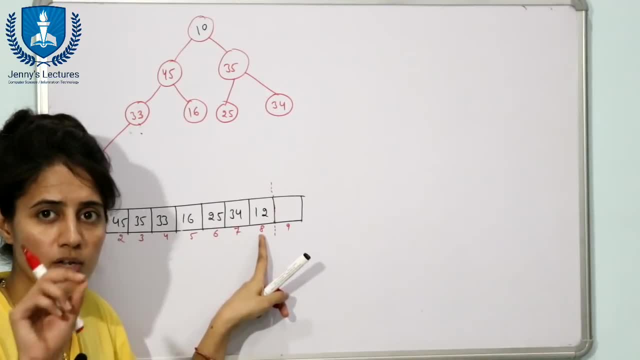 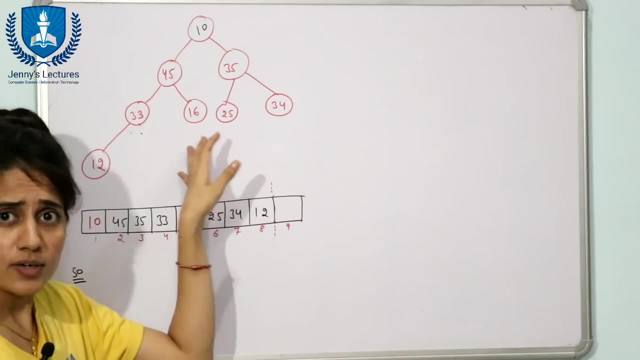 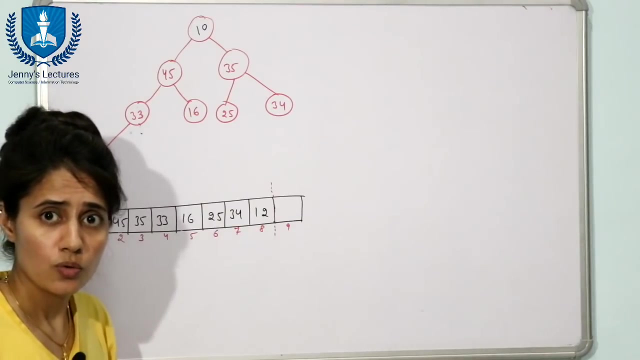 n is what after one deletion? n is what eight. so heap is now till n minus one. one size has been reduced. now see, now you have to check after deletion: is it still satisfying the maxi property? it is not like that: you have deleted 50 and you are done with with the deletion. no, you have to. 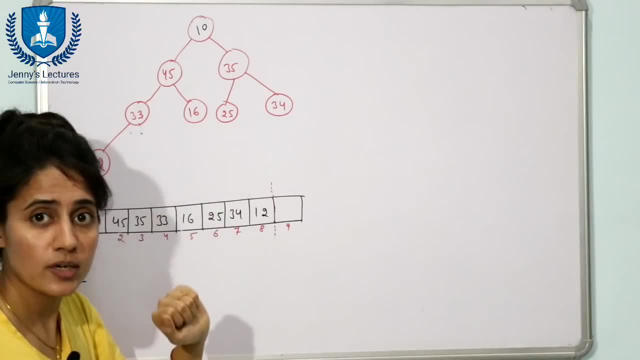 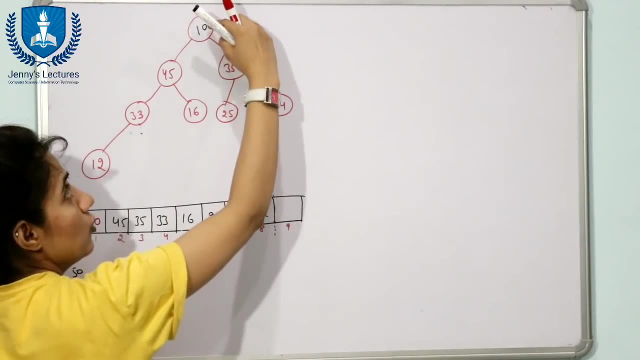 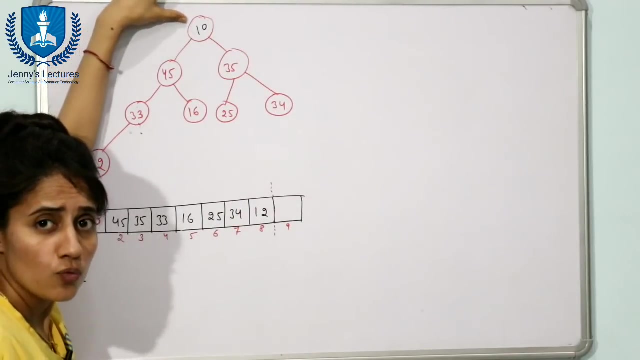 check this is satisfying maxi property or not. how you will check. now we have, we have, uh, we have shifted the last node to the root node. now you have to check. you have to compare this root node with its child, because the parent node would always be either greater than or equal to its. 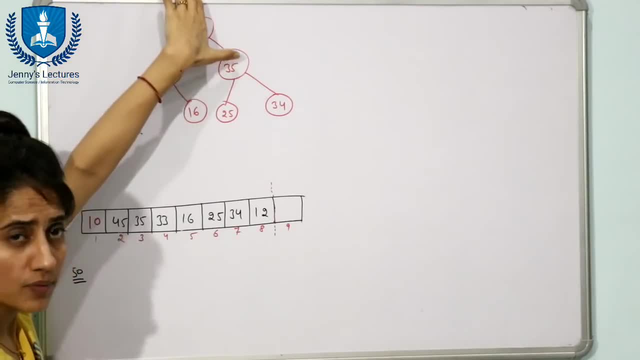 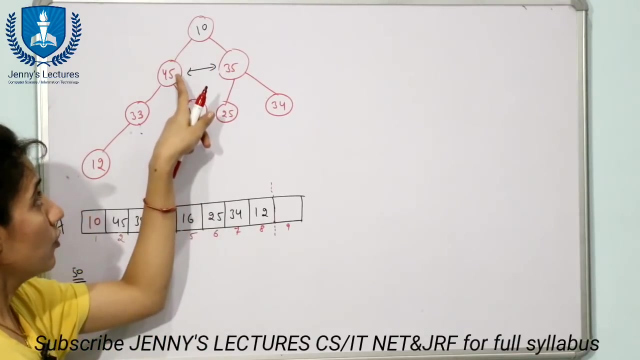 child node. now compare it is having two child. one is 45 and one is 35. which one is greater? 45 is greater. now compare this 45 with this root node, parent node. 45 is greater than this parent node, then obviously shifting would be done. 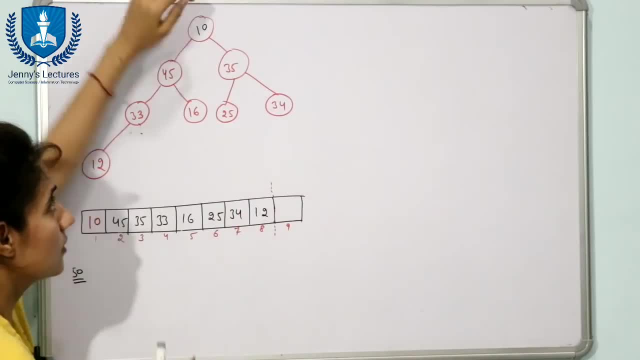 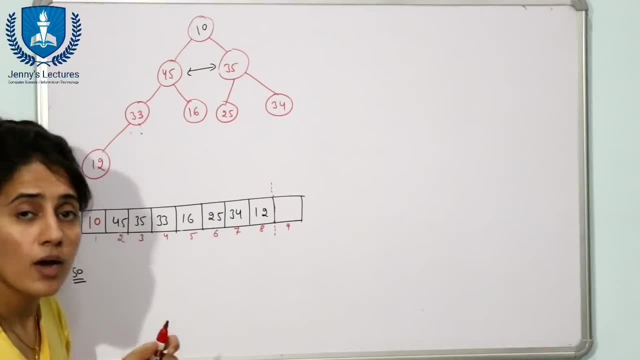 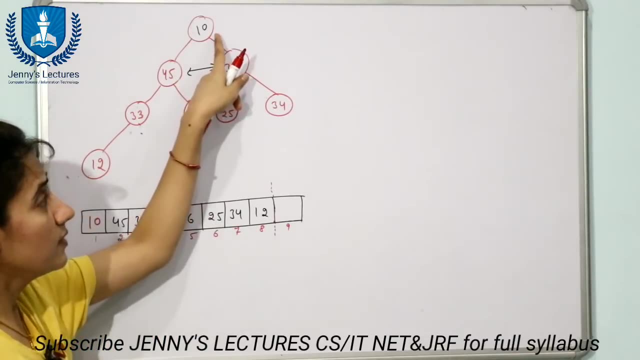 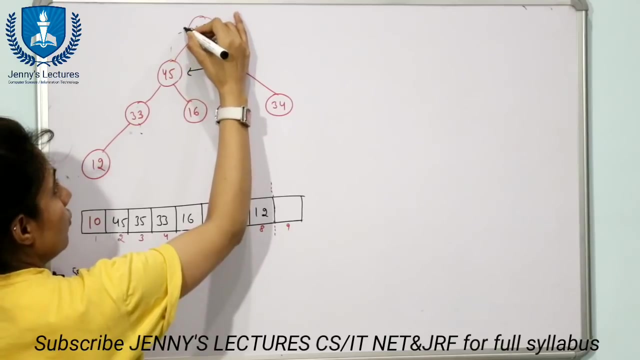 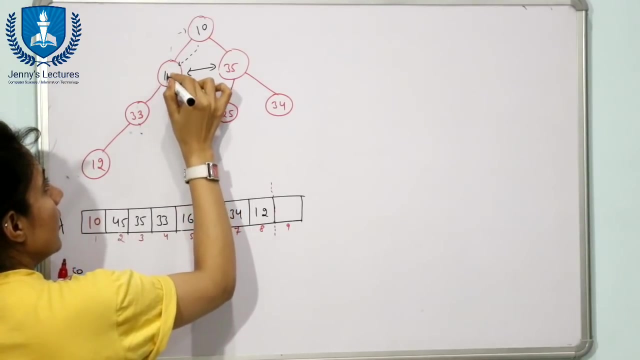 greater, 45 is greater. now compare this 45 with this root node, parent node. 45 is greater than this parent node. then obviously shifting would be done. now shifting would be done, 45 would go up and 10 would go down. right, so here now you will write 10 and here you will write what: 45. 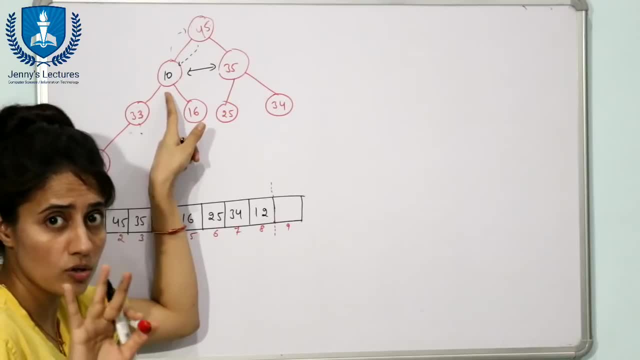 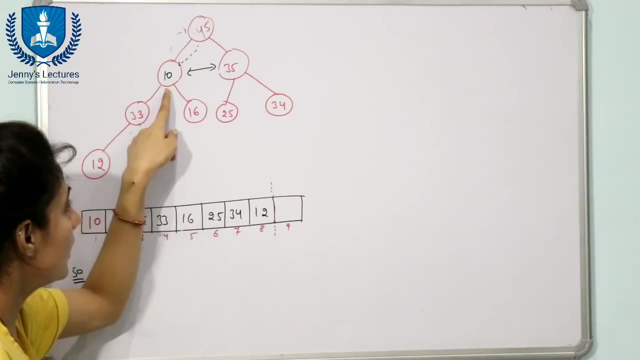 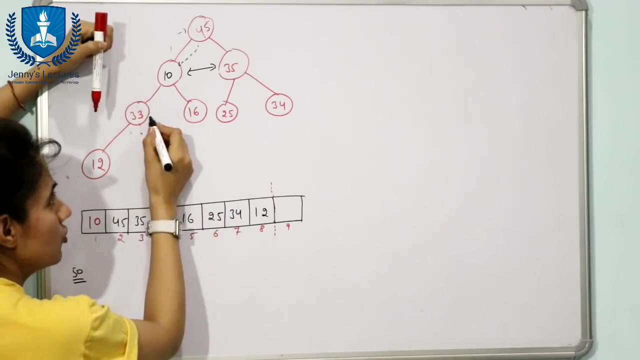 this is holding will start up and the operator is picked. so the modelx is calm down and the conditions include this. whatever this rule for thisurable self nullifier when? hmm, what is this? is my error? very bad protein here, so i will just write this one. i just i will do, i will go there. i mean this. 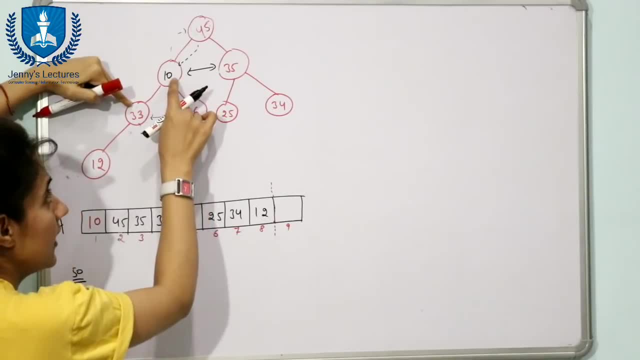 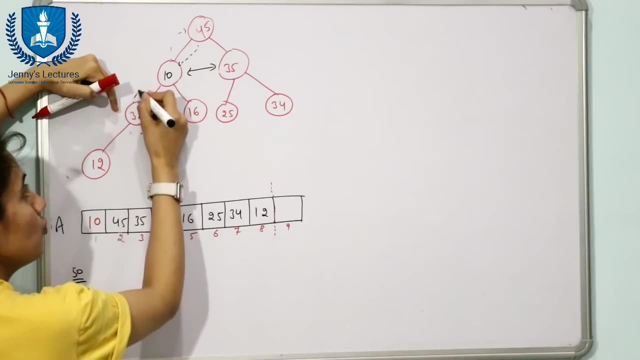 one by itself means that statef står d specialar, the statef shoulder is the stinker, and here the distribution of says that should be. the result will be 1.22. we are ourselves then give 12 and node equal to its child node. so we have to do swapping like this now: 10 would go down and 33. 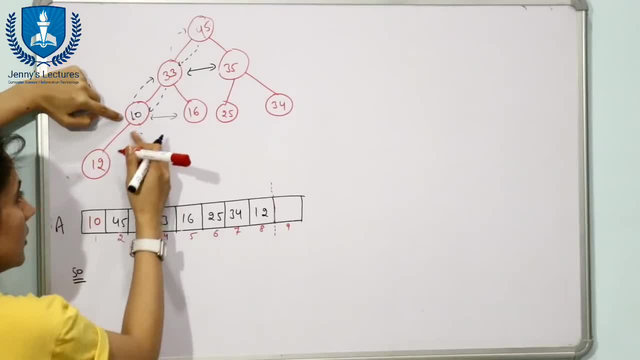 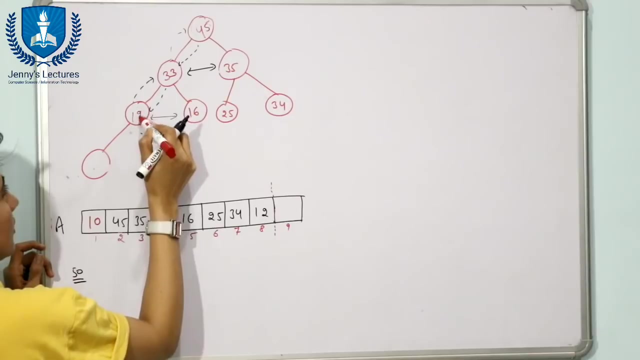 would go up. still, we have one child left. now calculate child is there? yes, one child is there, another is not there. now compare with this one: this parent node is less than its child node. then swapping would be done in mix heap. so now 12 would go up and 10 would go. now 12 is here. 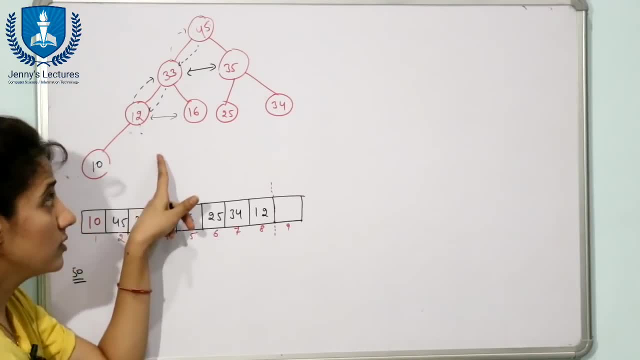 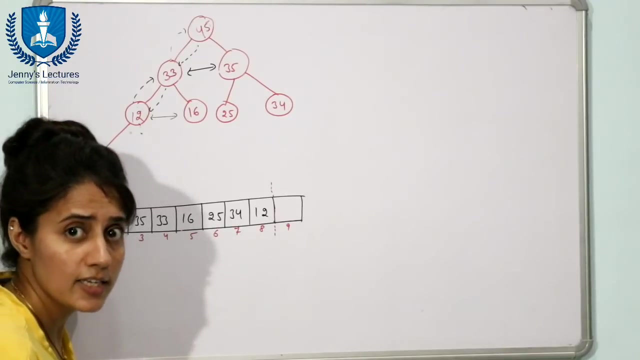 and 10 is at this place. now this is the tree. now this is satisfying the mix heap property. so this is how you you are going to delete now, if you, if you implement this, this here, only then how you will implement in this array. see, here we have 10 in deletion. in deletion you are going to 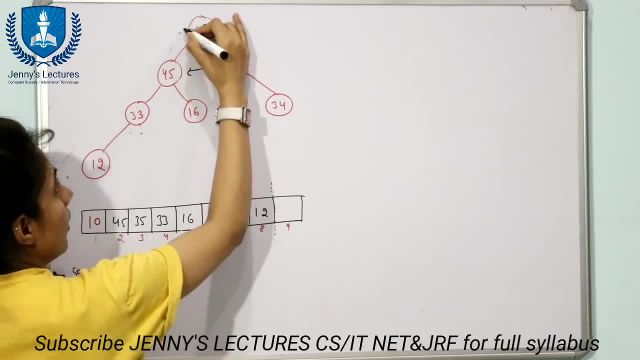 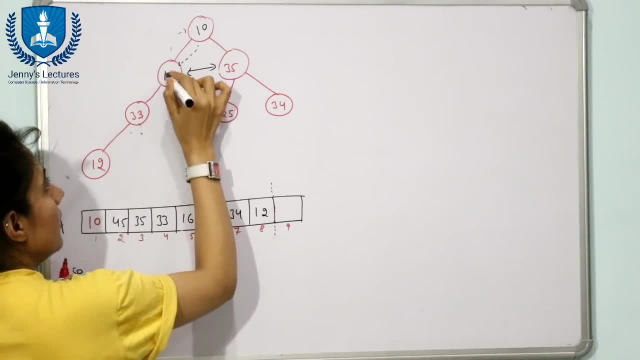 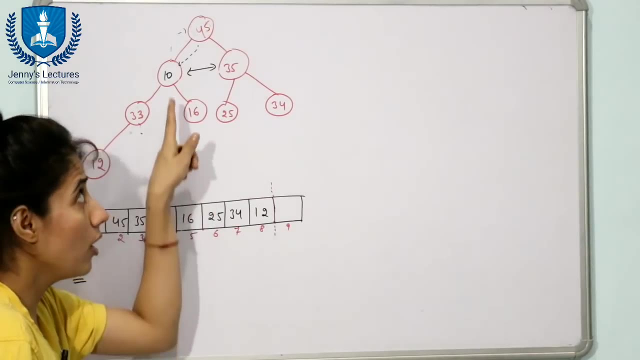 now compare this root node with its child, because the parent node would always be either greater. now shifting would be done: 45 would go up and 10 would go down. right, so here, now, you will write 10 and here you will write what, 45. this is not done now. this is not done now. this, this process. 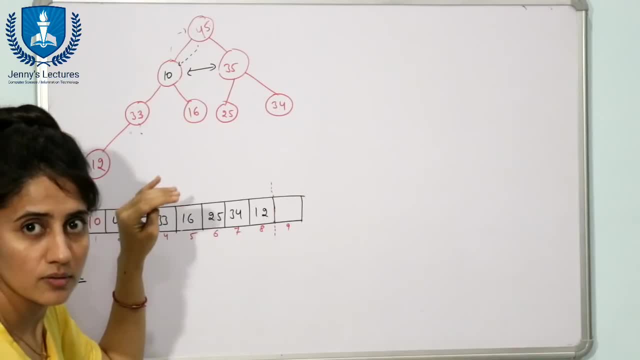 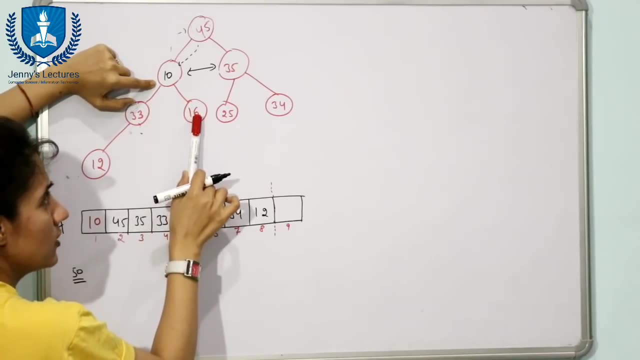 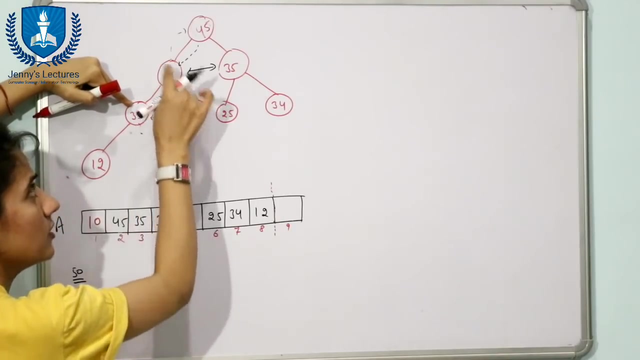 will be continued till we, till we reach to the last level. fine, now again, 10 would be compared with its child, child node. one is this one, one is this one. now compare these childs. which one is larger? 33 is the larger one. so now we compare this 33 with this 10. 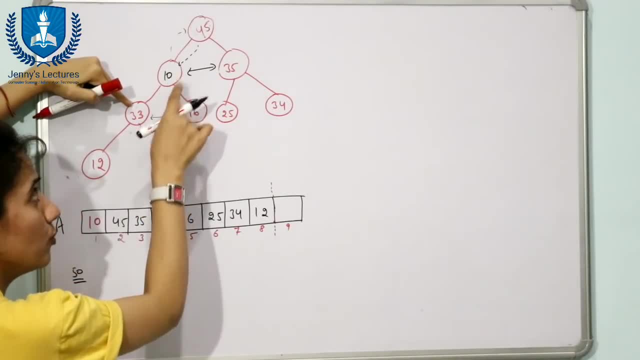 obviously 10 is less than 33, but root the parent should be greater than or equal to it's child node. so we have to do swapping like this: now 10 would go down and 33 would go up. still, we have one child left. now calculating now, we will do the following: now 10 would go down and 33 would go up. 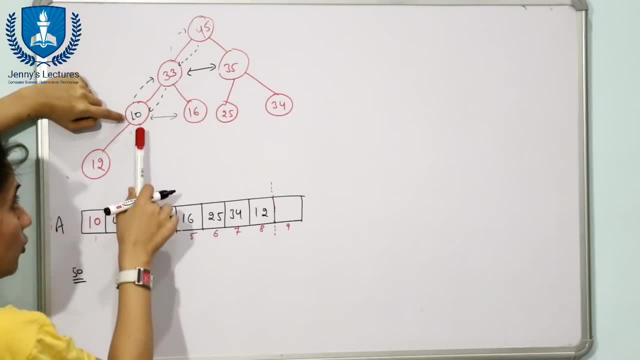 still we have one child left. still, we have one child left. now calculating, now calculating: child is there? yes, one child is there, another is not there. now, compare with this one: this parent node is less than its child node. then swapping would be done in maxi. so now 12 would go up. 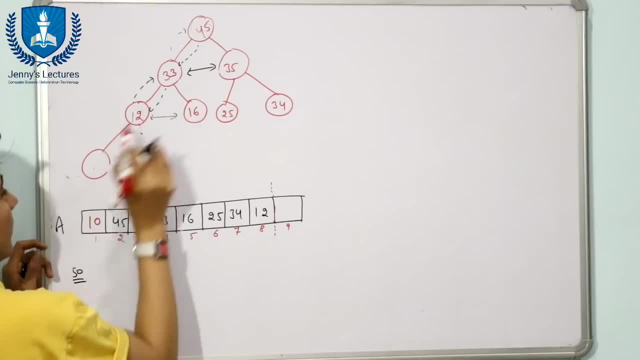 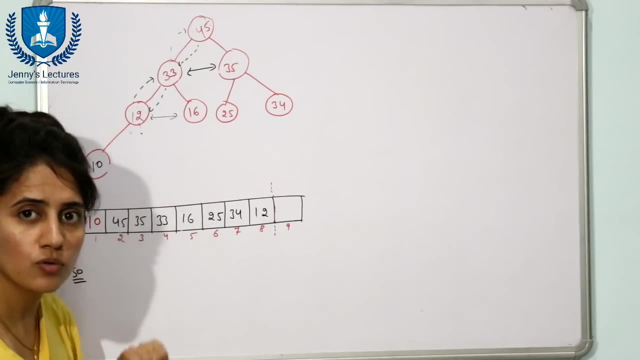 and 10 would go. now, 12 is here and 10 is at this place. now this is the tree, now this is satisfying the maxi property. so this is how you, you are going to delete now if you, if you implement this, this here, only then how you will implement in this array. see, here we have 10 in deletion. in deletion. 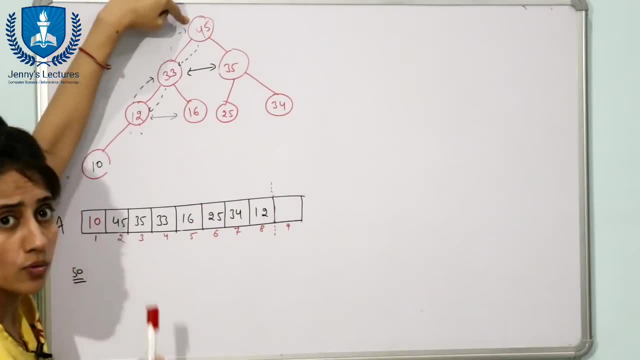 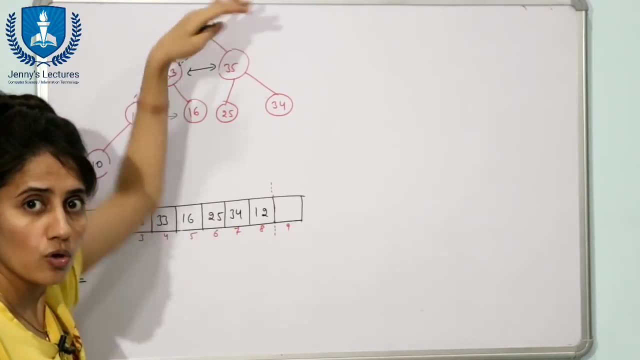 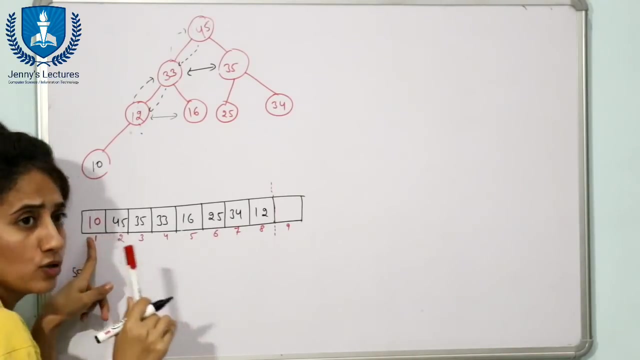 you are going to adjust the tree from top to down, and when we were inserting in that case, we were adjusting the tree from here, bottom to top right. so now 10, 10 is there? now, find out the child node of this 10, because we are going to compare this 10 with its children. fine, now. 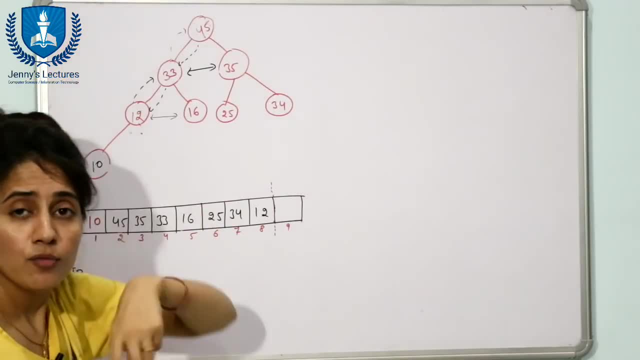 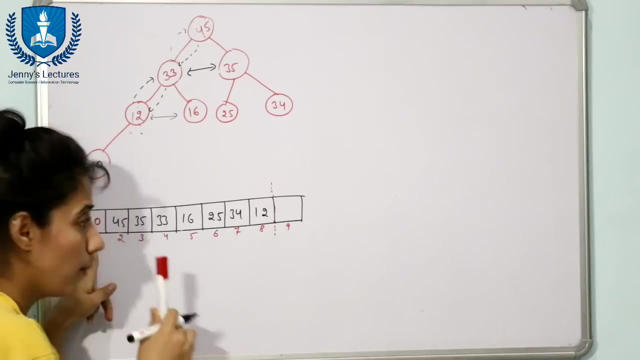 adjust the tree from top to down, and when we were inserting in that case we were adjusting the tree from here, bottom to top, right. so now 10, 10 is there? now find out the child node of this 10, because we are going to compare this 10 with its children. fine, now left child would be at. 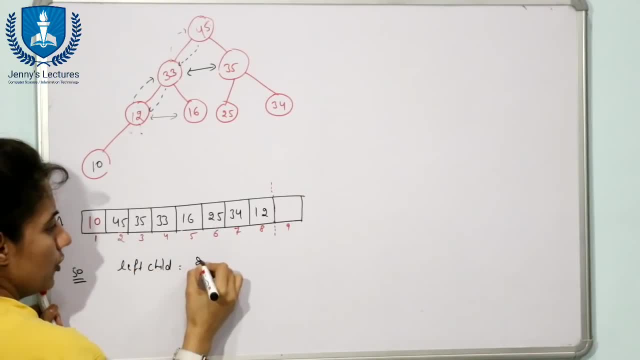 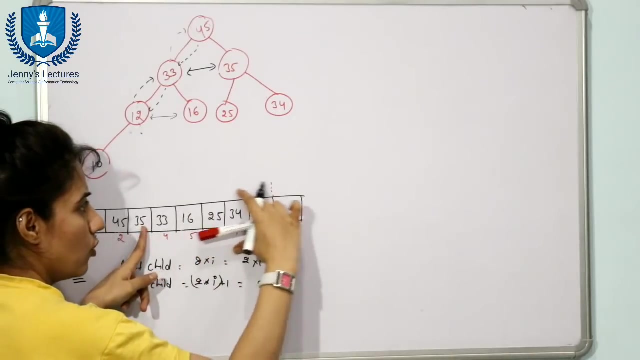 2 into i, that is 2 into 1 at second index and right child would be at 2 into i plus 1, that is at third. second and third means 45 is left child and 35 is right child. when you are you are, you are considering only this array. so in the tree also 45 was the left. 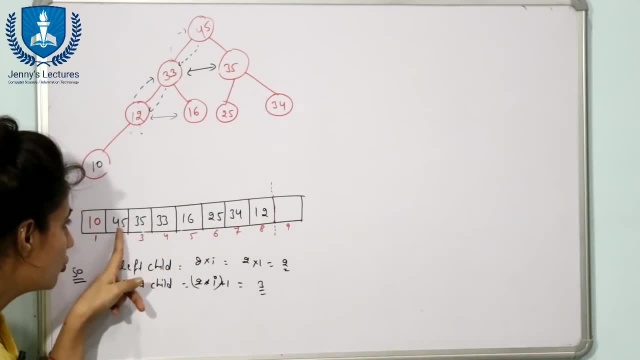 child and 35 was the right child. now compare these two childs. which one is larger? 45 is larger. now we compare this 45 with this 10. now, 10 is less than 45. now we are going to swap. now we will do what swapping now. 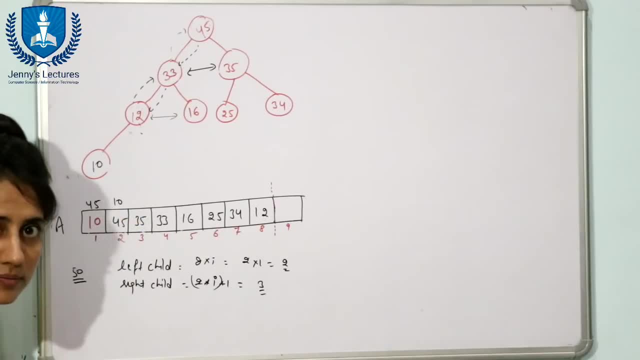 10 would go here and 45 would go here. right now, updated arrays: here we have 10 and here we have 45. now again, 10 is here, but we are not done. we will still calculate the left child of this 10 and right child of this 10. 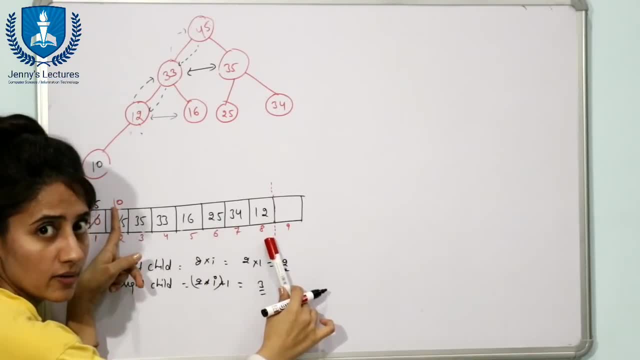 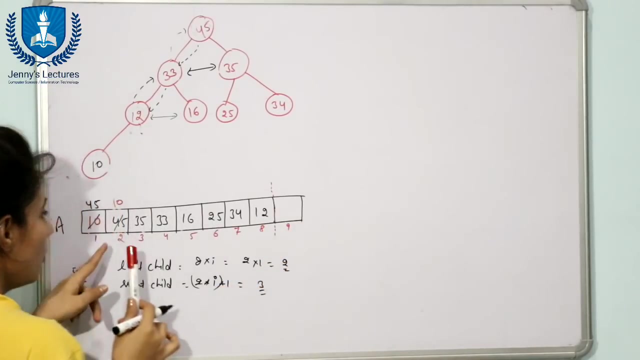 until we have reached up to this n. when you find out the left child is greater than this 8 and right child is also greater than this 8th index, then you are going to stop fine, because obviously after 8 we are not having any node. so now see, now i value is equal to. 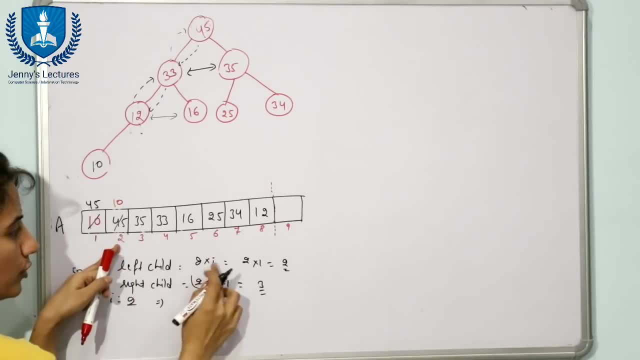 2 now. so let's see: left child would be at 2x2, that is, 4, and right child would be 2x2 plus 1, that is at 5. 4 and 5 means 33 and 60. now out of these, which one is larger, that is 33. 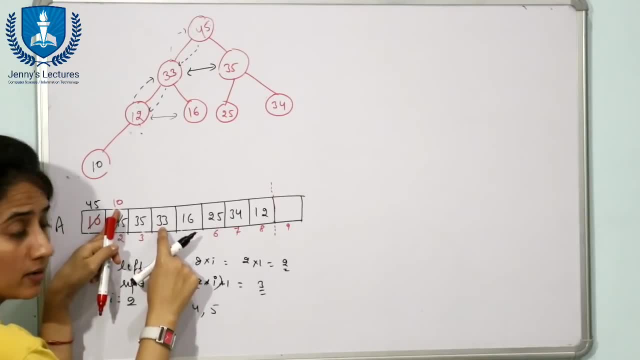 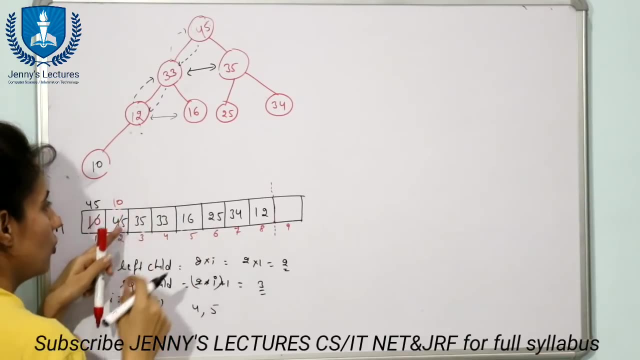 now compare 33 with this: 10. 10 is parent and 33 is its child. so parent can not be less than child in make. see, now you have to swap these two now: at the place of 33 we will write 10, and at the place of 10 you will. 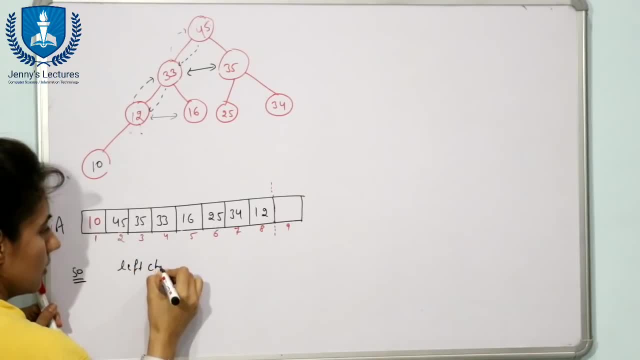 left child would be at 2 into i, that is 2 into 1 at second index, and right child would be at 2 into i plus 1, that is at third. second and third means 45 is left child and 35 is right child. when you are you are, you are considering only this array, so in the tree also 45 was. 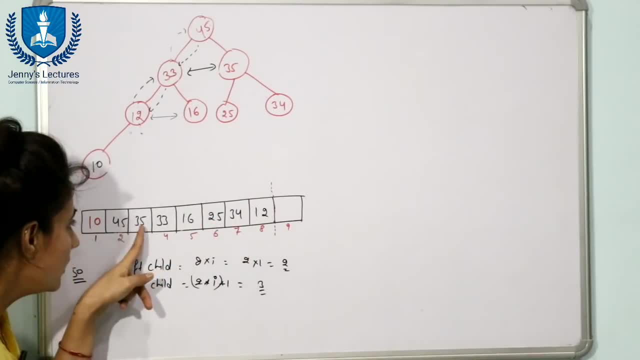 the left child and 35 was the right child. now compare these two childs. which one is larger? 45 is larger. now we compare this 45 with this 10. fine, now 10 is less than 45. now we are going to swap. now we will do what swapping. now, 10 would go here and 45 would go here. 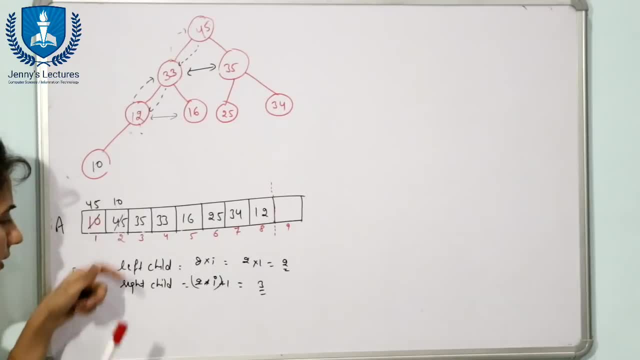 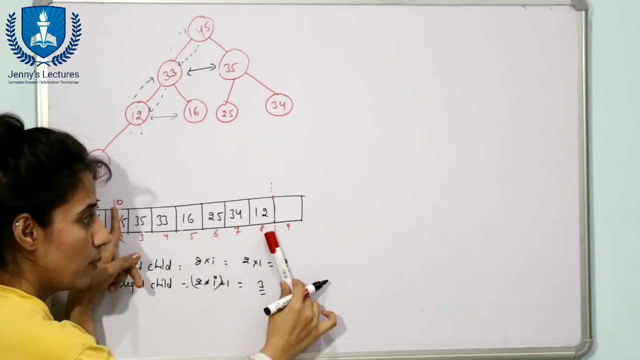 right now updated arrays: here we have 10 and here we have 45. now again 10 is here, but we are not done. we will still calculate the left child of this 10 and right child of this 10 until we have reached up to this n, when you find out the. 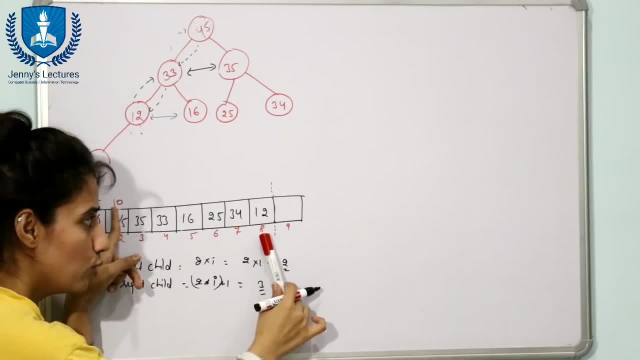 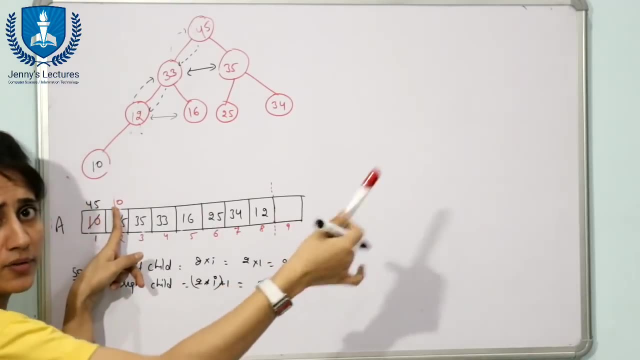 left child is greater than this 8 and right child is also greater than this eighth index, then you are going to stop. fine, because obviously after 8 we are, we are not having any node. so now, now, see now i value is equal to 2 now. 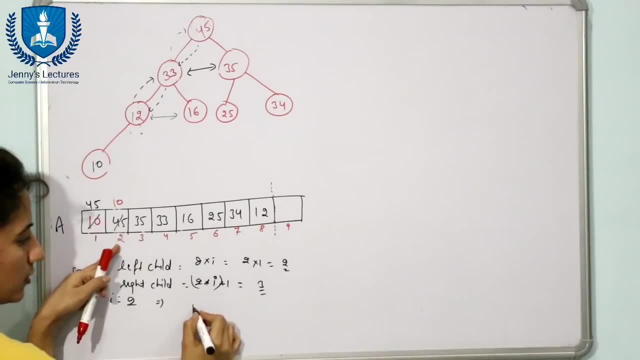 so now. so left child would be at 2 into 2, that is 4, and right child would be 2 into 2 plus 1, that is at 5. 4 and 5 means 33 and 60. now out of these, which one is larger? that is 33 now. 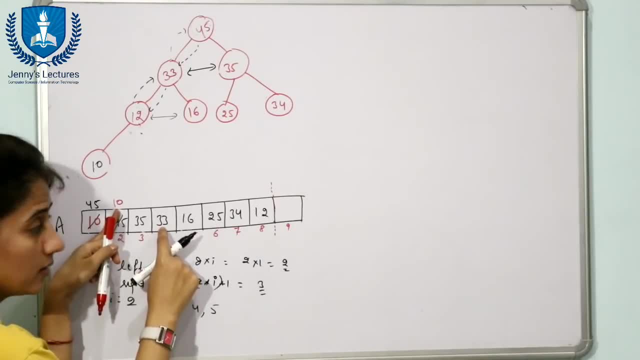 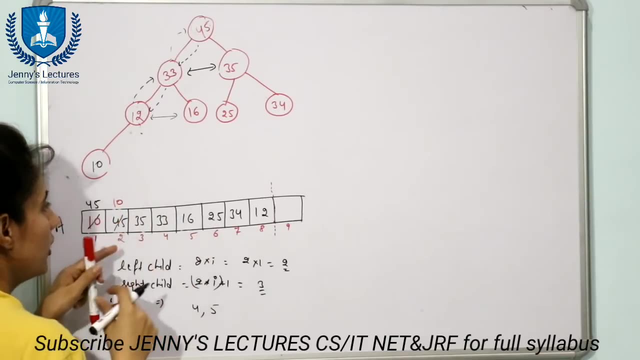 compare 33 with this: 10. 10 is parent and 33 is its child. so parent cannot be less than child in mexico. no, now you have to swap these two. now, at the place of 33, we will write 10, and at the place of 10 you will write what? 30.. 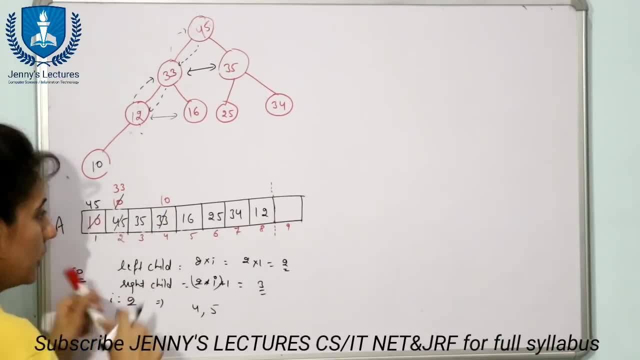 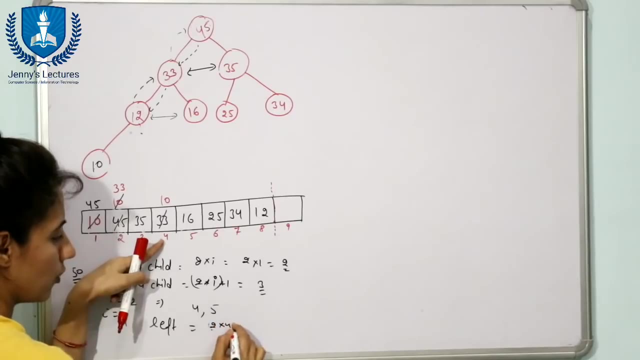 so now here we have 10. now i value is 4. now now again calculate left child of this and right child of this. so left child would be at 4 into 2 into i, that is, 2 into 4 at index 8, and right child would be 2 into 4 plus 1, that is at 9. so find out: at 8, yes, 9, we don't. 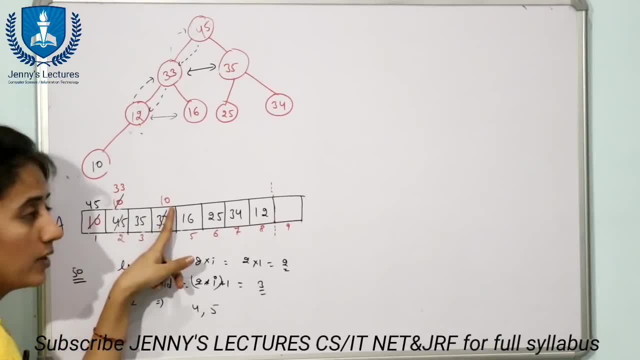 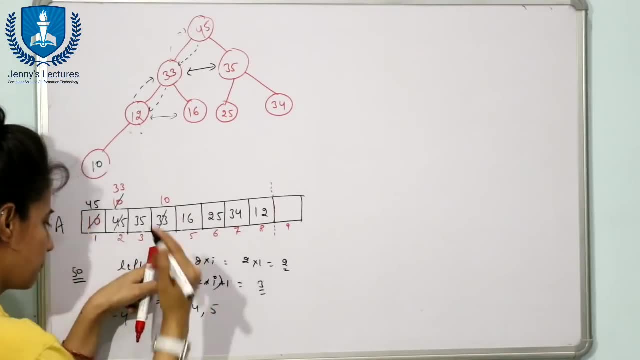 write what 30, 3 now here we have 10. now i value is 4. now now again calculate left child of this and right child of this. so left child would be at 4x2, that is, 2x4 at index 8, and right child would be two into 4 plus. 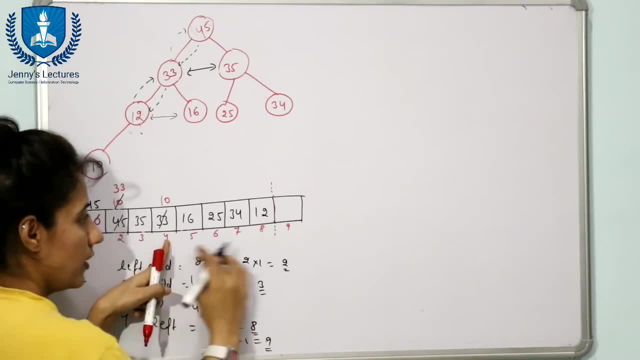 one that is at nine, so find out at eight. yes, nine. we don't have any 9th index. we don't have any value in this 9th index, so the total will be 1 over the. So this is. we are not going to compare this, right child. 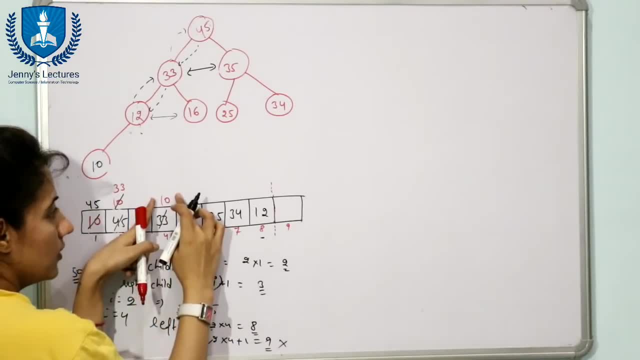 We are going to just compare this left child. Now compare this 10 with this index. the value having at index 8 with its left child, 10 is less than its child. So you are going to swap this thing. So here we will write 10 and here you will write word 12.. 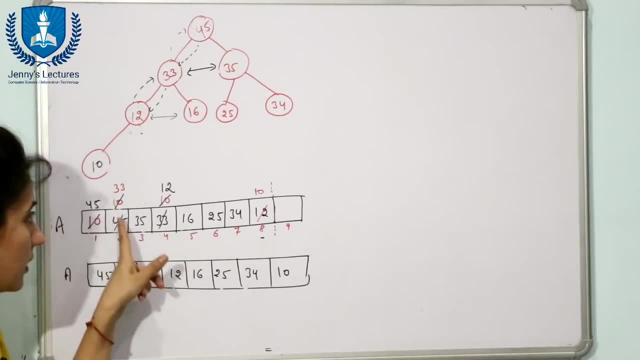 This is what we have done in this tree. So after doing this updation, the array would be something like this: This is how we are going to delete and see: here we have one space left, at 9th We have 8. here we have 7,, 6,, 5,, 4,, 3,, 2 and 1, and the deleted item was 50 right. 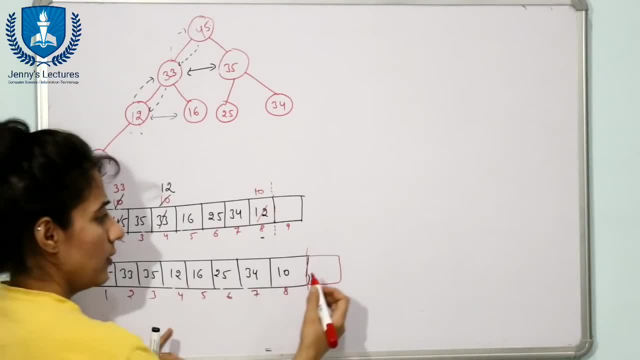 So what you can do, you can simply do what you can: put 50 at this place. You can use the space See, although the heap is from 1 to 8, but this space is free in an array, So you can the deleted element. 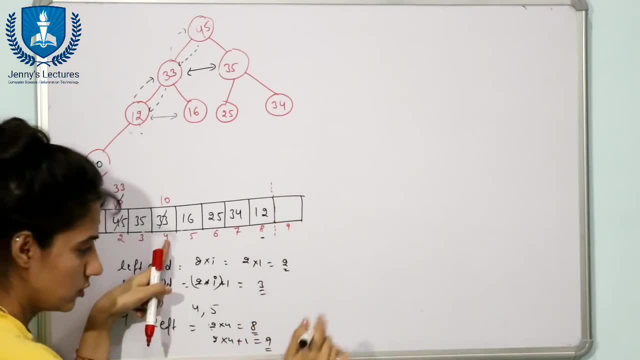 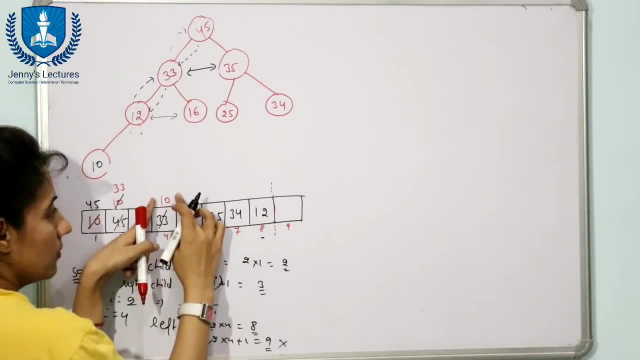 have any ninth index. we don't have any value in this ninth index. so so this is. we are not going to compare this right child, we are going to just compare this left child. now compare this 10 with this index, the value having at index 8 with its left. 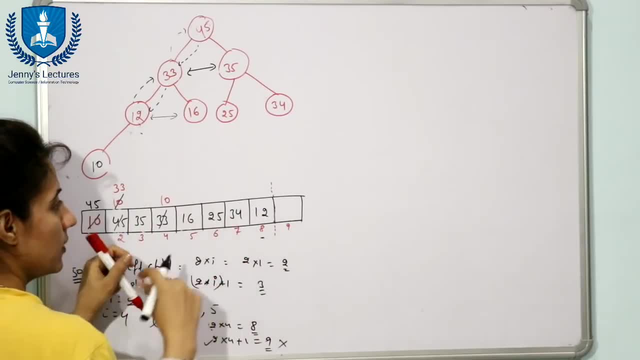 child 10 is less than its child, so you are going to swap this thing. so here we will write 10 and here you will write word 12.. this is what we have done in this tree. so after doing this updation, the array would be something like this: 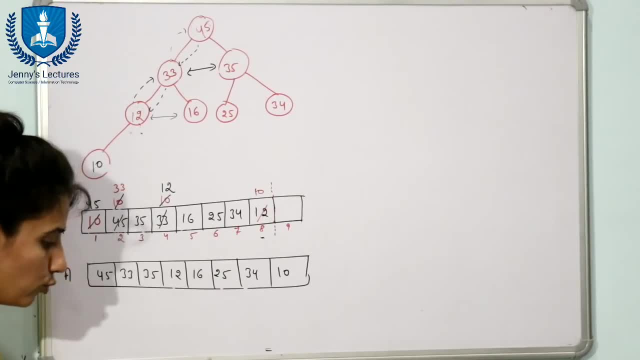 fine, fine, fine. this is how we are going to delete and see, here we have one space left, at 9th we have 8. here we have 7, 6, 5, 4, 3, 2 and 1, and the deleted item was 50, right, so what you can do, you can. 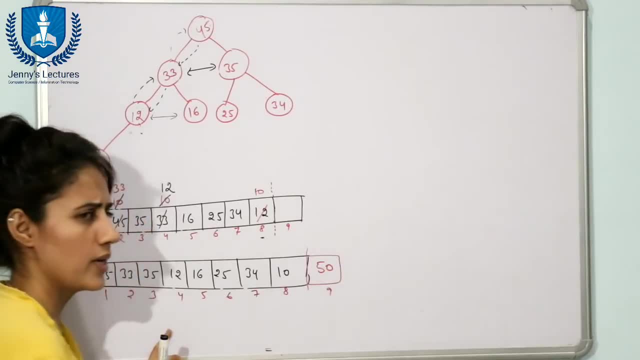 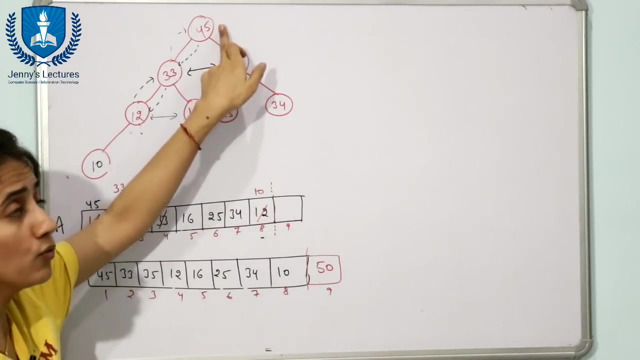 simply do what you can. put 50 at this place. you can use the space see, although the heap is from 1 to 8, but this space is free in an array, so you can. the deleted element can be put here only now. see next. next deletion check. next deleted element would be 45, because we can only delete. 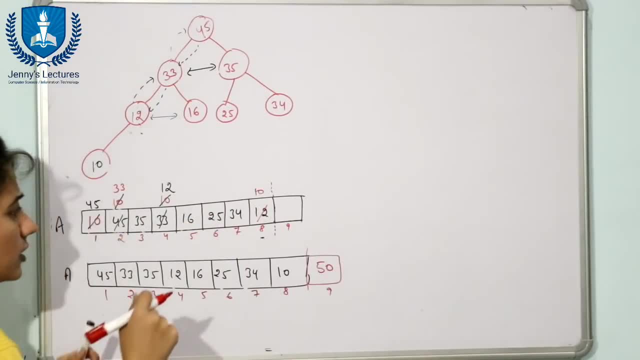 data from the root node. fine, now see. suppose 45 has been deleted. now, what now? 45 has been deleted, 45. next element is 45. what after deletion? what you will do? you will replace this. you will put here the last element in this tree. last element is 10, or you can see in the array. 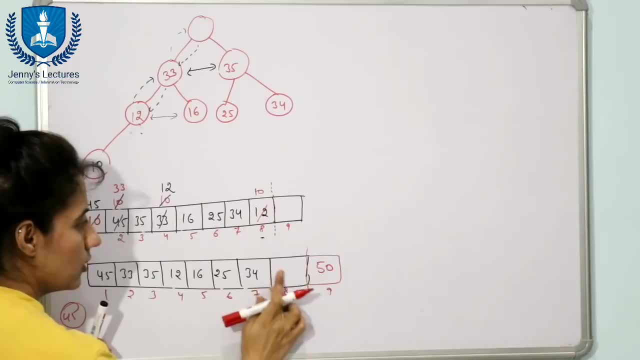 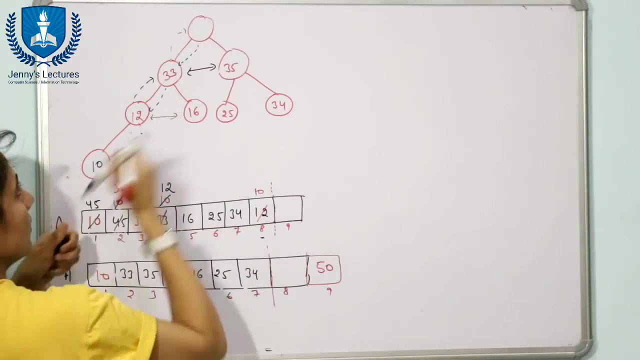 last element is 10. so now we are going to put this 10 at this place. and now, now heap is till 1 to 7 and this space is free. fine, now, here you will write what: 10, and we are going to delete this from this tree. but now, 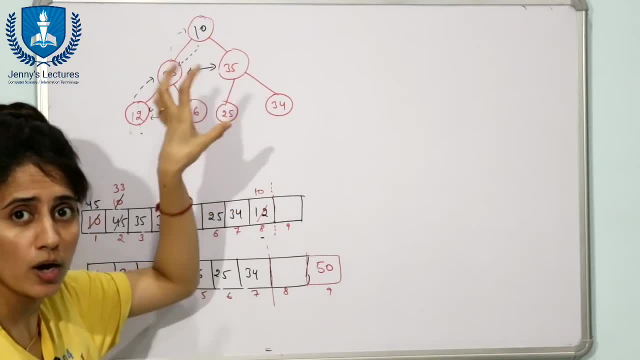 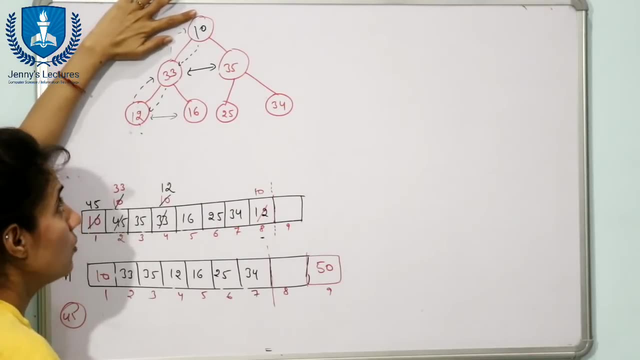 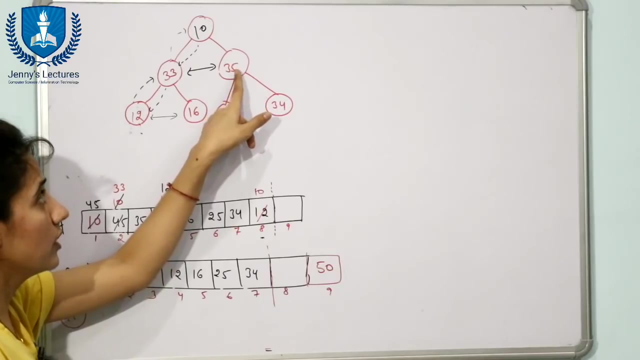 this is not the deletion. now you have to heapify this again. you have to check it is satisfying the maxheap property or not. now 10 is here. calculate its child node. child node are 33 and 35. which one is greater? 35 is greater out of these node. now 35 would be compared. 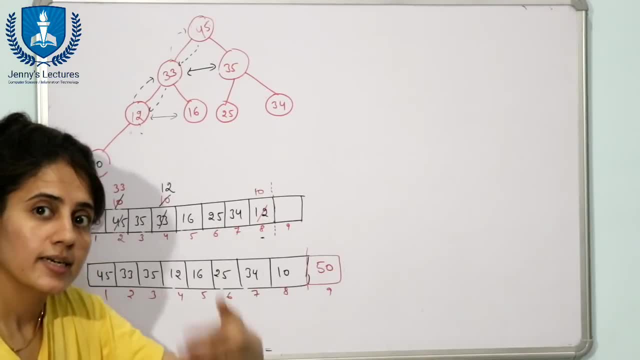 You can be put here only Now. see next. next deletion check. Next deleted element would be 45, because we can only delete data from the root node. Fine, Now see, suppose 45 has been deleted. Now what now? 45 has been deleted. 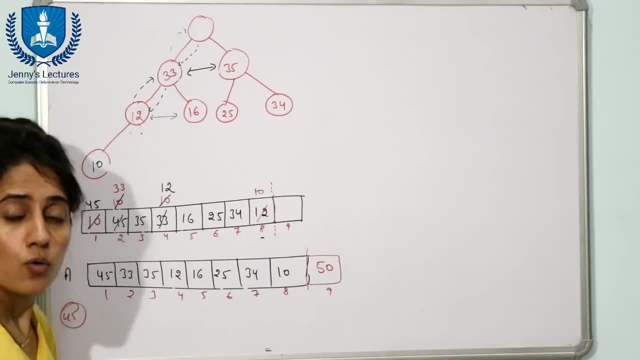 45. next element is 45.. What, after deletion? what you will do? you will replace this. You will put here the last element in this tree. Last element is 10.. Or you can say in the array, last element is 10.. So now you are going to put this 10 at this place. 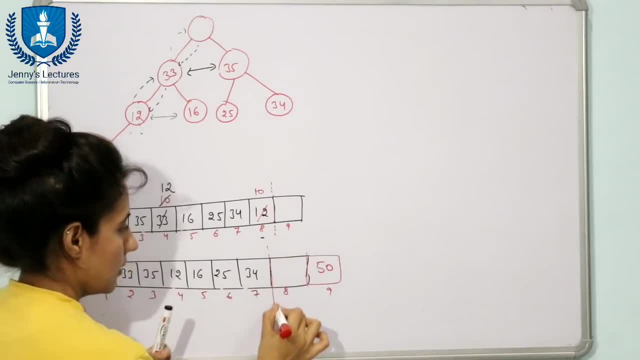 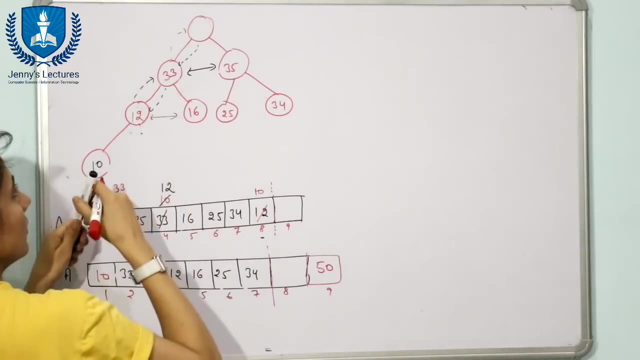 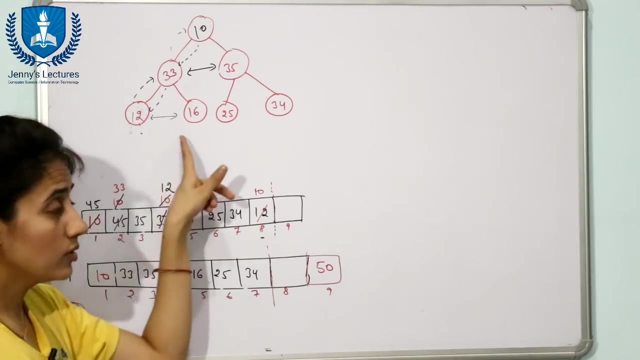 And now? now heap is till 1 to 7 and this space is free. Fine, Now, here you will write what: 10, and we are going to delete this from this tree. But now, this is not the deletion. Now you have to heapify this again. 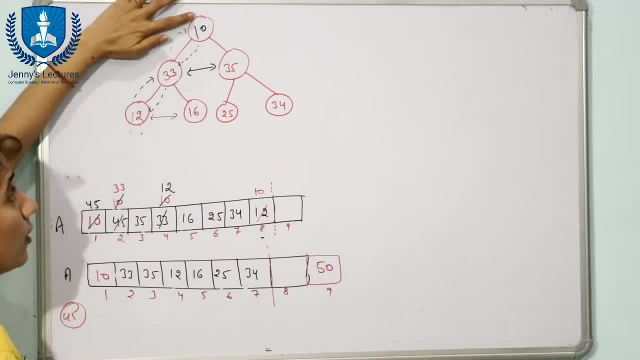 You have to check it is satisfying The max heap property or not. Now 10 is here. calculate its child node. Child node are 33 and 35. Which one is greater? 35 is greater out of these node. Now 35 would be compared with its parent, that is 10.. 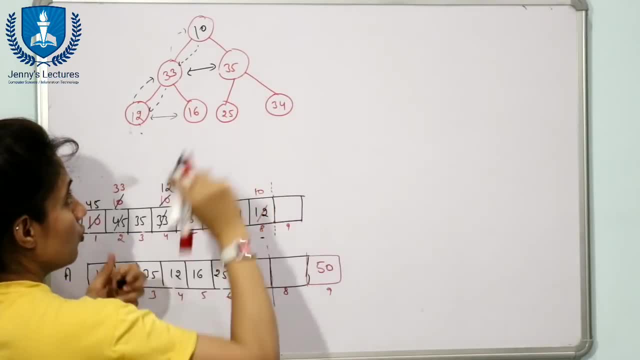 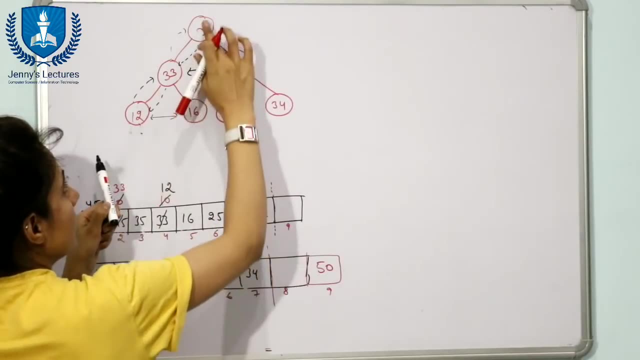 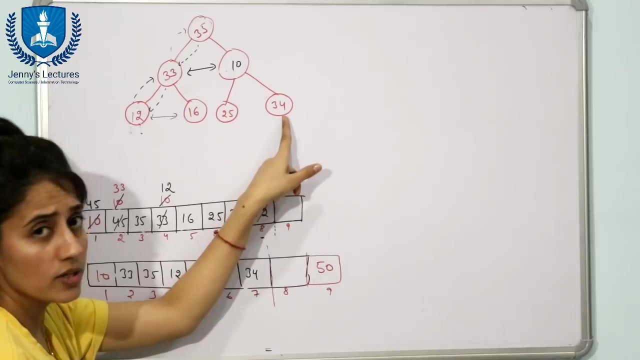 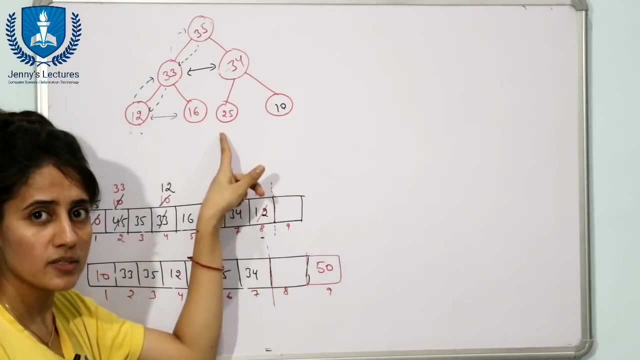 So now 10 is less than 35. that is not possible in max heap. So you are going to swap this thing. So here you will write 35 and here you will write 10. 10. Now again, calculate This: left and right child: 25 is left, 34 is right. compare these two: which one is greater? 34 is greater. now compare 34 with this 10: 10 is less than 34. that is not possible. now you have to swap this thing. here you will write 34 and here you will write 10. this is the mix heap after deletion of 45. 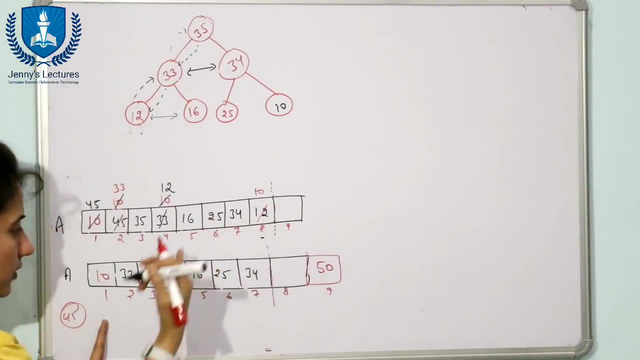 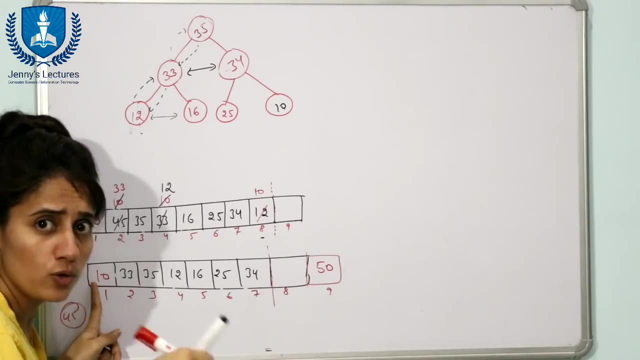 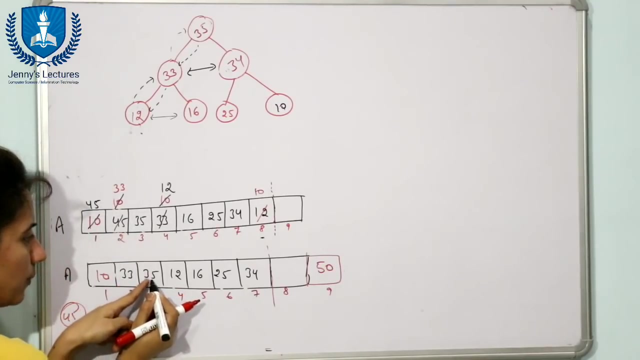 So same. you can do with this array like we have done in this case. find out the left and right child of this one. I is equal to 1.. So left side- left side would be 2 into I, that is, 2. right would be 2 into I, plus 1, that is at 3, now 33 and 35. which one is larger? 35? compare 35 with this 10. so obviously 10 is less than 35. so parent cannot be less than child. so we are going to swap this thing. here you will write 10 and here you will write 35 again. 10 is at this place again. find out its left child: 2 into I, that is at 6th index, and 2 into I plus 1. right would be at 7th index. 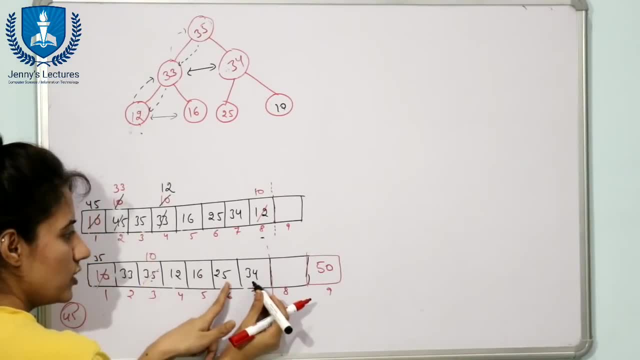 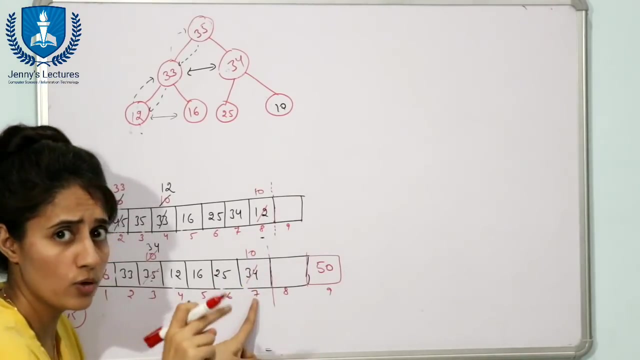 So these two would be child. Which one is greater? 34 is greater. 34 is compared with this 10. so 10 is less than 34. that is not possible in mix heap parent should be greater than or equal to its child node. so now you are going to swap: here you will write what 34 and here you will write what 10. now again, 10 is here. now again. calculate its left child. left child would be 2 into I, 7 into 2, that is 14. but we are not having any 14th index. 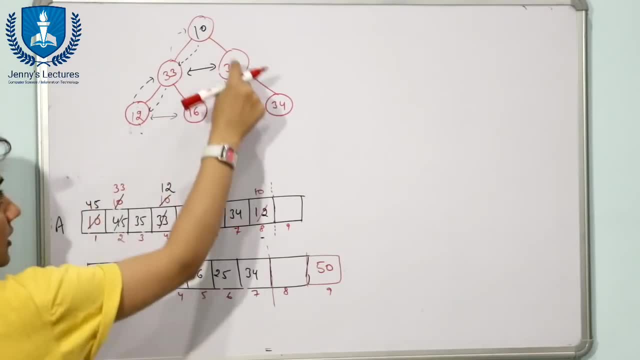 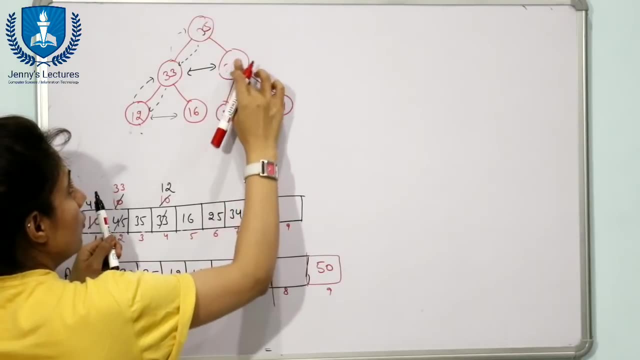 with its parent, that is 10. so now 10 is less than 35. that is not possible in maxheap. so you are going to swap this thing. so here you will write 35 and here you will write 10. now again calculate its child node. 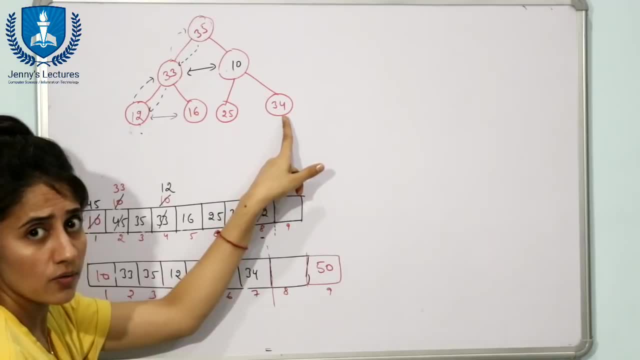 25 is left and right. child 25 is left, 34 is right. compare these two. which one is greater? 34 is greater. now compare 34 with this 10. 10 is less than 34. that is not possible. now you have to swap this thing: here you will write 34 and here you will write 10. this is the. 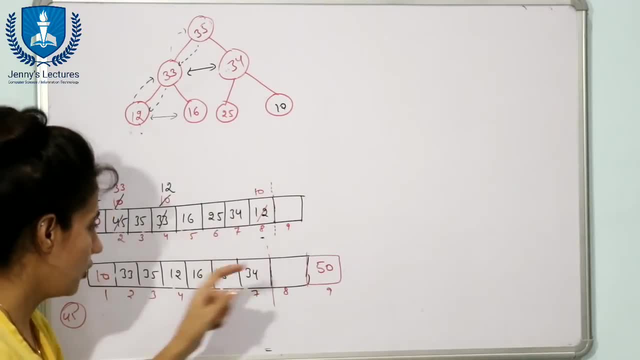 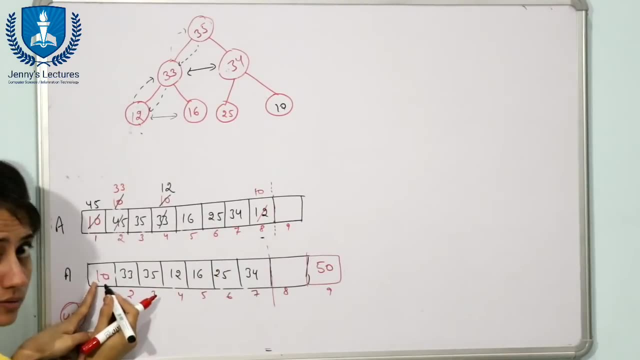 maxheap after deletion of 45. so same you can do with this array like we have done in this case. find out the left and right child of this one. i is equal to 1 and i is equal to 1. so left side- left side would be 2 into i, that is, 2. right would be 2 into i plus 1. 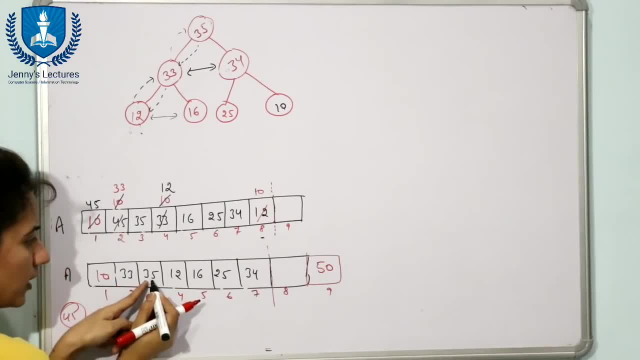 that is at 3. now 33 and 35. which one is larger? 35. compare 35 with this 10. so obviously 10 is less than 35. so parent cannot be less than child. so we are going to swap this thing: here you will write 10 and here you will write 35. again, 10 is at this place again. find out. 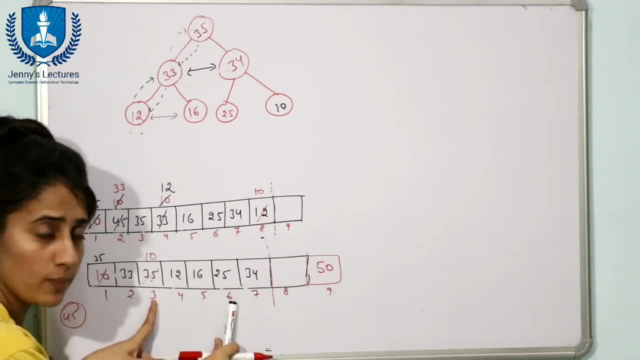 its left child. 2 into i, that is, at 6th index, and 2 into i, plus 1 right would be at 7th index. So these two would be child. Okay, Of children of this 10, which one is greater? 34 is greater. 34 is compared with this 10. 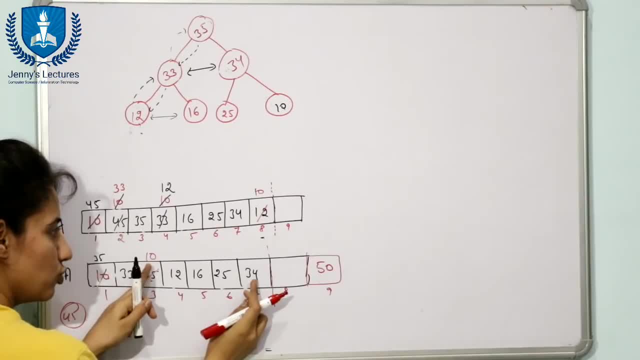 so 10 is less than 34. that is not possible. in maxheap, parent should be greater than or equal to its child node. so now you are going to swap. here you will write what 34 and here you will write what 10. now again, 10 is here. now again. calculate its left child, left child. 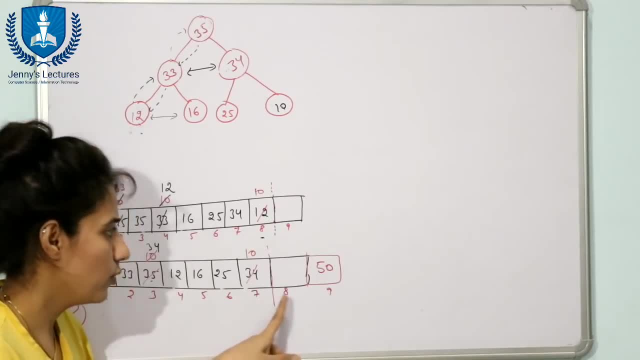 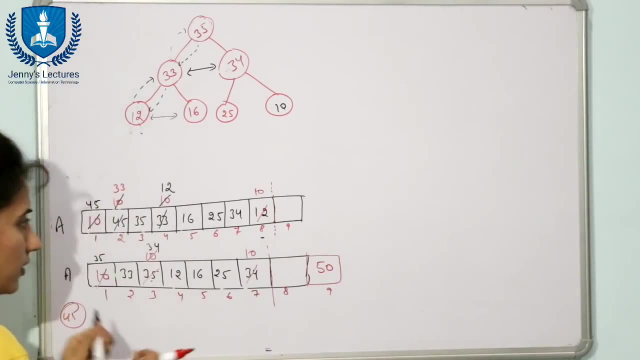 would be: 2 into i, 7 into 2, that is 14. but we are not having any 14th index, so now we are going to stop this. Fine, So now after. after this arrangement, the array would be something like this: 50 is there and. 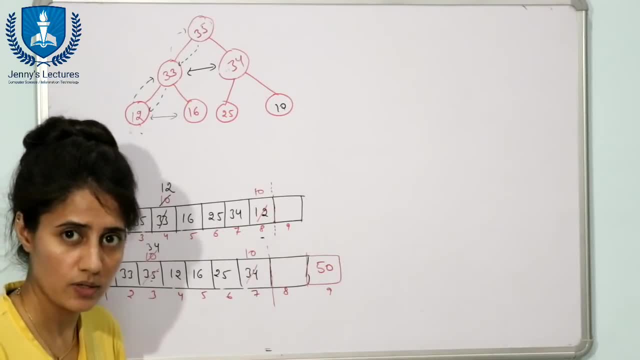 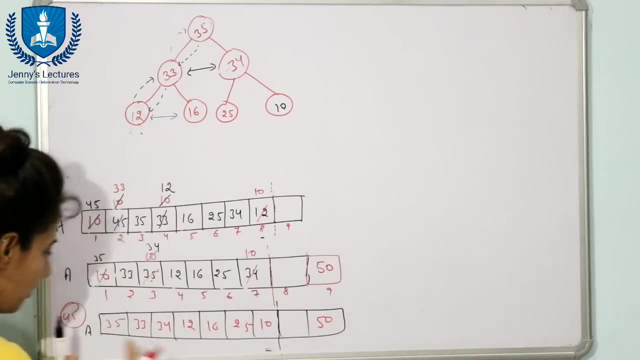 So now we are going to stop Find. so now, after this arrangement, the area would be something like this: 50 is there and next we have deleted element is 45, so we can store 45 here because this is free space. Okay, next element can be deleted as 35. so again, we will. we'll do what: 35 would go there and 10 would go here. 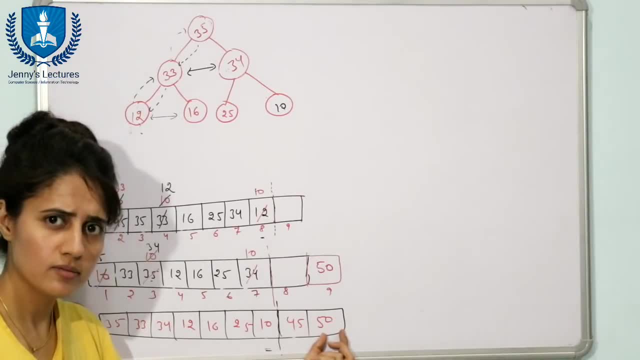 Now here I think you are analyzing that the largest element is at this position. now the second largest element again would be the third largest element would be at this place and when you you deleted all the elements, then this, this array, would be in sorted order. i hope you are getting this concept. 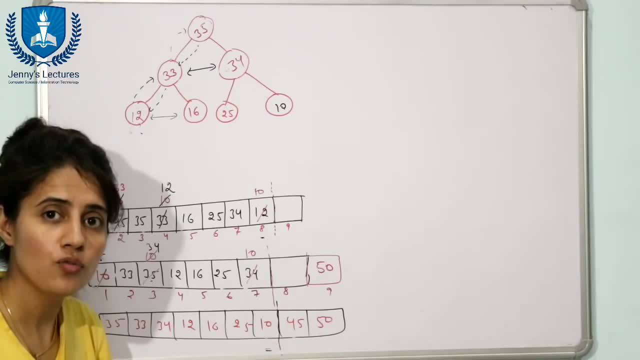 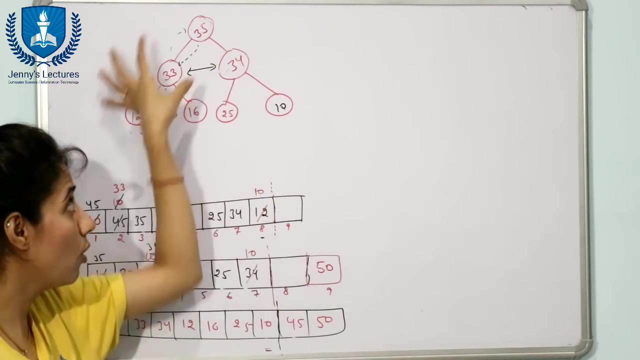 fine. so this is the basic, this, this is the base idea of heap sort. if you are going to, if you are going to sort the data in ascending order, then just build a max heap, delete one by one elements from the mix heap and after deletion, or after deleting of all the elements, you can find out. 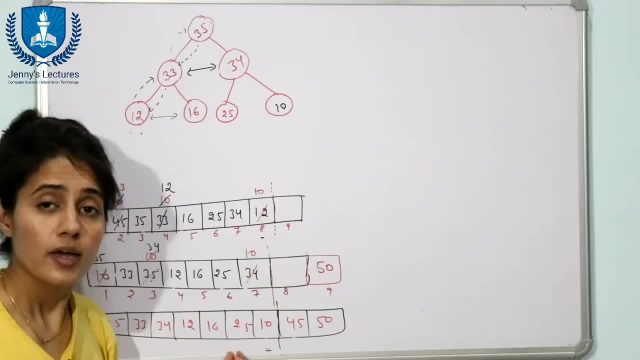 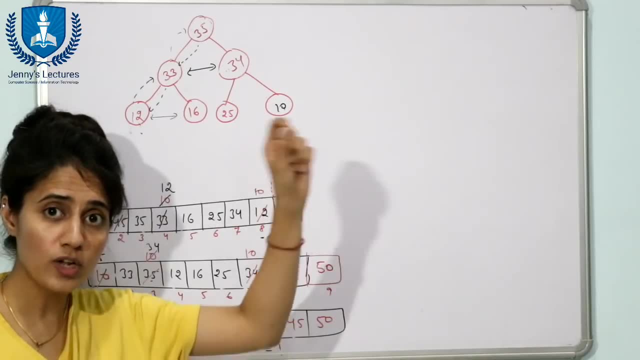 that your data is has been arranged in ascending order and if you want to sort the data in descending order then just use min heap, because the root element in min heap is the minimum element and obviously deletion would be from the root element. so that is why first element would 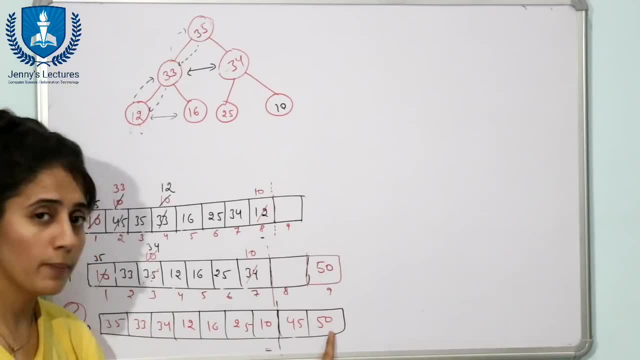 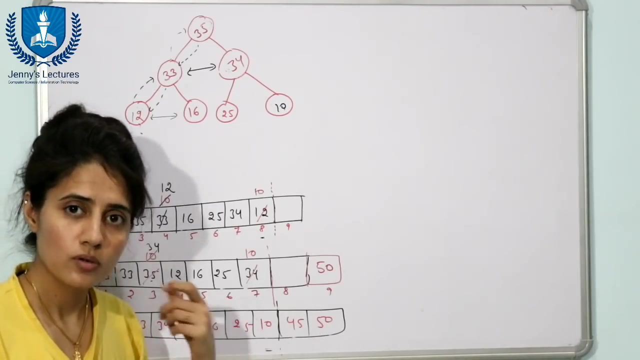 be deleted. the root element, so root element would be here only so the minimum element element would be here only then the next minimum, then the next minimum, the largest element would be at here only so data would be at that time in descending order. so this is the idea of heap sort. in next video i am going to discuss with you heap sort we are going to take. 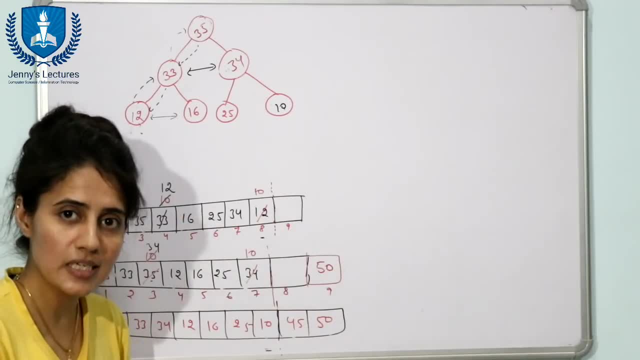 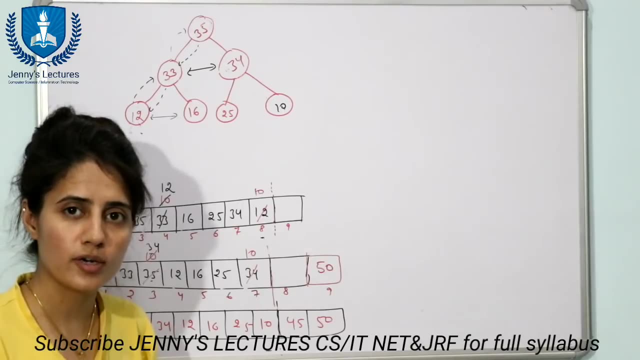 one array. we are going to construct a heap, first of all max heap, then we are going to delete one by one data from that max heap and ultimately you see that the data is sorted in ascending order. fine, and also we will discuss what is that heapify method. so i'll see in the next video. till then, bye. 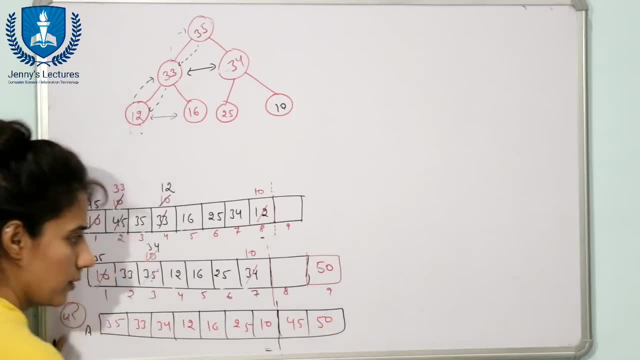 next we have deleted element is 45, so we can store 45 here because this is free space. okay, next element can be deleted as 35. so again, we will do what: 35 would go there and 10 would go here. now, here, I think you are analyzing that the largest element is at the this position. 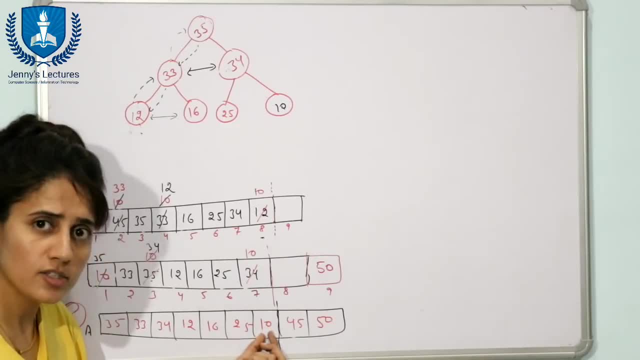 now the second largest element Again would be: the third largest element would be at this place and when you you deleted all the elements, then this, this array, would be in sorted order. I hope you are getting this concept fine. so this is the basic, this, this is the base idea of heap sort, if you. 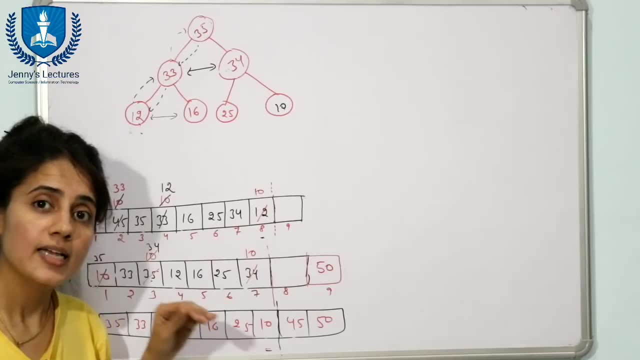 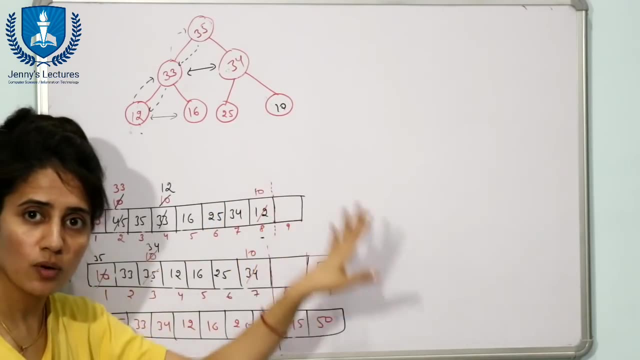 are going to. if you are going to sort the data in ascending order, then just build a max heap, Delete. So if you are going to sort the elements from the mix heap and after deletion, or after deleting of all the elements, you can find out that your data is has been arranged in ascending. 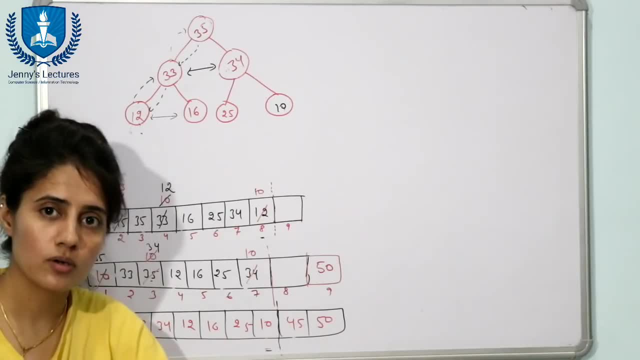 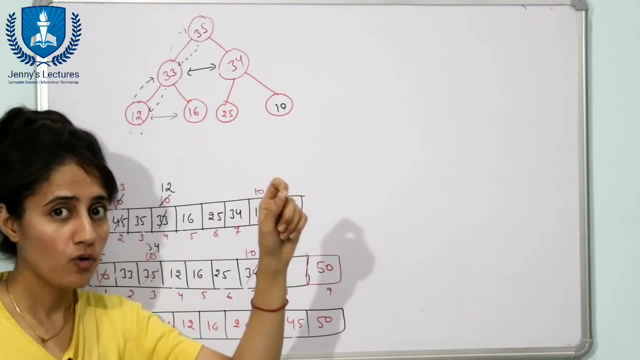 order. and if you want to sort the data in descending order, then just use min heap, because the root element in min heap is the minimum element and obviously deletion would be from the root element. so that is why first element would be deleted, the root element. so root. 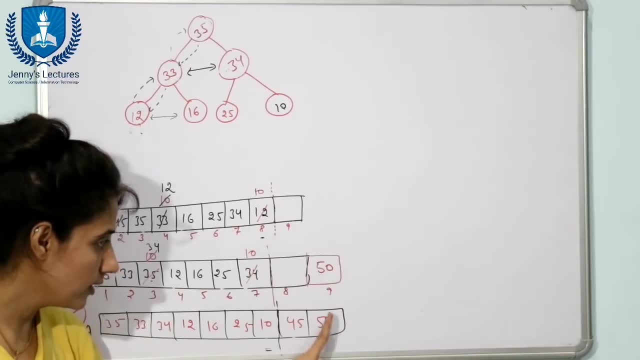 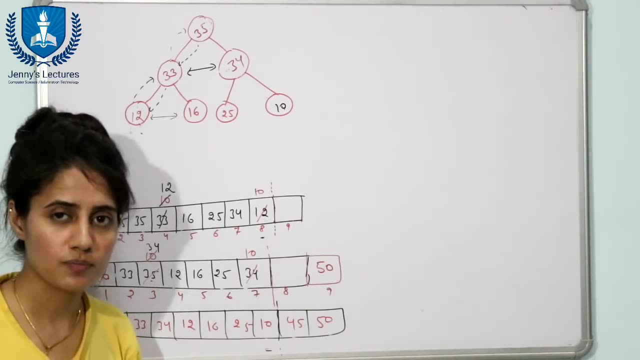 element would be here, only so the minimum element element would be here. only then the next minimum And the largest element would be at here. only so data would be at that time in descending order. so this is the idea of heap sort. In next video I am going to discuss with you heap sort. we are going to take one array. we